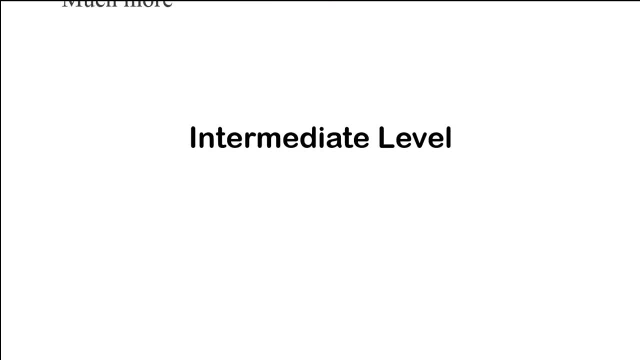 And then I will jump to the intermediate. I will start from a very, very basic level, where I will explain what is Ngrams, what is NavBag classifiers and how to make text classification system and how to train models and model testing. 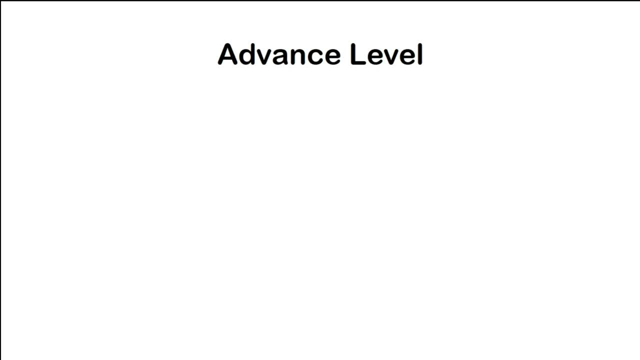 Then I will jump to the advanced level and I will explain how to check model accuracy. Then we will jump again to sentiment analysis, tokenization, parts of speech, tagging noun, phrase extraction. But this time I will explain. I will explain them so deeply and I will also explain how to detect languages and how to translate them. 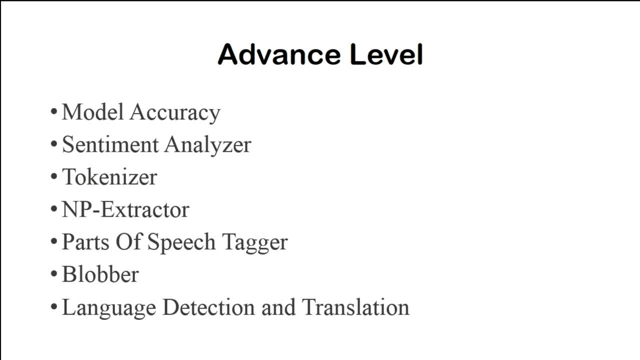 But wait now you are thinking that how this man will explain all of these things in just two hours. So don't worry. don't worry because in this course we will use the most easiest Python library for natural language processing, and that is TextBlob. 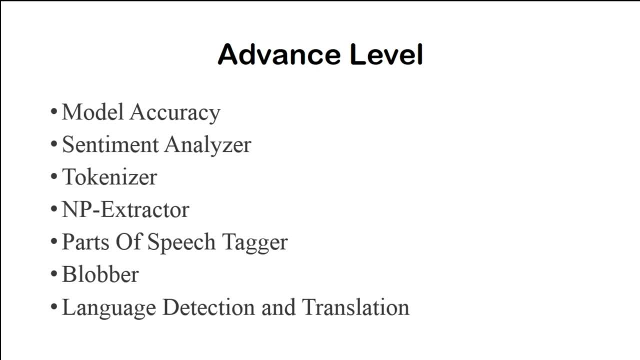 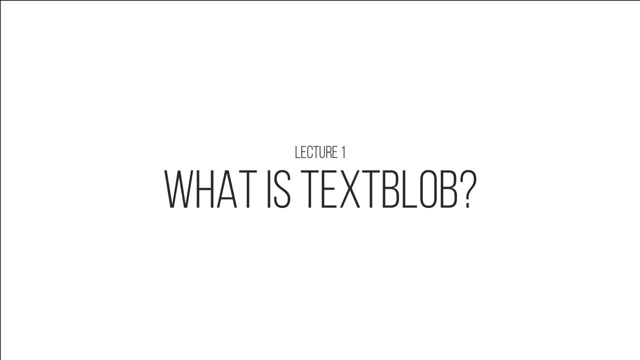 So if you are really interested, Then what are you waiting for? Just give a try to this course and I will see you in the next tutorial. So in this tutorial, we will talk about TextBlob. So let's begin the lecture. 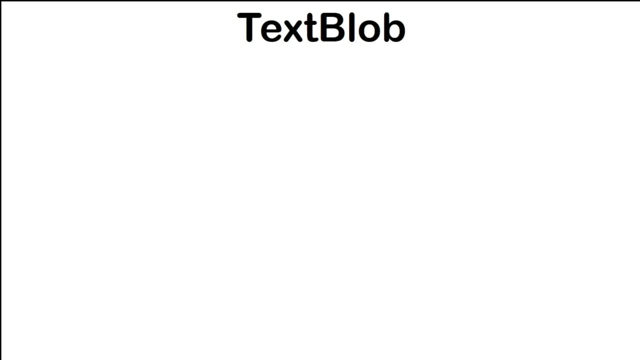 Okay, so TextBlob is basically a combination of two words: Text and Blob. I hope you know very well. Okay, so TextBlob is basically a combination of two words: Text and Blob. I hope you know very well What is Text. 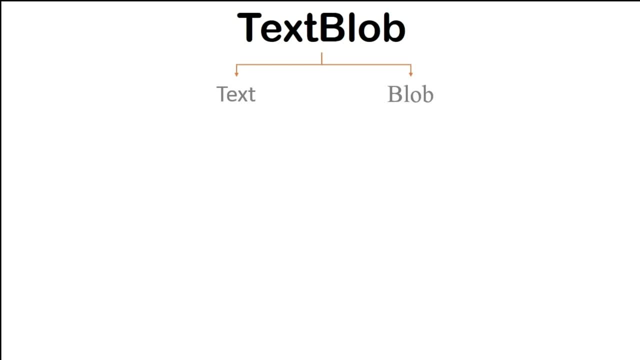 So Text could be a word, a sentence, a paragraph or even a whole essay. Okay, and what is Blob? So a Blob is basically a small spot or lump of anything. Okay, so in this case, what will be our Blob? 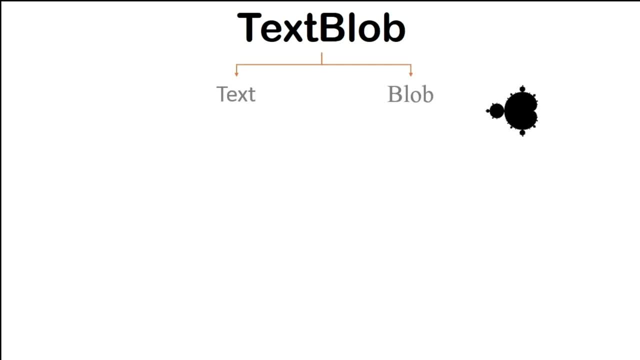 So our Blob will be a blob of text, a spot of text, Okay, so I hope this will make sense. So, by definition, So a TextBlob is a Python library for processing textual data. Okay, so keep in mind that it is a library for processing textual data. 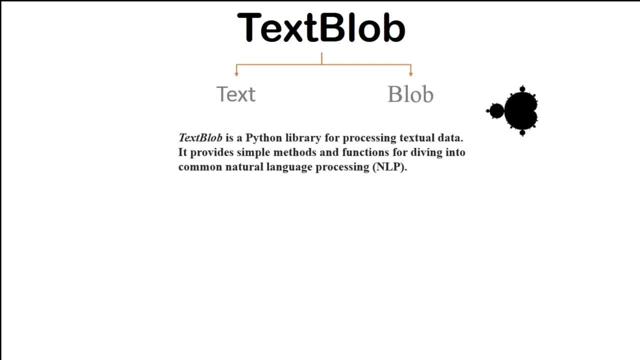 So it provides us simple methods and functions for natural language processing, Or if I say it provides us APIs, simple APIs for natural languages processing, then it will be quite good. Okay, So here I have a question, And I hope the same question will be in your mind as well. 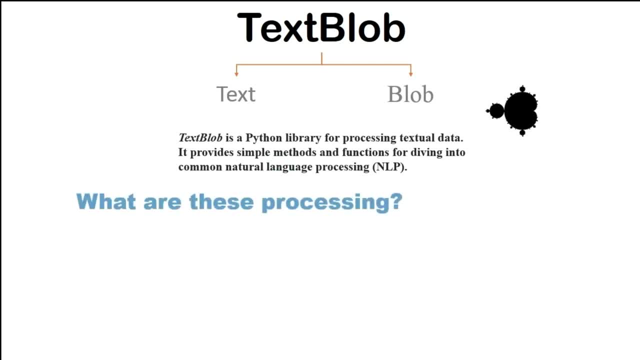 And that is what are these processing. So what are natural language processing? Okay, So these processing includes part of speech tagging, noun phrase extraction, sentiment analysis, classification, translation and much more, And we will go through all these things very deeply in the next tutorial. 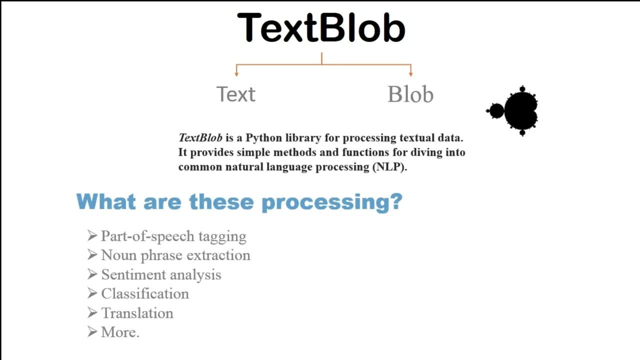 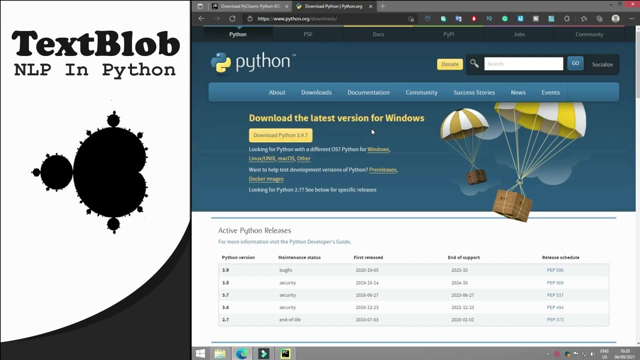 So keep watching the course and just follow the instructions. And in the next tutorial we will see how to prepare environment for TextBlob. So I will see you in the next tutorial. In this tutorial we will see how to prepare environment for natural language processing using TextBlob library. 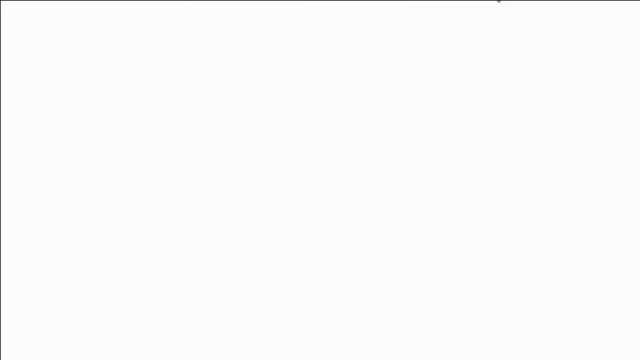 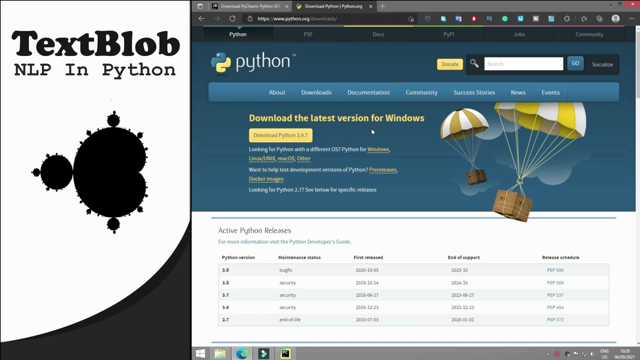 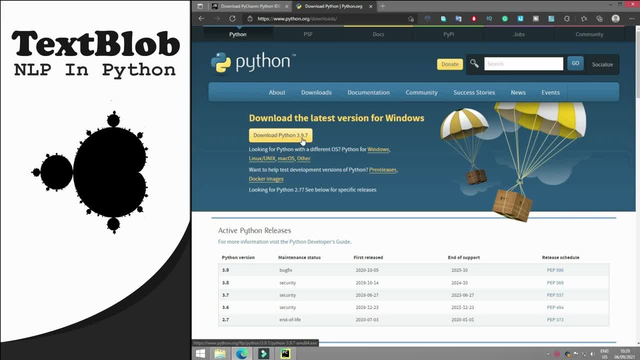 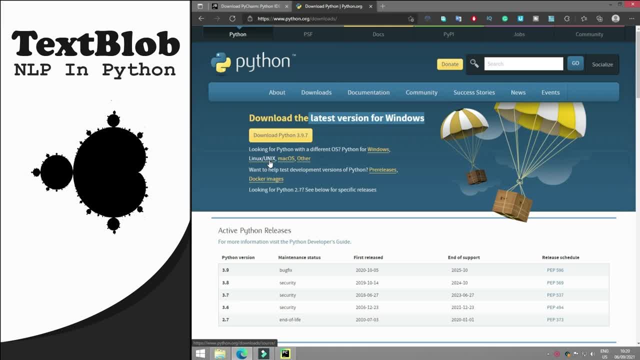 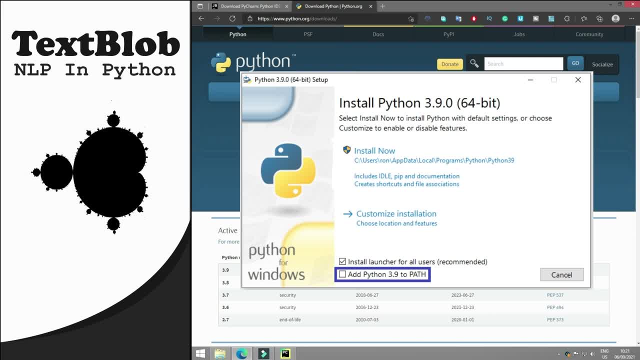 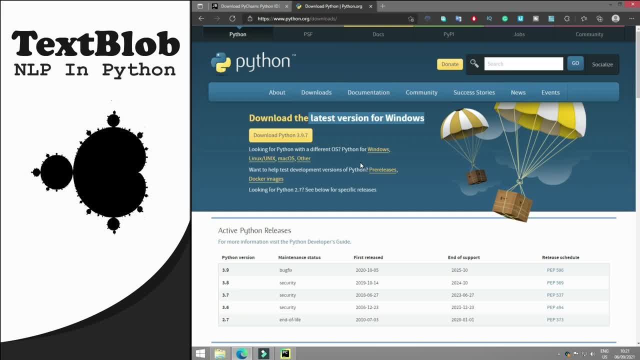 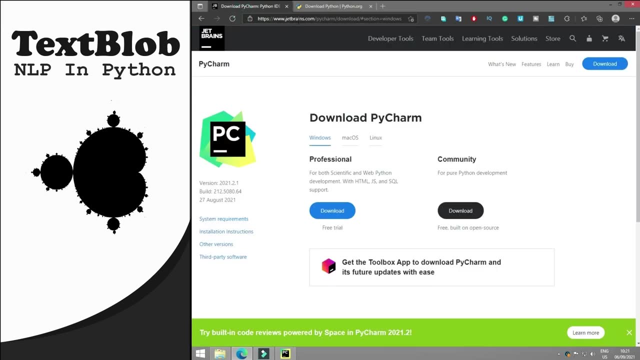 environment variable. okay, so now make sure that you do this step. this is very important, otherwise you need to add- uh- this, the path of python- manually to the environment variables. okay, so after downloading and installing python, just go to the uh jetbrandcom slash pycharm. okay, and what is? 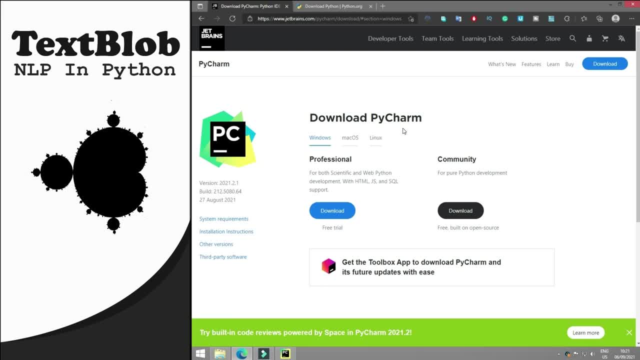 pycharm, so i hope you know very well. uh, pycharm is basically an ide, an integrate, integrated development environment, uh, in which we will actually write our code. and the reason why i'm using pycharm is that, firstly, its interface is quite good and, secondly, it is made for python. 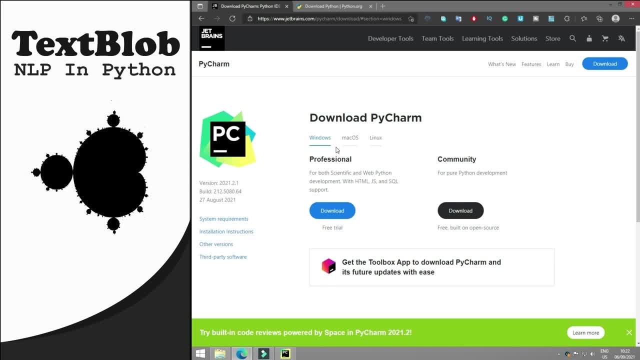 development and that's why i'm using pycharm. so there are two versions of pycharm: the professional one, okay, and the community one. so we need, uh, pure python development. so we will download community one, okay, otherwise you can. you can use pycharm professional one, but i think that we do not need it and it is paid as well. okay, so just download. 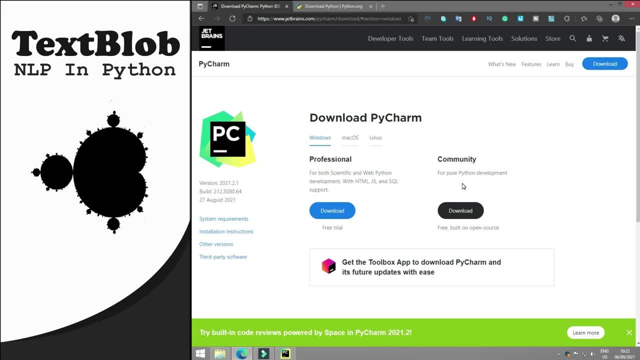 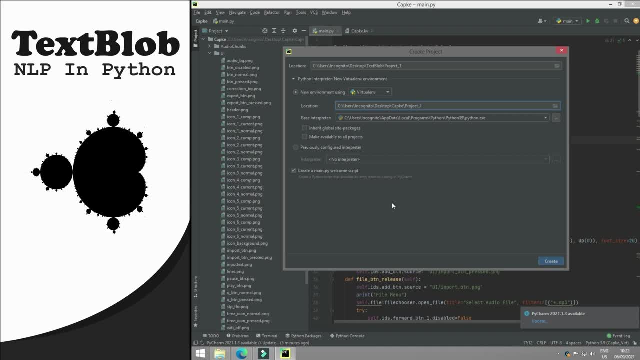 the community one and just double click on the setup, hit next, next, next and install, and this will install your pycharm. okay, so after installation of pycharm, you will get such type of interface. okay, not in the back one. okay, you will get this type of interface in which it will. 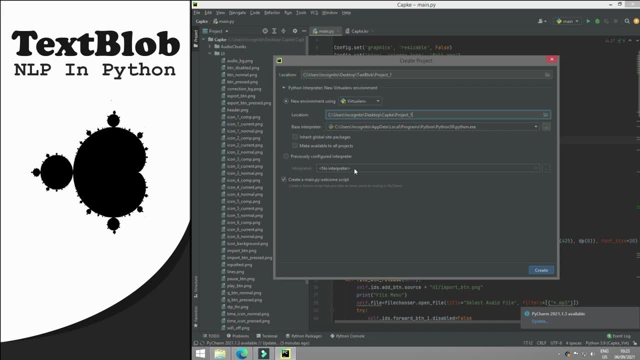 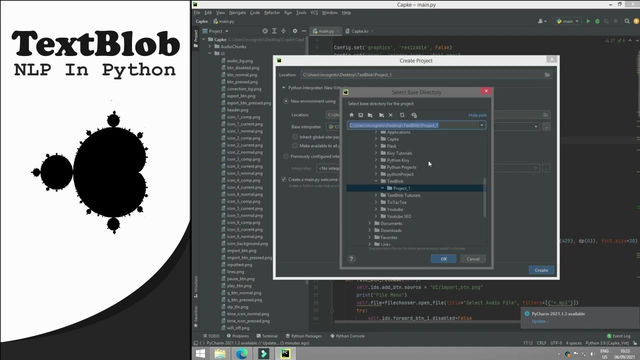 ask you location, okay, and all other things. we will go through all these things. so, first of all, location: so we need to create a new project and we need to set a location for our project. so just click on this file button, okay, and just define your location. so i want to save my project in the 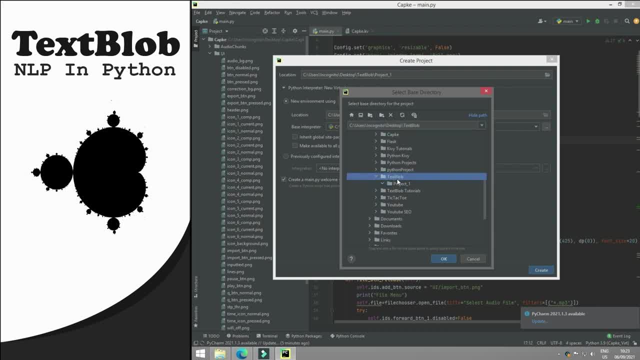 desktop and i have created a separate folder with the name text blob. so how you can create a separate folder? so just click on this button, okay, and it will create a new folder for you, okay. so after creation of new folder, i have created an other folder with the name project, underscore one, and in which i will save all my 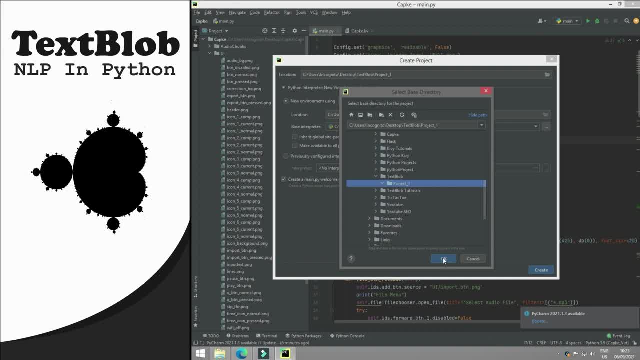 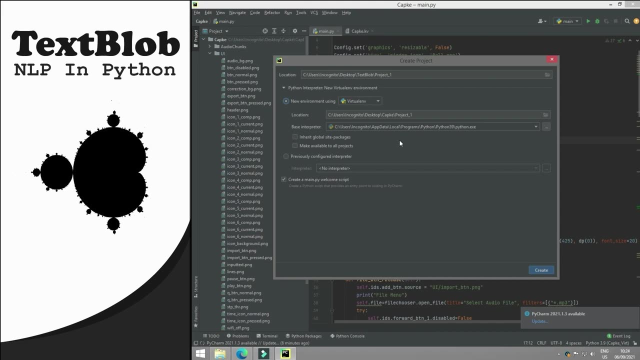 files, okay. so after creating everything, just click okay, okay, and now we need to create a virtual environment. what is virtual environment? so virtual environment is basically an environment which is a virtual environment. okay, so i hope this will make a sense. but everything we do in virtual environment do not interact with our main system, or everything we do in our main system do not. 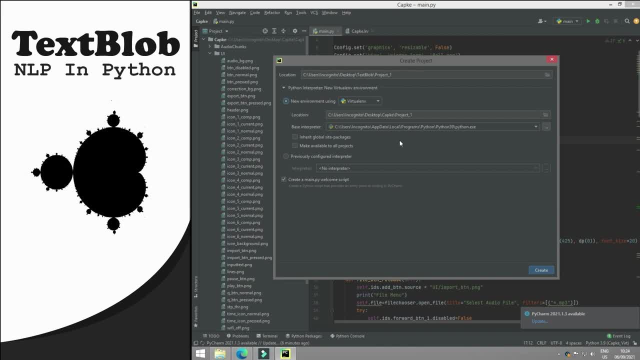 interact with our virtual environment. so this is basically a difference between a main system or a virtual environment. okay, so we need to define the location for our virtual environment as well. so just click on this folder and i will go with text blob. okay, and uh, i will create a separate uh file here. okay, a separate folder. so 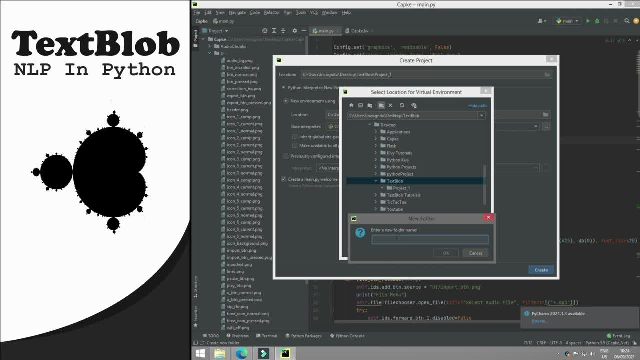 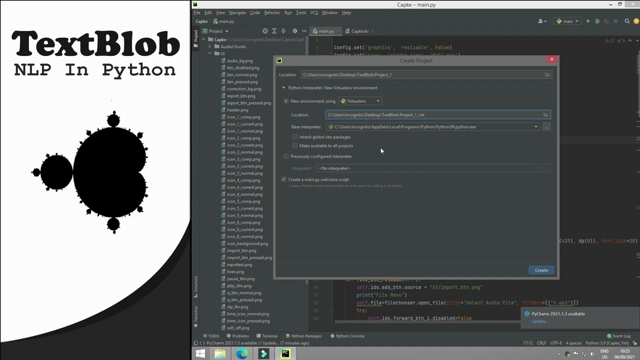 just click on this folder icon, okay, and just write like: project underscore one underscore v-i-r-t virtual- okay, and just click ok, and this will create a virtual. uh, this will create an other folder in which we will save all of our virtual data and just click okay, okay, so i hope, till this, till that point, you have understood everything. 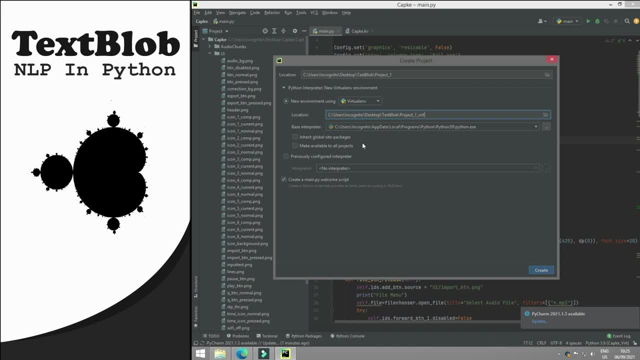 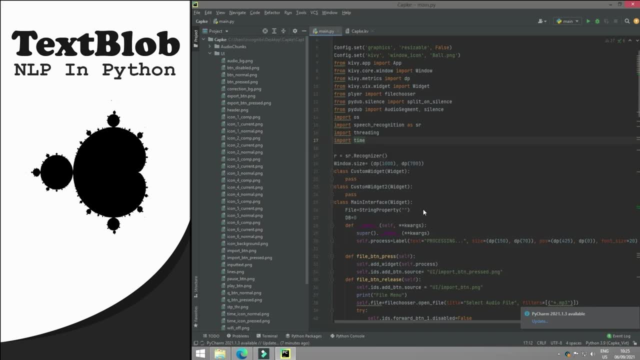 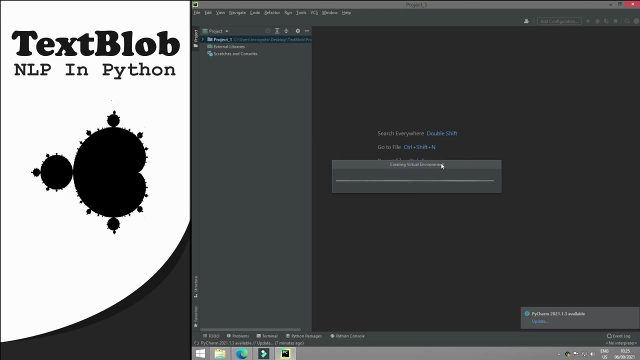 and nothing else we need to do. just keep everything as it is and just click here create, and this will on this window and this will create our virtual environment for us. okay, and it is loading components, creating virtual environment. okay, so just wait for a few seconds. so, once our virtual environment is ready, you will find such type of interface. okay. 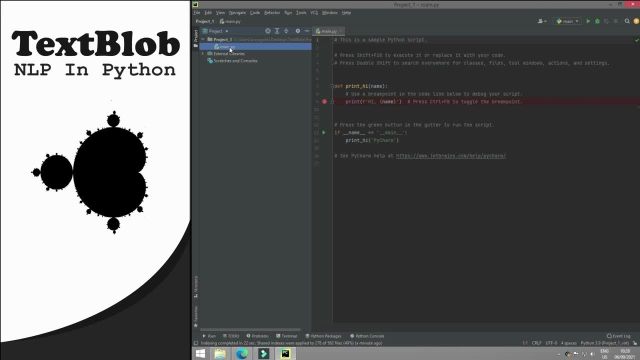 this is our project, one folder, and this is our mainpy file. don't worry about this code, just select everything and just press backspace. okay, so we do not need that code. okay, so now we have installed python, we have installed pyjama. okay, and now third step, and that is to install. 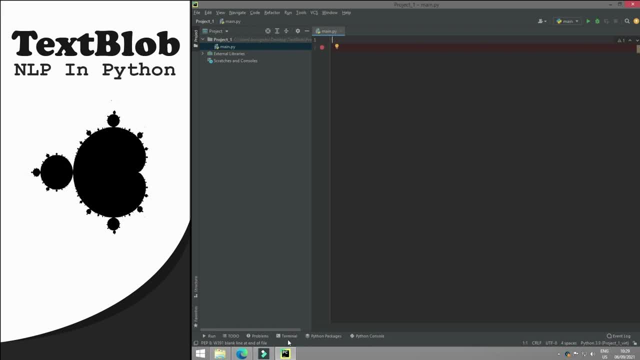 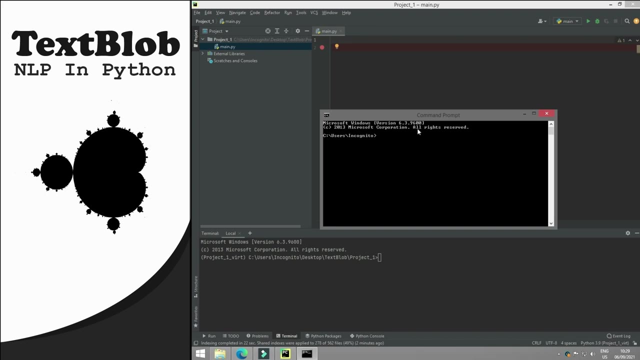 olympics, our text blob. okay. so it's very simple, just open the terminal. okay. so if i install my text blob using cmd, okay, just type here cmd. and if i install my text blob using cmd, then the program which we will write in inside our pycharm will not run and it will give us an error. and this is because we 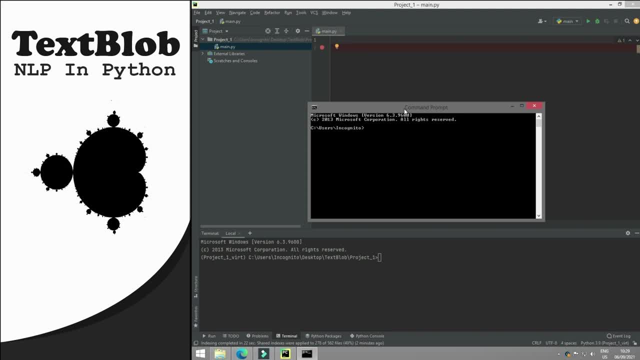 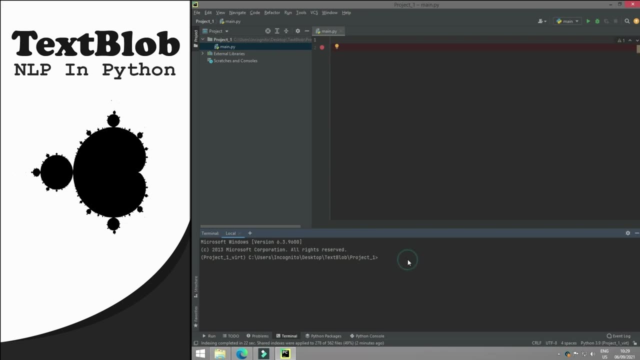 have created a virtual environment, so there would be no interaction between our system and our virtual environment. okay, so do not install text blob using cmd. okay, try to install it using the terminal of pycharm. okay, so just write here pip and install, and just write here text. be a lobby. 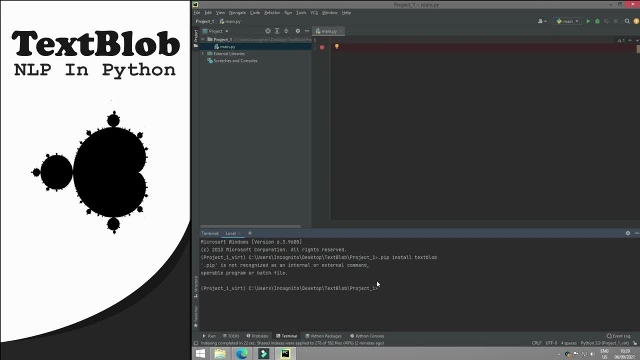 text blob and just hit enter. okay, pip is not recognized, sorry, pip. pip install and std install text install. install text the blob, okay, and hit enter and this will start. uh, installation of text blob. okay, and this will take a few seconds. okay, so after the installation of text blob, uh, we need to actually uh the. 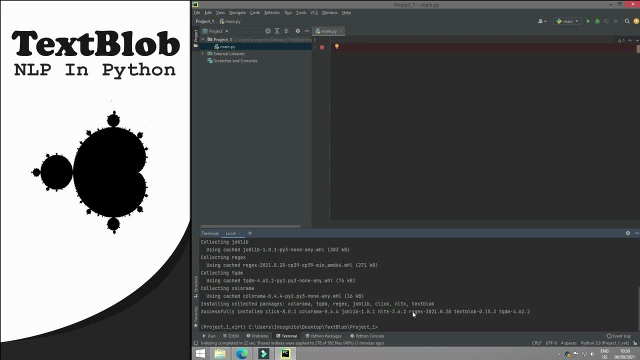 necessary nltk corpora. so let me clear you that the text blob is based on uh nltk library. okay, so we need to install the necessary corpora for uh, this text blob. okay, so just write here python. okay, and then dash m text blob dot download. download underscore corpora. okay, so we need to install the necessary corpora. 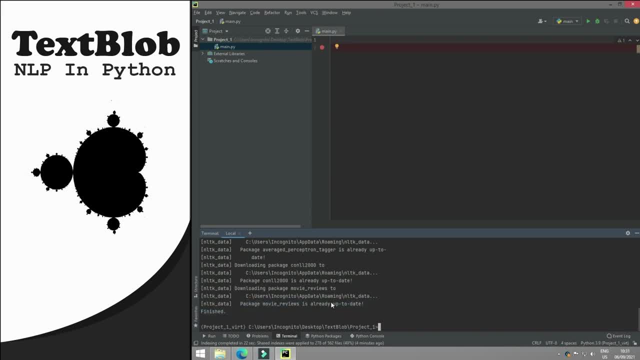 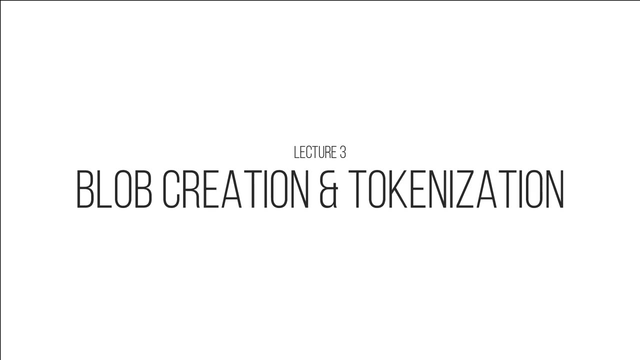 for text blob and hit enter. so now we have the necessary corpora as well. and this was all of our all about preparation of environment, and in the next tutorial we will jump into the development. so i will see you in that tutorial. so in this tutorial we will jump into practical work. 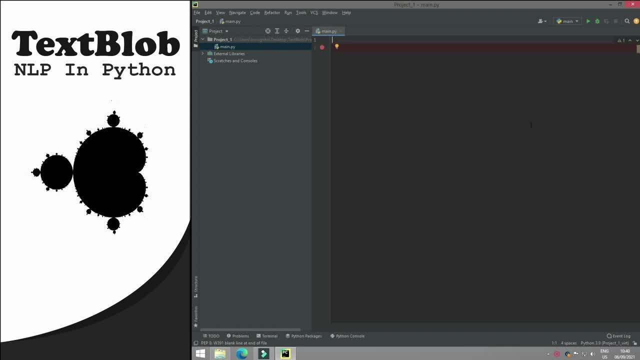 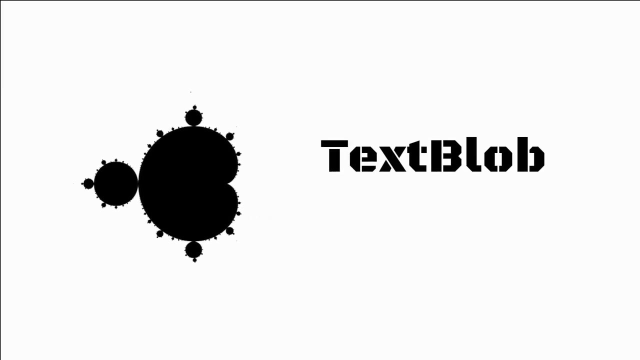 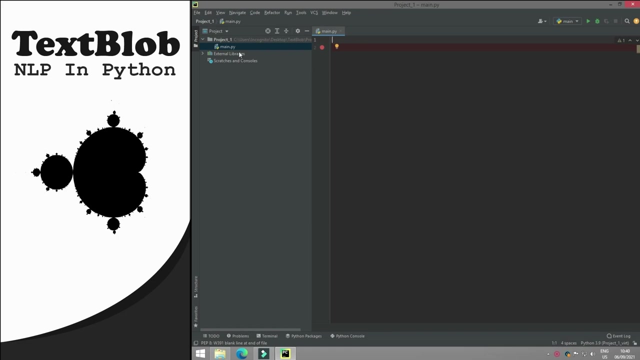 and we will see how to create blobs of text in text blob, and then we will see how to perform tokenization, which is one of the basic nlp operation. so let's begin the lecture. okay, so previously we have created our virtual environment and this is our manpy file. 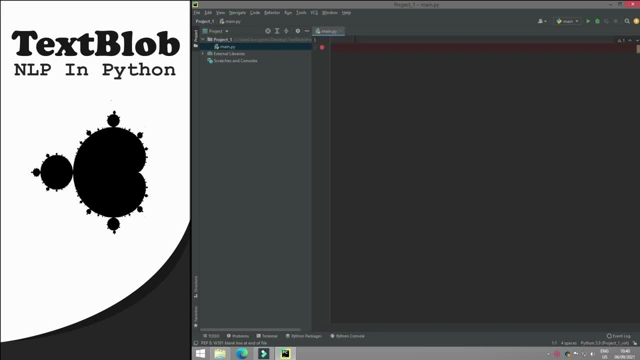 so first thing first, and that is import our text blob. so just right here: from text blob, import, import, import text blob. okay, so we have imported our text blob and we have created our text blob and we have created our text blob, imported our, this text blob and, with the help of this class, we will actually create our. 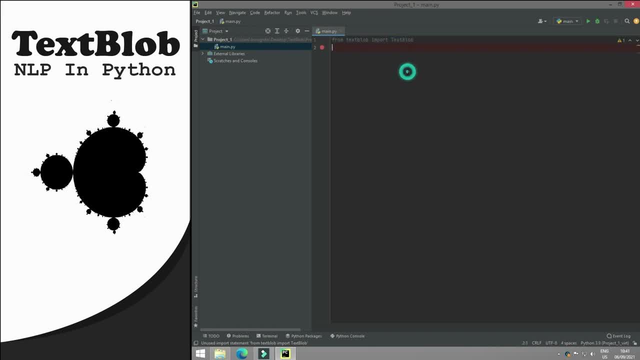 blob of text. okay. so let me clear you that performing anything in text blob consists of two steps, okay. so in the first step, we create a blob of text, okay, and in the second step, we call a certain function for a specific task. okay, so i hope this will make a sense. so now let's come to. 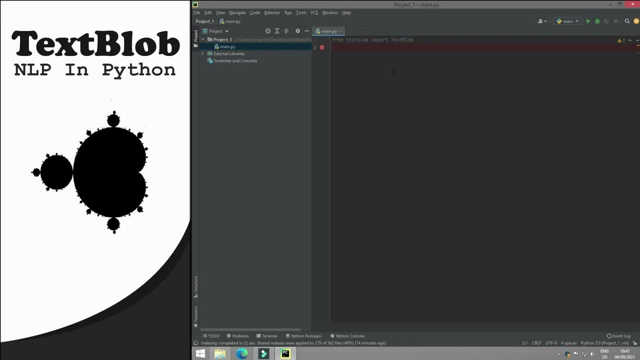 step number one, and that is creating a blob of text. so, just right here, vlob blob is equals to, and text brackets. okay, and now inside this text blob, just pass our required string, okay. so, for example, in this case, i will go with like: hello, hello, uh, this is natural. l-a-n-g-u-a-g-e- natural. 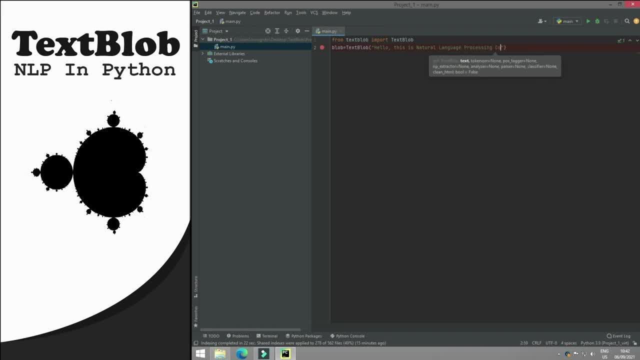 processing course. okay, so this is natural language processing course and awesome, we have created our blob. and if i type here print b-l-o-b blob, it will print our blob. okay, so if i run it. okay, so this is our string. okay, so awesome, you have completed step number one and that. 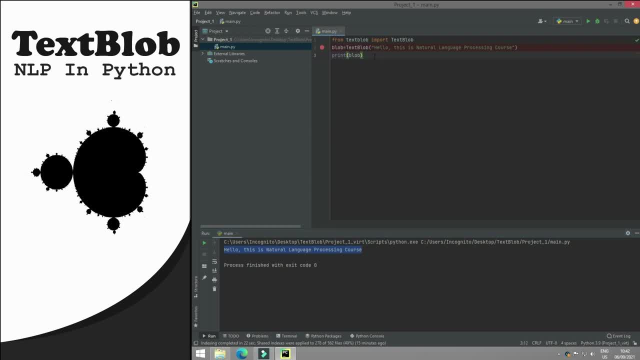 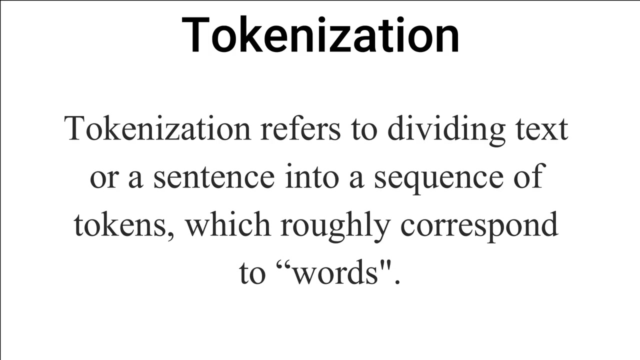 is creation of a blob. and now we will jump to step number two, and that is calling a function for a specific task, and in this case our specific task is tokenization. so before i jump into tokenization, you need to understand what is tokenization. so tokenization basically refers to dividing text or a sentence into a sequence of tokens, and 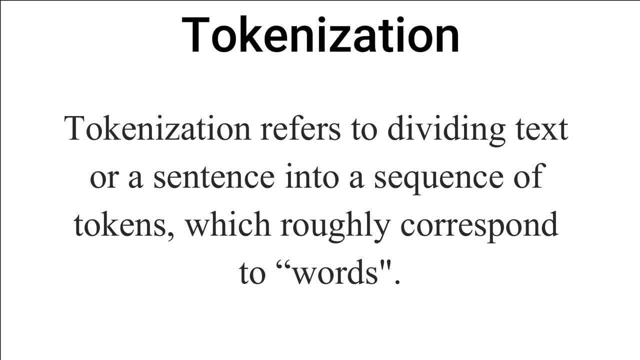 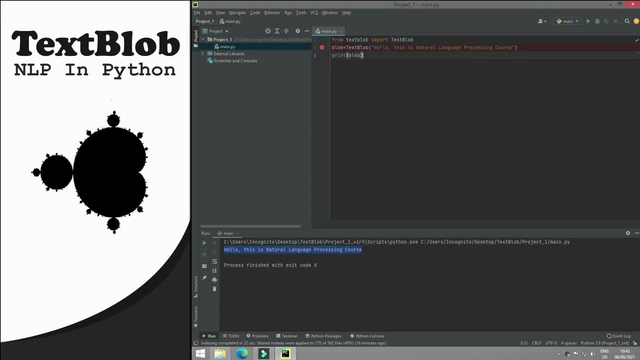 these tokens roughly corresponds to words. okay, so in a simple definition, we need to divide this sentence into words. okay, and it's very, very easy task, okay, so just call blob- okay, our variable blob, and just put dot and then just write here words. okay, we need to divide that. 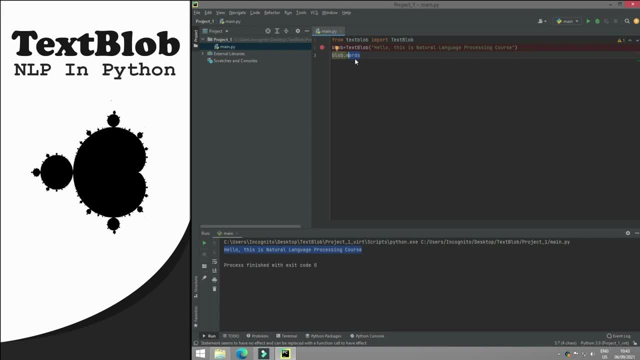 sentence into small tokens or small words. okay, and if i run it, we will get a little bit of work for this deal. so just go back to aseguor, which we run. the thing we are going to do here, that isthis little binary of the text and this is our. 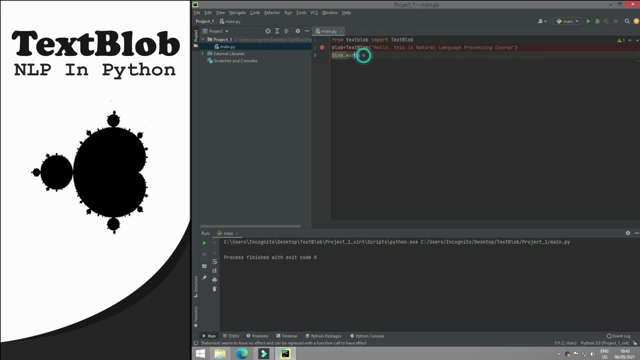 класс and you can see that its exactly what it's called. so we will leave this one as longer. once again, okay, it's 3, three, four, five, six, seven, eight. okay, we are going to write printnow here. then it will appear in detail in real time. if you close it, then you will see that at the end when it goes up the rest of theiting time. then you know this function has been created token, but we know lots of things in the library and we need to print it. so this is our, this is a natural language processing course. now let's click here to print everything from here. and if we�� car of war on the Bunny. 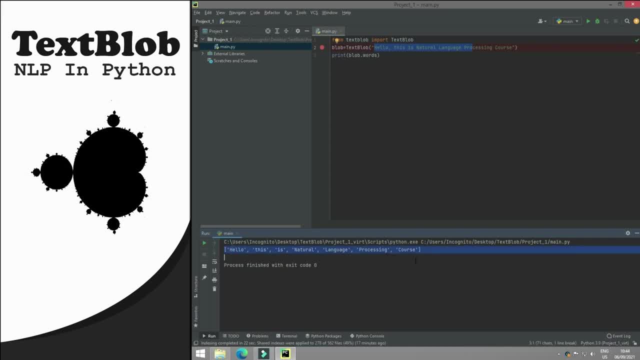 course. okay, so this is basically a list. okay, and uh, you can actually loop through all these words as well, okay? so, for example, if i write here for uh b in b l o b, blob, dot, w o r d s words, okay, and i need to print each word separately and in this case this will be my b, and if i run it, 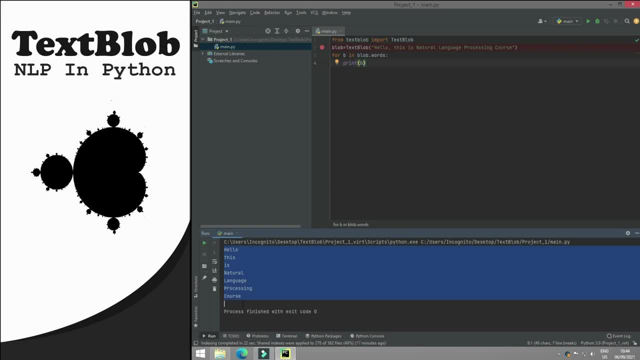 yeah, here is my hello. this is natural processing class, so this is how you can actually perform tokenization in text blob with just a single letter. so that's why i choose text blob library for natural language processing: because it's very, very cool, it's very easy and it's very awesome. 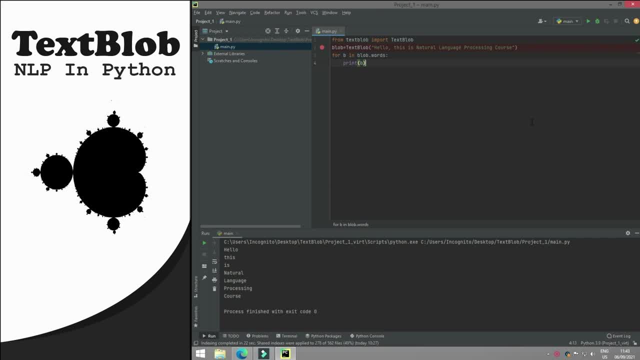 in this tutorial we will see how to find different type of part of speech in a sentence. if i say we will do part of speech in a sentence, if i say we will do part of speech in a sentence, if i say we will do part of speech tagging in this tutorial, then it will make more sense. so let's begin the lecture. 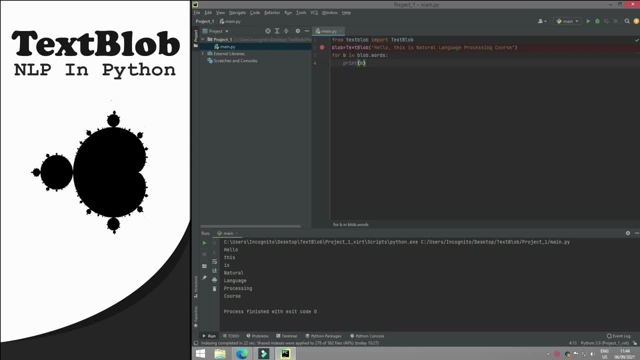 okay. so, uh, previously we have done till this point, we have done tokenization here, okay, and i hope uh you have understood it, and now we will do part of speech tagging. so it's very simple. uh, just keep in mind that, uh, performing any type of task, 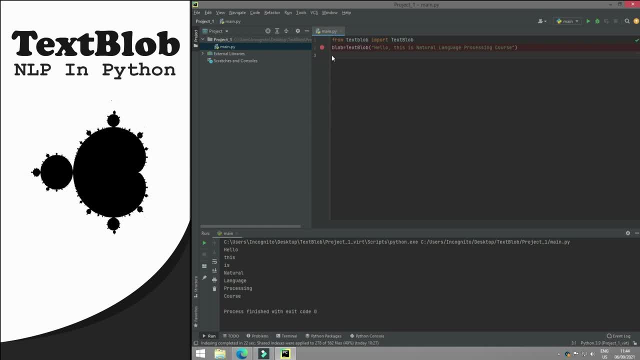 in text. blob consists of two steps: creation of a blob and then performing a certain operation on that blob. okay, so this is our step number one and this is our blob. so this is hello. this is a natural language processing course. okay, so this is my blog and now i will apply uh tagging. 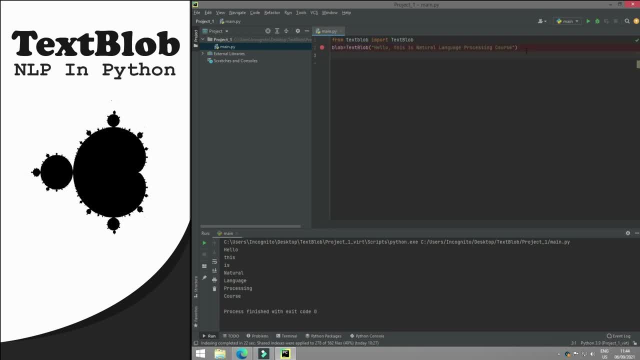 part of speech: tagging on this blob. so it's very, very simple: if i say blob dot t-a-g-s text okay, and if i say all of these tags in a variable, like i will say that part of speech, okay, pos part of speech, and i will say i will save every tag in this part of speech variable and then i will print. 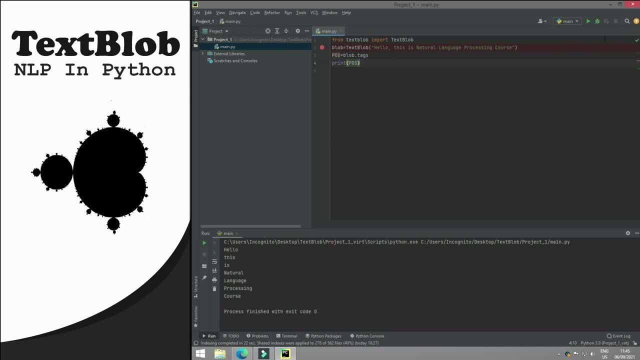 that variable. okay, pos, and if i run it, hope this thing will work fine, okay. so, yeah, here is my output, okay, so here the hello is my noun. okay, and this is my dt. so these are all the abbreviation of a different part of speech. okay, i have given a list. you can just download that list and go. 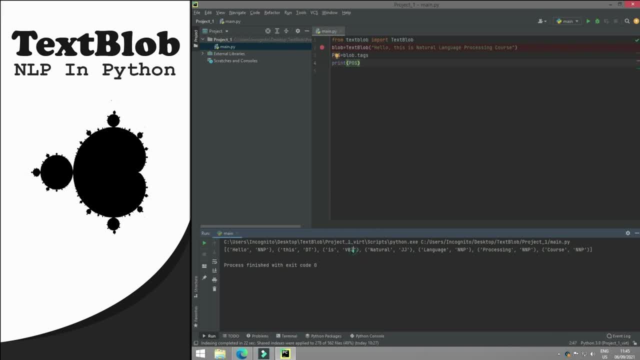 through all these abbreviations. okay, so wbz represent verb. okay, natural jj and language noun- again okay. so this is how you can perform tagging in text blog. okay, so now what i want? i want to print only nouns. okay, so it's very simple. i will loop through. 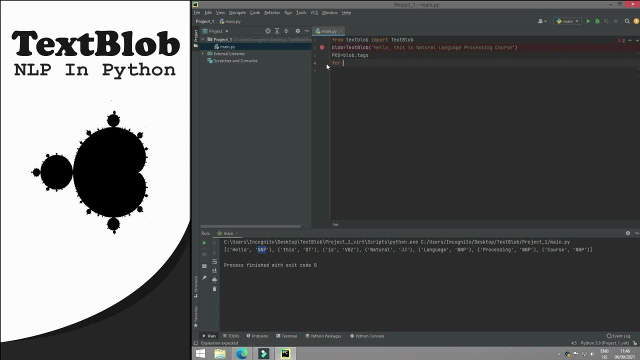 the list okay, for, uh, i will say the name of the world or i will say world okay, and i will say tag in pos, okay. so why i'm writing here world and tag? because this pos returns two tags: one is the word okay and the other is the tag okay. and that's why i'm writing here word and 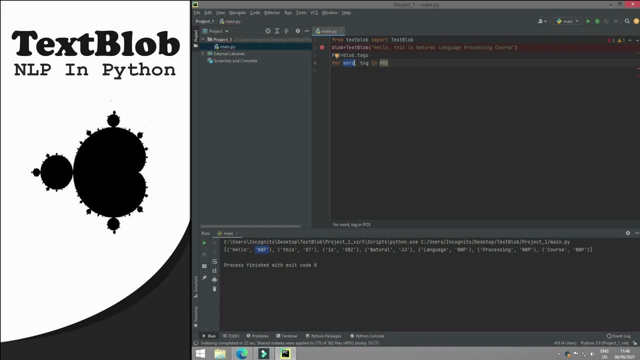 comma tag. okay, i will say word in this variable and i will say it's tag in this variable. okay, so it's good. and now i will check if, if my tag double equals to my tag double equals to like an n and p, noun, okay, then i will just need to type: my tag double equals to my tag double. 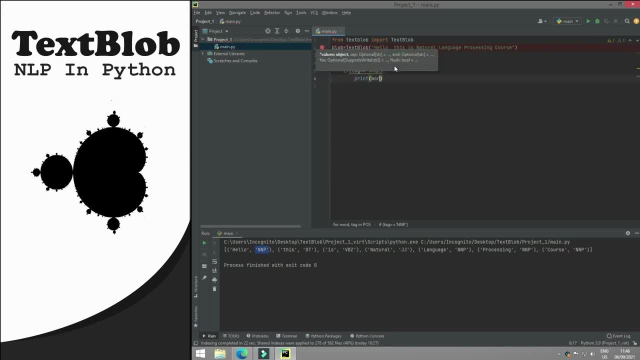 to print that world, okay, w o r d word- okay, so this will print just noun, okay, and if i run it- and yeah, here are my nouns, okay, hello, language processing course. okay, so i hope you have understood. we will see how we can perform noun phrase extraction in text blob. so let's begin the 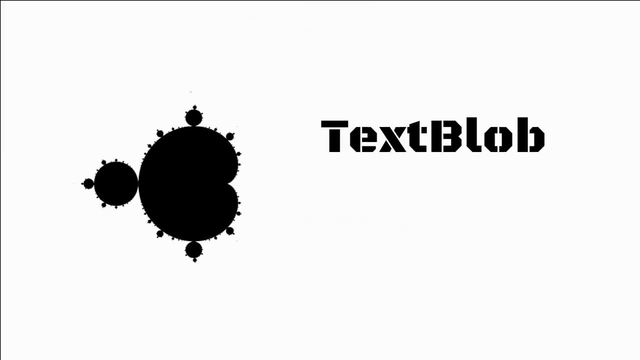 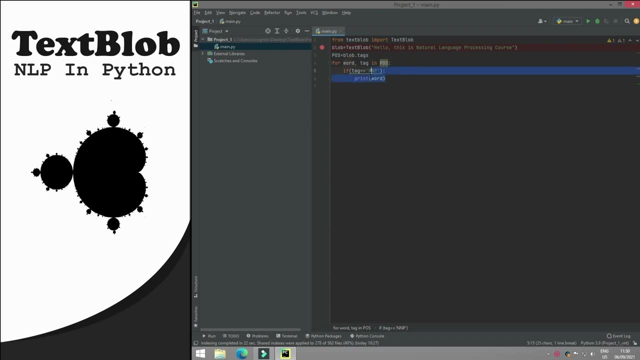 lecture letter tat uh, previously, uh, we have done till that point where we were performing some uh spot of speech tagging processes in text blog, and in this tutorial we will see how we can extract noun phrases, okay. so, uh, but before i go to noun phrase extraction, let's change our text here, okay, or let's increase it, okay. so hello the. 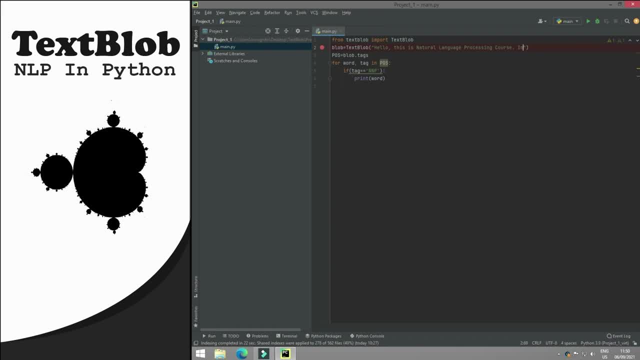 this is natural language processing course. in this course- see all you are course- you will learn text blob from beeg i double n. from beginning, you will learn some basic concepts. okay, so i think it's quite good. and now we will apply noun phrase extraction. okay, so we have our 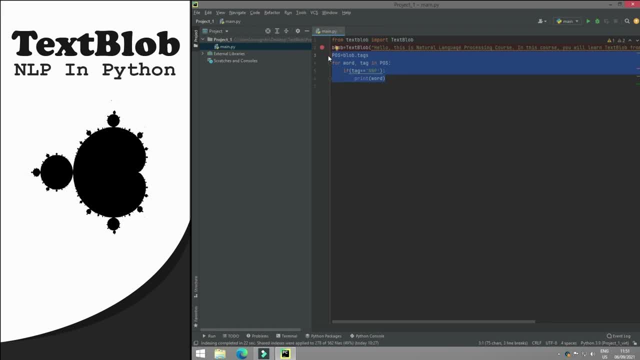 book blob okay, and now we will perform our noun phrase extraction operation here. and it's very, very simple: just try to be a lobby blob dot noun phrases okay, and we need to print it. so you can write here: p-r-i-n-t. print okay and noun phrase says okay, or you can assign: 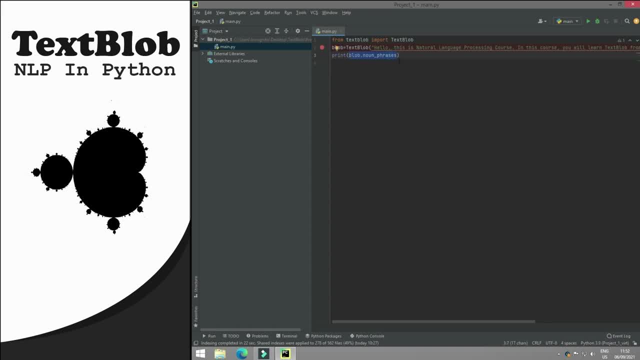 a separate variables to this blob dot noun phrases and then you can print that variable as well. okay, so, if i run it? okay, so, yeah, here are my one, two, three and four noun phrases. okay, hello, language processing text- blob basic concepts. okay, so this is quite good, you can even 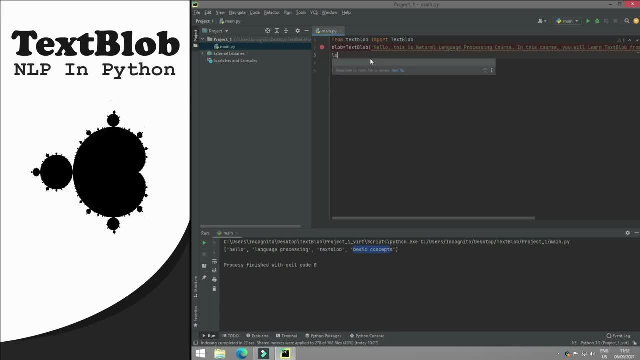 find the length as well okay so if i write here log block dot noun phrases okay and if i say that length and i say blob dot noun phrases okay if i say that length of a sentence like an ingre �, characters addi and if i add actual letters i would say like all of these are known expressions 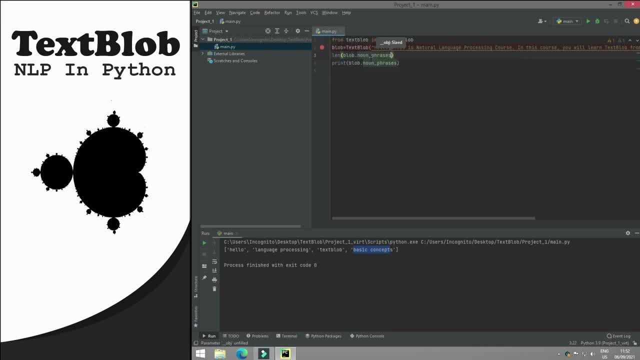 i would say like add. all of these are known expressions. then an G sweet do word sounds like dot dot noun phrases. and sixth time, i plugins are reaching a high deal. depending on the honors board, there might be an exact fit and i should 만든 an example. so, as you know, language processing tends to have specific sizes. uma iub infection. 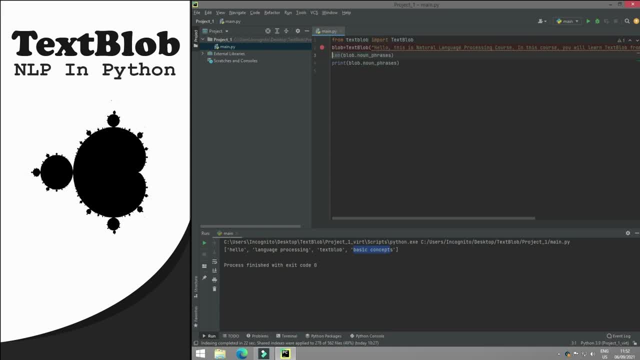 impportsикс did copy very hurry. okay, so this is quite good. you can even find the length as well. okay? so if waar say that length in a variable, like i will say, l is equals to, and then if i print l, you will find that it will return four. okay, because there are four noun phrases in this paragraph. if i run it, 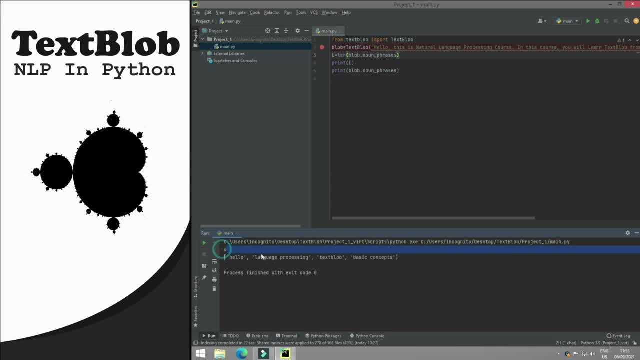 yeah, uh, here are, uh, my output, okay, and here is four, okay, so, so this paragraph contains four noun phrase, okay, so, uh, i don't know uh, how i didn't mention, but you can actually find the total number of words in this paragraph as well using a phenomena which we have done, and that is: 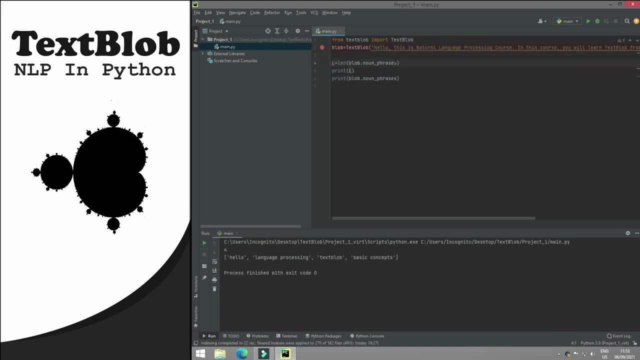 tokenization. okay, so with the help of tokenization you can find the total number of words in this paragraph as well. okay, so it's very simple. like i will say, n is equals to uh, b, l or b block dot, uh volts, w-o-r-d-s walls, and i will find the length: okay, so l-e-n, and then i will print that. 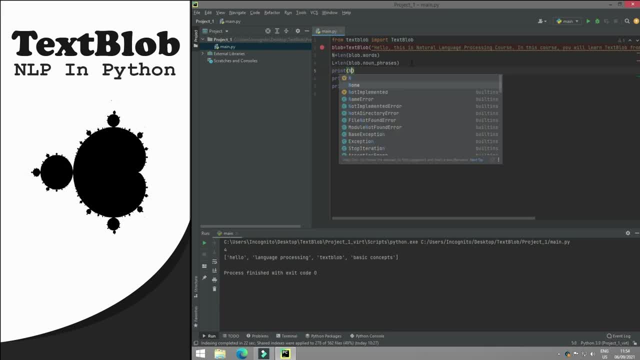 and okay, p-r-i-n-t print and and it will return the total number of words which this paragraph has. okay, and yeah, here is my output and this paragraph consists: i contain only 22 words. okay, so you can actually count it, but it's quite a time-consuming task. so this is how you. 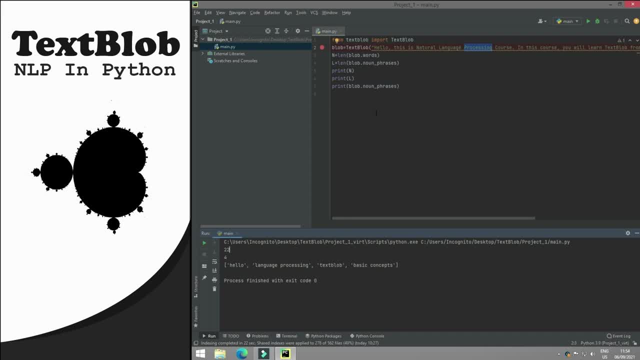 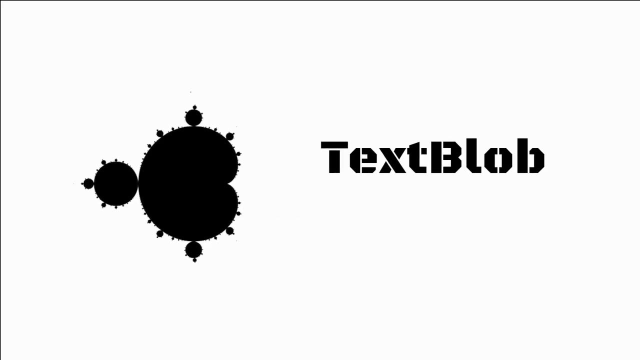 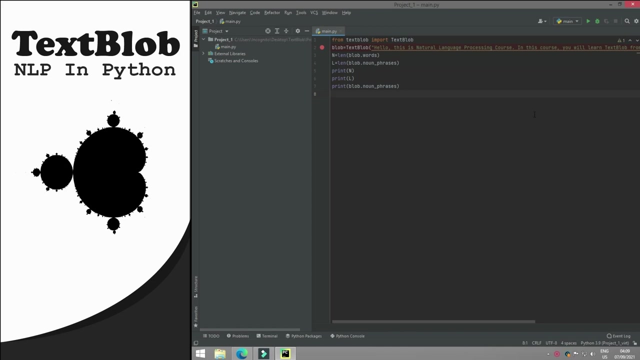 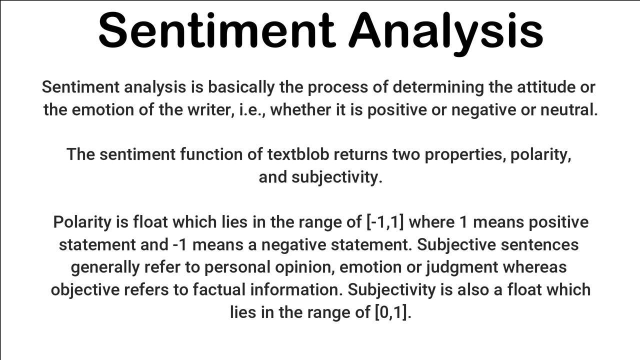 can actually count the total number of words in a paragraph. so in this tutorial we will see how to perform sentiment analysis in text blob. so let's begin the lecture, okay? so first of all, before I jump into coding, it is very important to understand what is sentiment analysis. so sentiment analysis is basically the 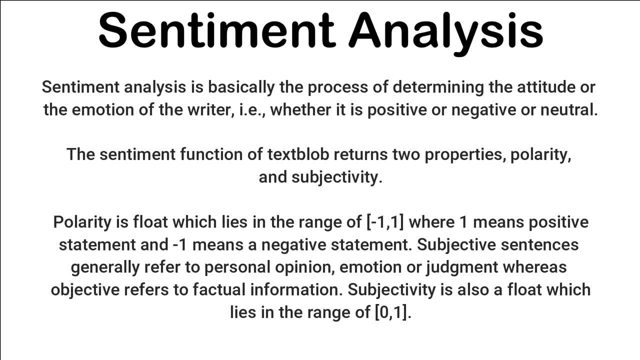 process of determining the attitude or the emotion of the writer, okay, whether it is positive or negative, or positive or neutral. so I hope you have understood what a sentiment analysis. okay, and now the sentiment functions of the text log, which basically enables us to determine the attitude or the emotion of the writer, returns two properties: the 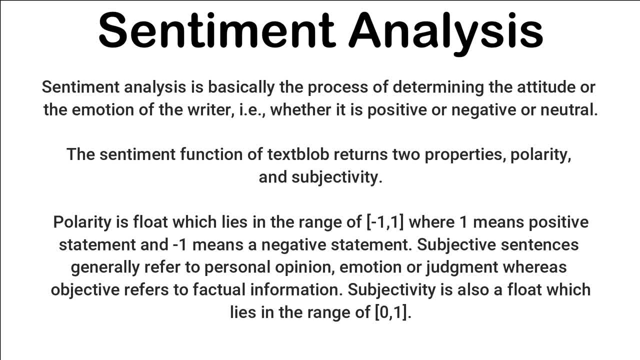 polarity and the subjectivity. so what is polarity? so polarity is a float, is a float value which lies in the range of minus one to one. okay, so if we get a polarity which value is between minus 1 to 0, then this means that the attitude 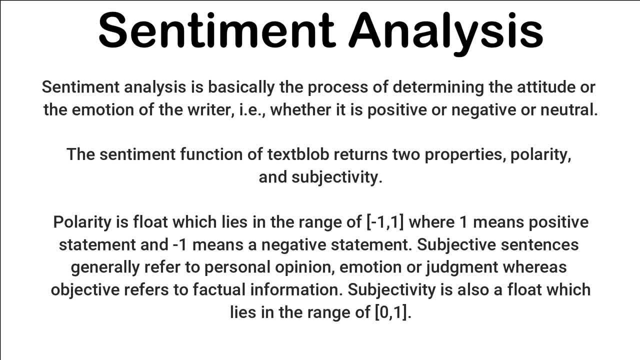 of the writer is negative. ok, if you get minus one value, this means that this sentence is very negative. or if we get a value between 0 & 1, then this means that attitude of the writer is positive. ok, so polarity basically tells us about the attitude of the writer and subjective. 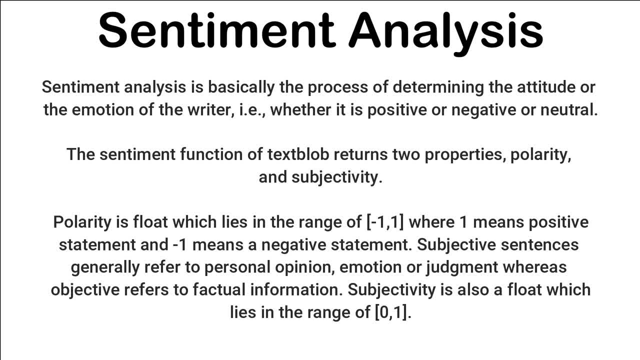 Sentences generally refers to personal opinion, emotion or judgment, whereas objective refers to factual information. okay, And subjectivity is also a float value which lies in the range of 0 and 1, okay, So polarity lies in the range of minus 1 and 1, okay. 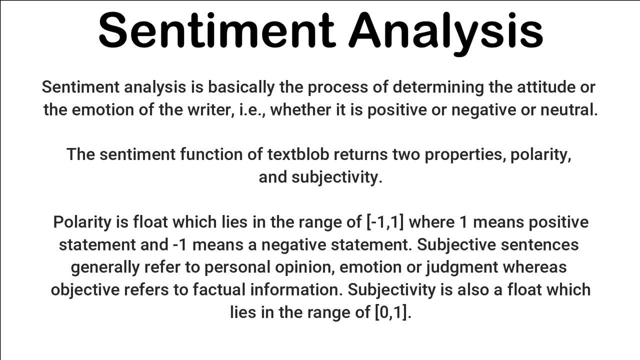 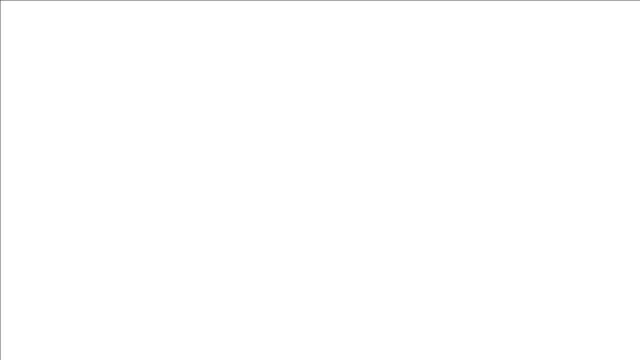 While subjectivity lies in the range 0 and 1.. So I hope you have understood what is sentiment analysis, and now let's jump into some practical work. So I am on my PyCharm. okay, Now we will do sentiment analysis, okay. 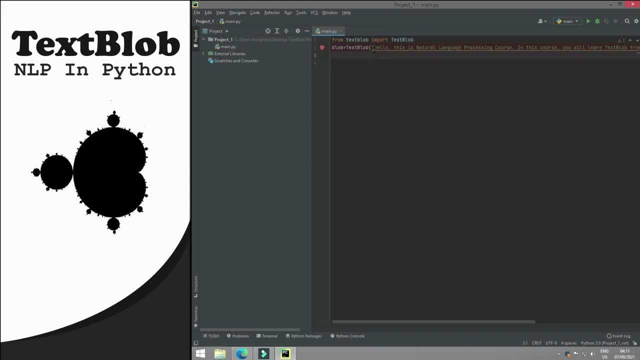 So just remove everything here and now. let's change this text, okay. So just change it and I will go with: like, YouTube is one of the best Platform P-L-A-T-F-O-R-M to learn new skills, okay. 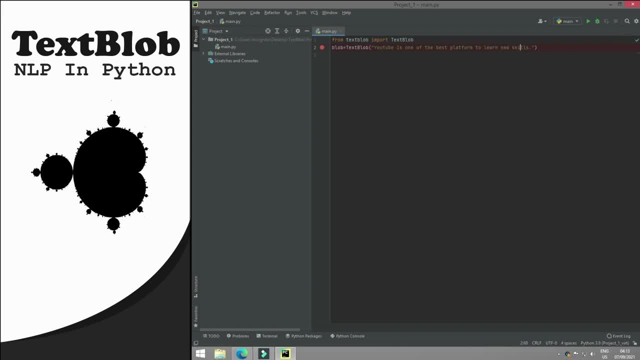 So I hope this sentence is good, okay. So now we will analyze this sentence. okay, So it's very, very cool, very, very easy. Just write blob, okay, Dot sentiment. S-E-N-T-I sentiment- okay. 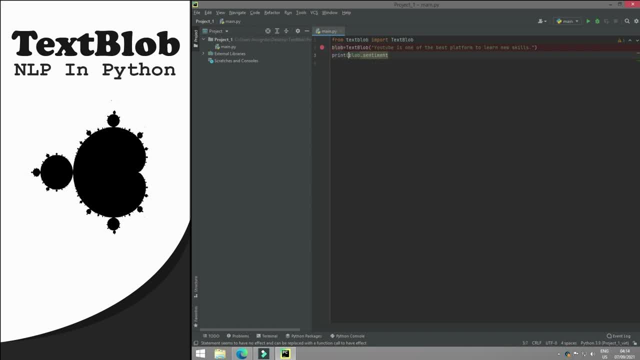 And I want to print it. So just write print and then blobsentiment and let's run it. And yeah, here is my output. That is polarity 0.5.. This means that it is quite positive And subjectivity is 0.3.. 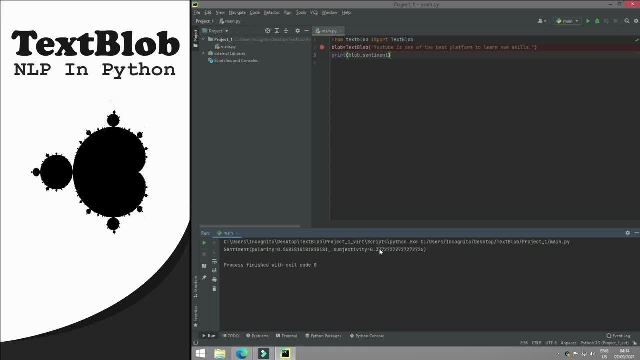 This means that it is a public opinion. okay, 30% Of public agree with this sentence. okay, So this is quite good. And now I want to print these values in a percentage. okay, So it's very, very easy. 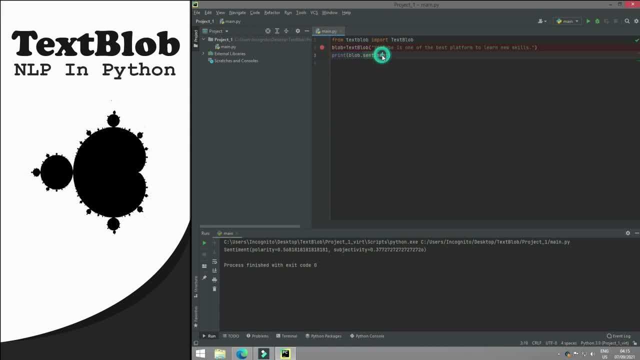 So basically, this sentiment blobsentiment function returns two things: the polarity and the subjectivity. okay, So I will save the polarity in P and the subjectivity in S is equals to blob Blobsentiment S-E-N-T-I-M-E-N-T. okay. 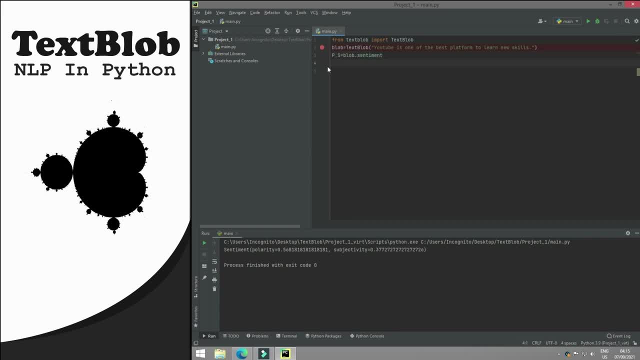 Blobsentiment. And now I will convert this P to percentage. okay, And I will call it like P underscore percent. okay, P-P-R-T-percent, okay, And now how I can convert this to percentage. So it's very awesome and it's very simple. 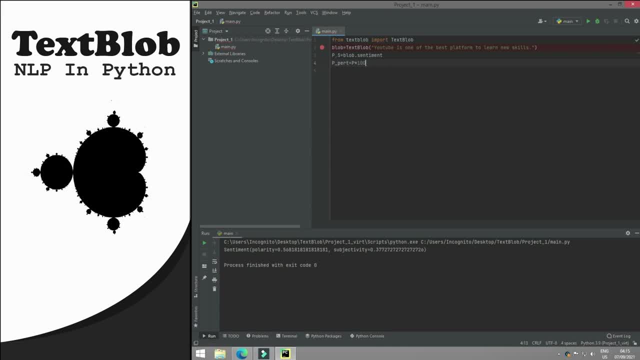 Just multiply that value with 100, okay, And then we need to Convert it into int. okay. So just convert it into int and this will return us a percentage value. And for the subject, just write: P-R-T-percent is equals to I-N-T. 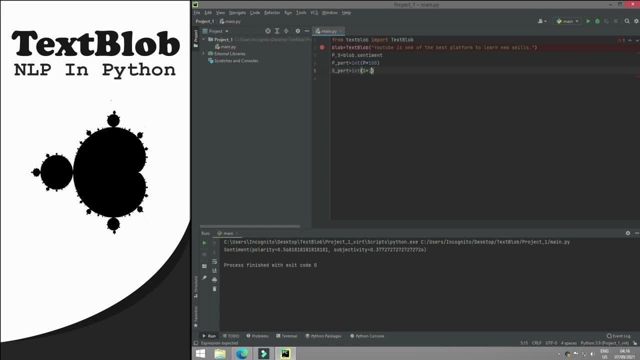 And then S multiply by 100.. And now I need to print these two values. So just write print And I will say P-O-L-A-R-I-T-Y- polarity, And for the polarity I will go with this value, which is P-percent. 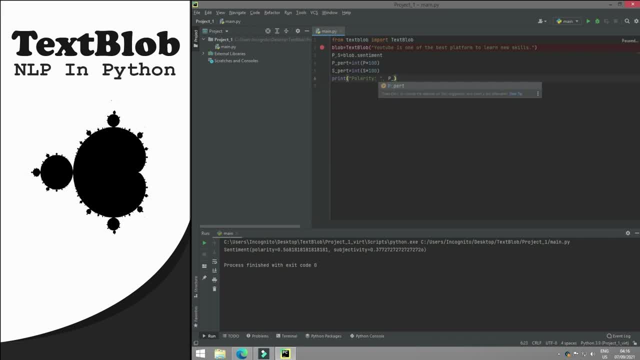 So just write here: P, underscore, P-R-T. okay, And I need to put percent sign as well here And now I need to print the subjectivity, So just write here: S-U-B-J-E-C-T-I-V-I-T-Y- subjectivity- okay. 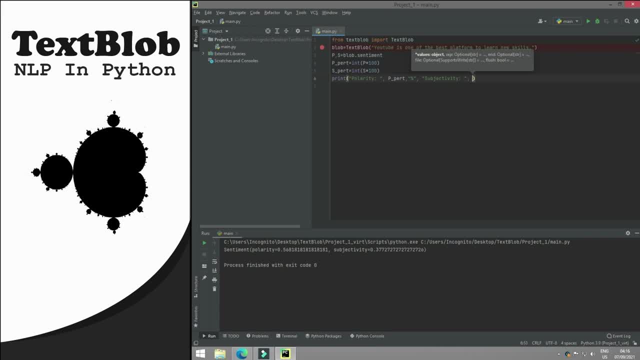 Okay, And for this the value of my subjectivity is S underscore P-R-T. okay, And I need to print the percent sign here as well. And now, if I run it, you will see everything in percentage. Yeah, my polarity is 56%, while my subjectivity is 37%. 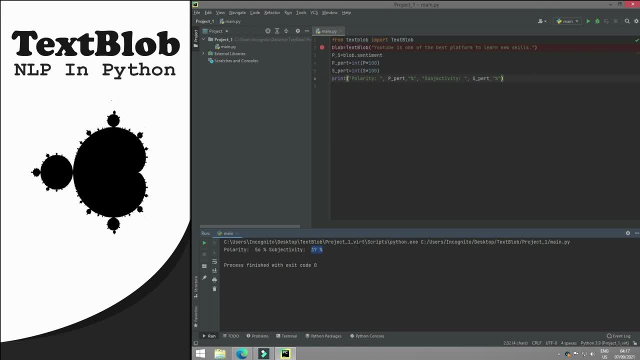 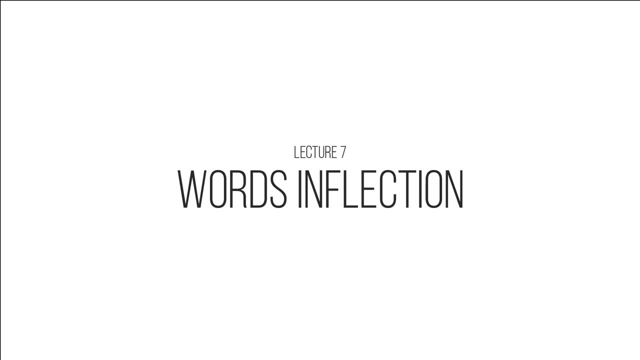 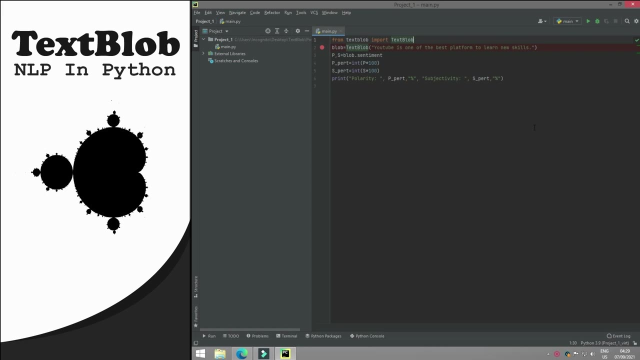 So this is how you can actually perform sentiment analysis in TextBlob. So I hope you have enjoyed this tutorial. In this tutorial, we will see what is world's inflection and how to perform world's inflection in TextBlob. So let's begin the lecture. 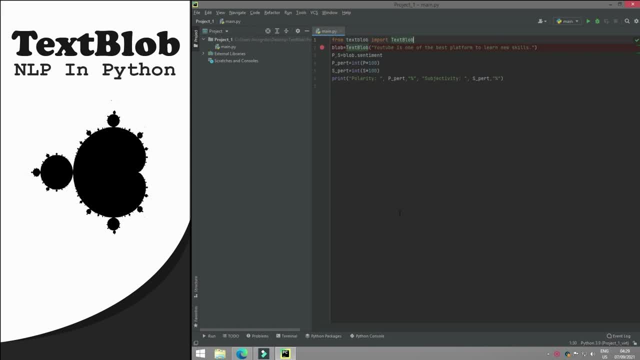 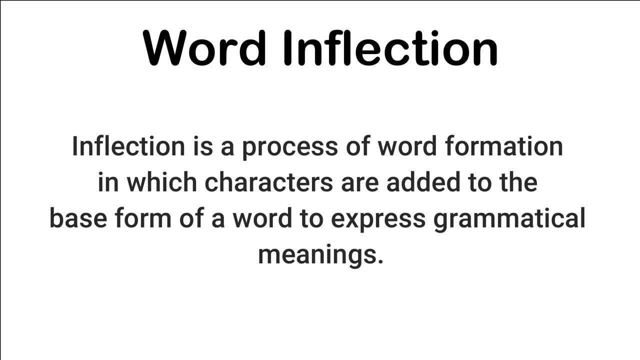 First of all, you need to understand what is world's inflection. So world's inflection is a process of world formation. okay, So keep in mind that inflection- inflection is a process of world formation, in which characters are added to the base form of world. 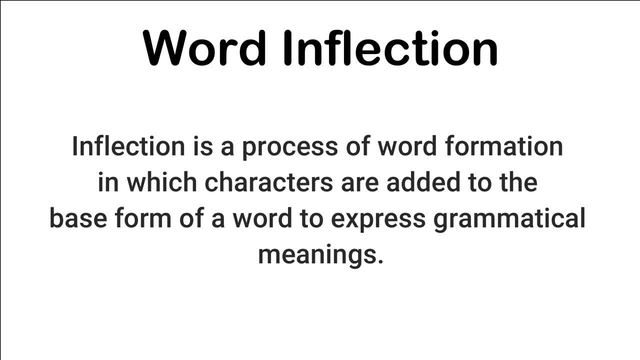 to express grammatical meanings, okay, For example. for example, I have a word, It is in its singular form. okay, And I want to convert it into its plural form. So this is called world's inflection. Or if I have in plural form. 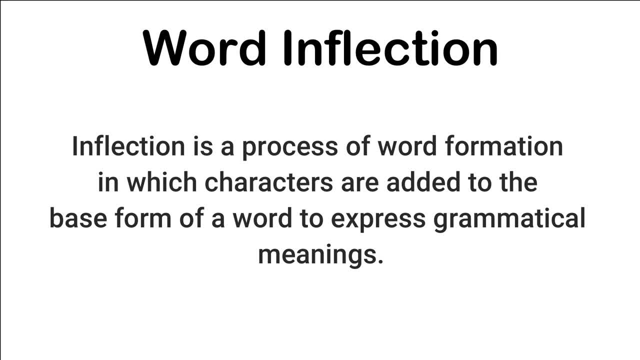 and I want to convert that world into its singular form. this is also. This is also called world's inflection. okay, So I hope you have understood what is world's inflection. So now let's do some practical work. Okay, so I am on my PyCharm. 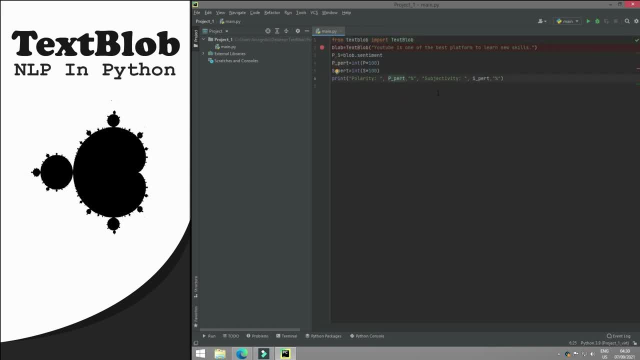 and previously we have done how to perform sentiment analysis in TextBlob, And now we will see how to perform world's inflection in TextBlob. okay, So it's very simple. First of all, I need a world. okay, So you can actually tokenize. 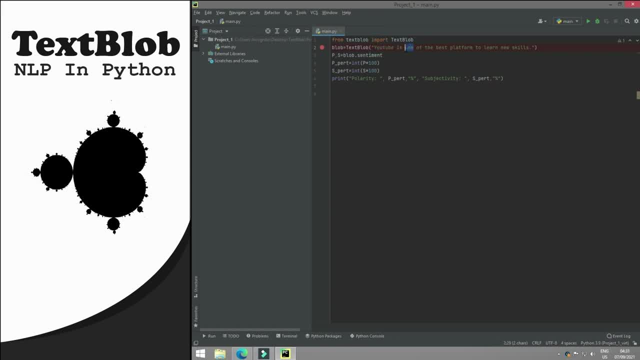 That sentence and then select any of the world by defining its index. okay, So first of all, we will go with that process. For example, I want to convert that platform world into its plural form. okay, So it's very simple. 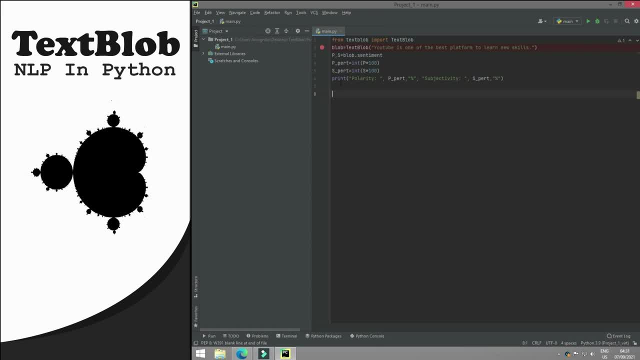 First of all, just tokenize that sentence. So just write BLOBWORDWords: okay, And I will save that list in WD. okay, And now we need to access to this particular world. So this will be at index number 6,, I think. 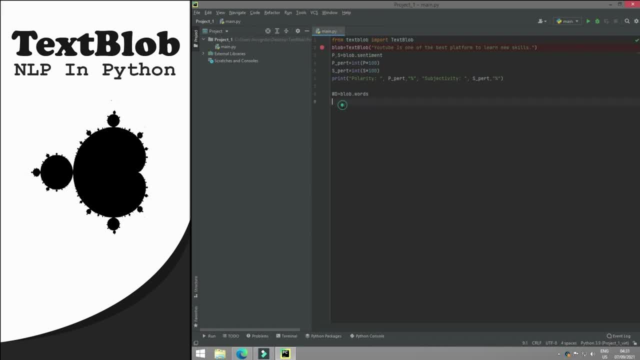 0,, 1,, 2,, 3,, 4,, 5, 6.. Yes, it will be at index number 6.. So, for example, let's print it So WD, WD and just define the index 6, okay. 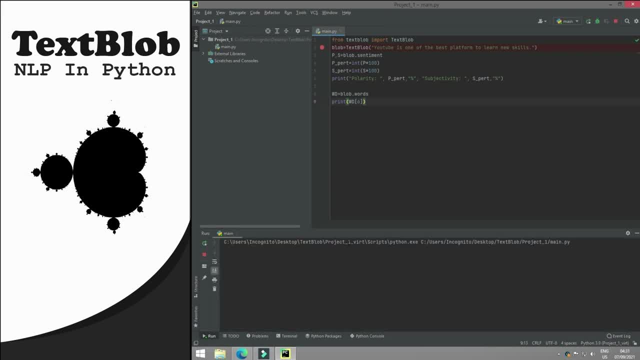 And now, if I run it, this will print: platform, Yes, Yes, platform. And now I need to convert that WD, that platform world, to its plural form. okay, So it's very simple, Just right. here I will create another variable and I will say it like P: okay. 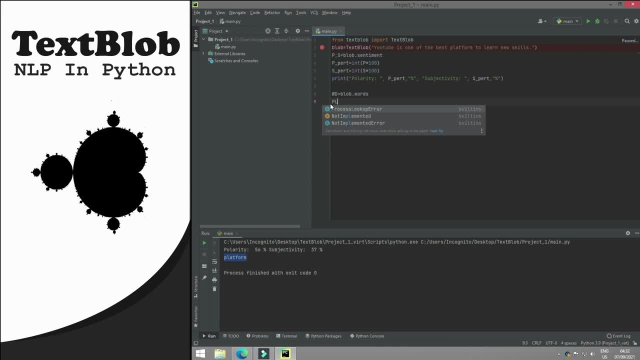 Or PL- PL plural. okay, And is equals to WD index number 6,. dot pluralize- PLU pluralize- okay. So this pluralize function will basically convert that singular into its plural form And then we need to print that PL- PL okay. 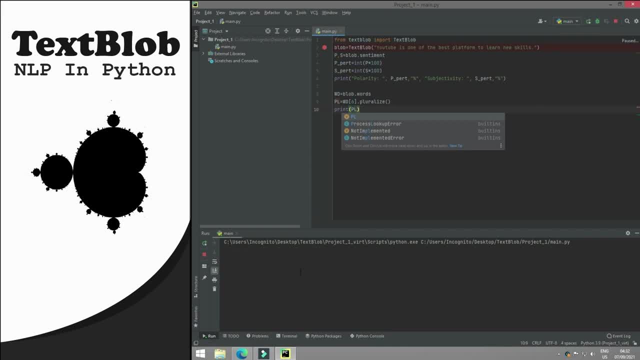 And now you will notice that we will get the plural form of platform and that is platform. So awesome, awesome, You have done words inflection in text below. And now, for example, if I don't have the sentence and I need to perform a words inflection operation, 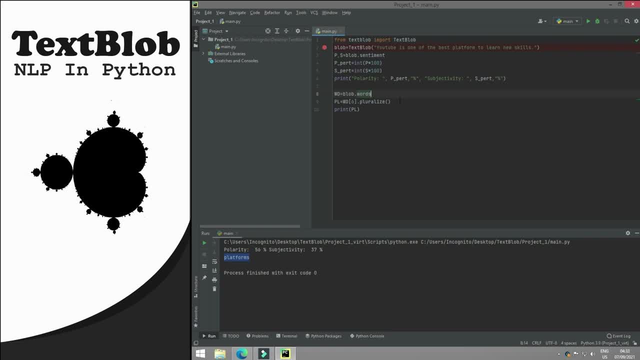 on a sentence. I need to do a single word, okay. So it's very easy, It's very awesome, And I want the user to enter that word in the terminal, okay. So first of all, let's create that function, the input function, okay. 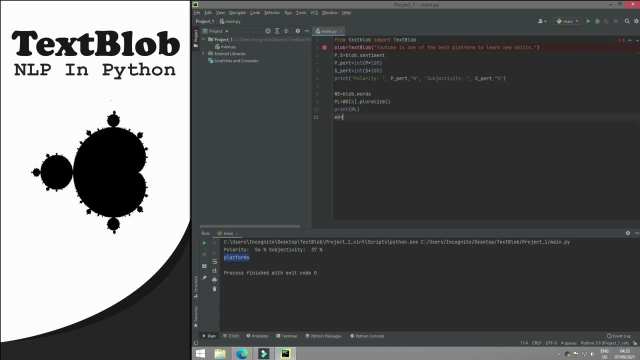 And I will say that word in WD is equals to INPUT, INPUT, not capital INPUT, input. okay, And I will say ENT, ENT, enter in the terminal And I will say that word in WD. And now I need to convert that word to its plural form. okay, 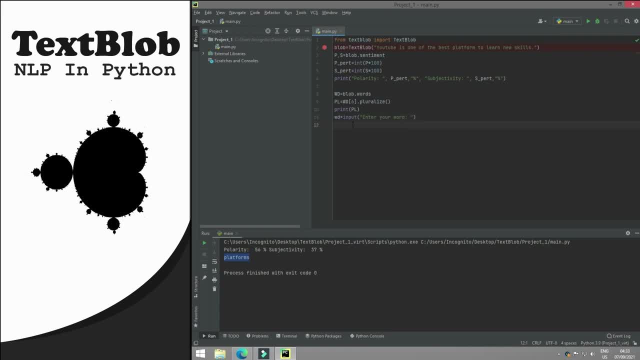 So I need to move that word to a particular class that is called words. okay, So I will import that class from text blog: IMPORT- IMPORT- W-O-R. IMPORT- W-O-R- rd world. okay, and then i will say: result: r-e-s-u-l-t result or raw result, r-a-w-raw. 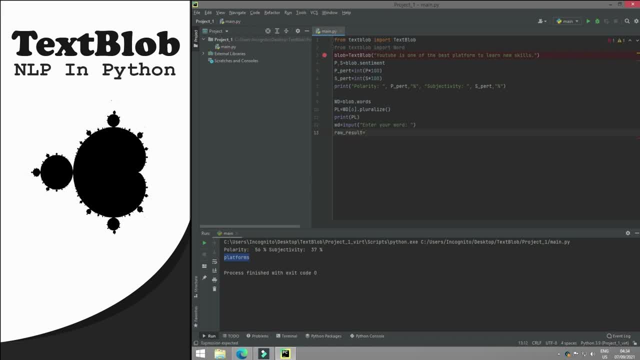 underscore result is equals to world. okay, and then i will pass that to world here. okay, so world and wd. okay, and now i will perform my operation on this particular variable. so i will call r-a-w- underscore result dot. p-l-u pluralize and i need to print it. okay, so just print it. p-r-i-n-t print. 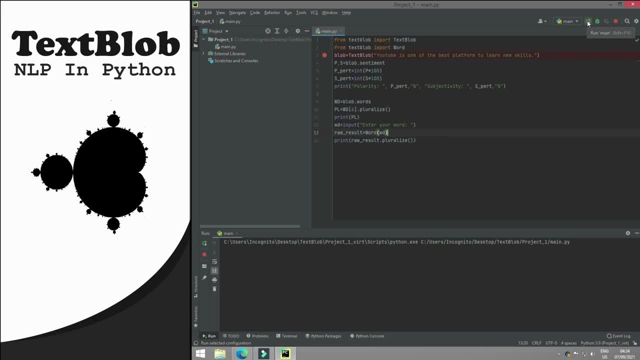 okay, and now everything will work fine, i hope. yes, enter your word, and i want like a double p-l-e: apple and- and yeah, apples are my plural of this word. okay, and now what i want? i want to convert a plural word into its singular form. okay, so it's very simple: just copy the same code. okay, and just copy. 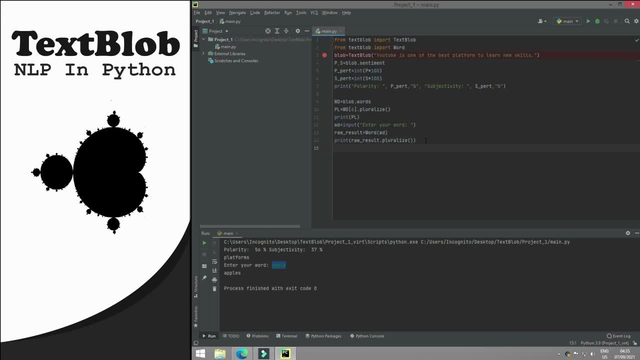 it, or and paste it here and just change the variables. it will be my singular, okay, singular. and round the score: result, underscore, singular, okay, underscore, result, underscore, singular. and now instead of pluralize, i will say singularize, s-i-n-g-u. singularize. and if i run it first, we need to interrupt the singular word so that it: 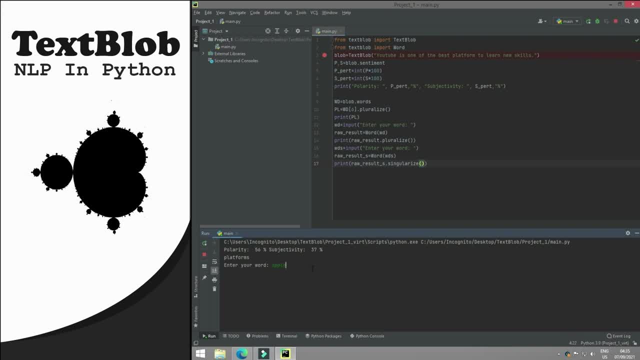 will convert it to plural words. so, okay, add up a p-l-e apple, and yeah, here is my plural. okay, and now i need to enter a plural word and i will call it like p-a-l-l-s balls, and yeah, here is my singular. so we can do m-o-n, while the score results will be p-e-a-l-l-s. 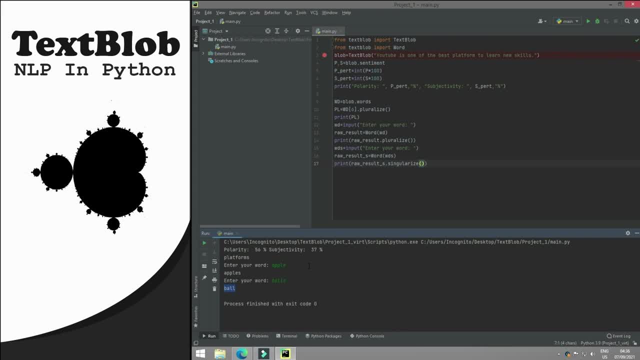 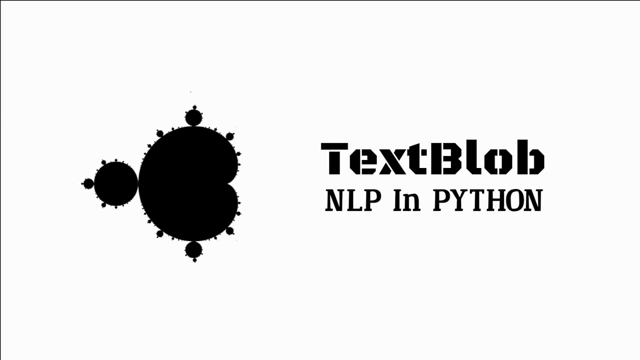 and we just change the cold computer aerial Boh Snap again like this. ok, let me tell you it is similar to m-o-n, since it is something that only works. Competitor, okay, so that's how you call it exactly. now let's see how it works, how lemmatization works in TextBlob. so let's begin the lecture. first of all. 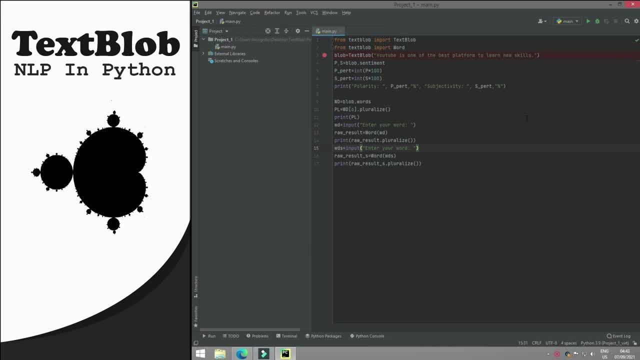 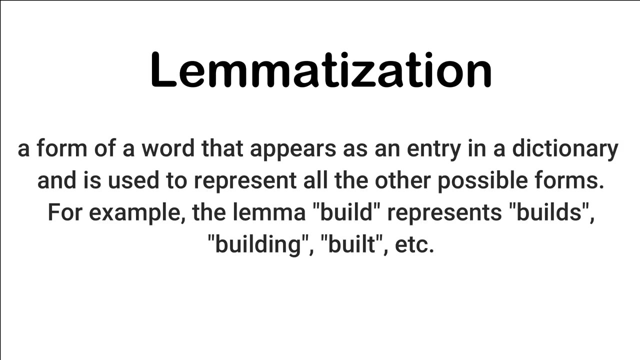 before I jump into coding, it is very important to understand what is lemmatization. okay, and in order to understand what is lemmatization, you need to understand what is lemma. so, according to Cambridge dictionary, lemma is a form of a word that appears as an entry or a tag in a dictionary and is 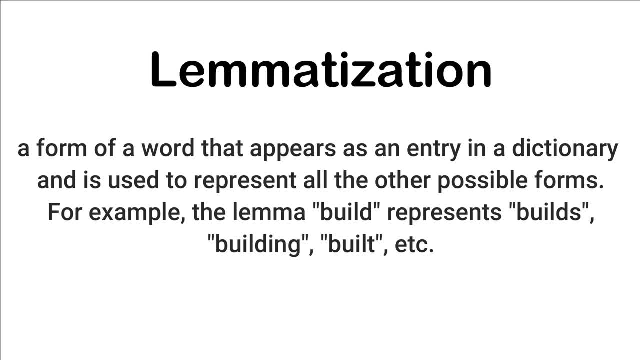 used to represent all the other possible forms. okay, so I hope you have understood. for example, build- okay, build is a word and it represent builds, building, built okay. so built is build okay. so build is build okay. so build is build okay. so build is basically a lemma or an entry point or a tag for builds, building and build okay. so i hope you have. 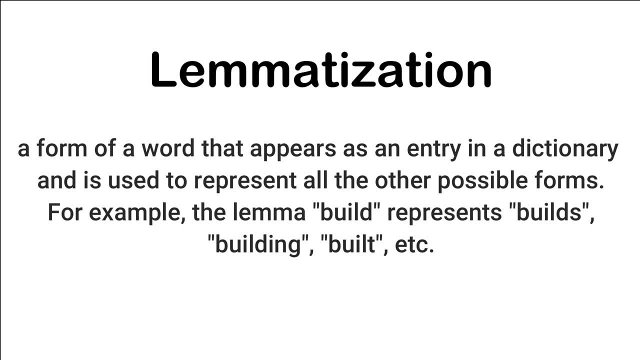 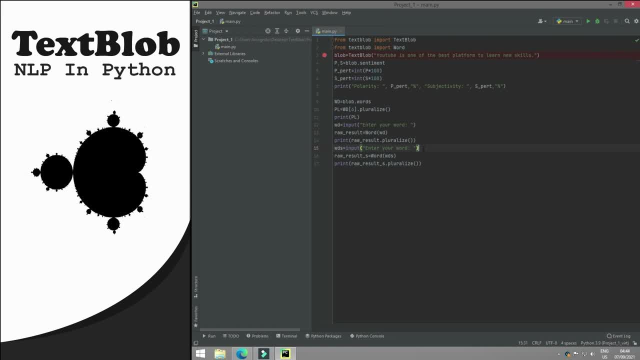 understood what is lemma and what is lemmatization, and now let's jump into some coding. so i am on my pycharm and previously we have done how to perform words inflection in text blob and now we will see how lemmatization works in text blob. so remove everything. okay, remove everything, and 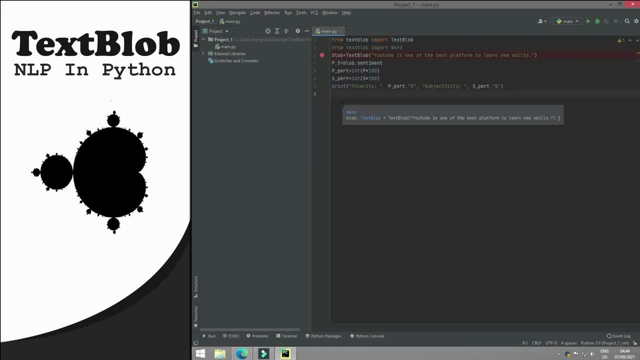 now what i need. i need to convert words into its uh entry point or into its tag world, okay, so i will also take uh user input, okay, and then i will convert that word into its uh entry point or into its lemma, okay, so just write here: wor or WD is equals to I, NP, UT input and write ENT or into you. 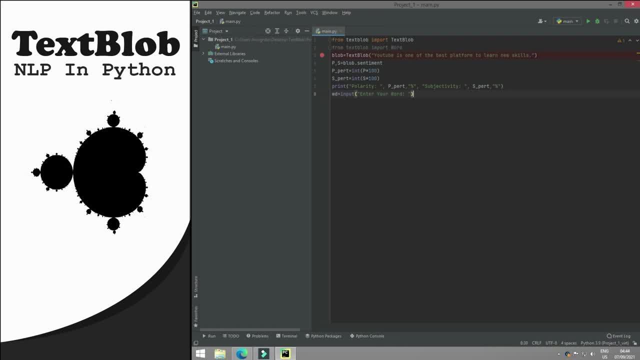 or world, okay, enter your word. and then I need to convert that toward our add W raw is equals to W or the world, okay, WD. and now I need to convert that drop into its lemur form. okay, so I will print. print our a W rod or lemur lemur ties. 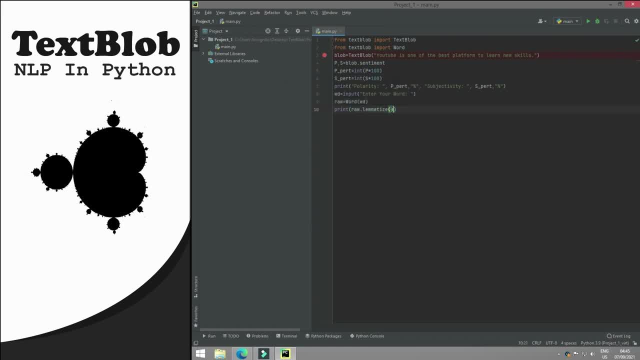 okay. and now inside this two rounded brackets, I need to pass the parts of speech in which I want to convert it. for example, in this case, I will go with verb okay and we represent my verb okay. and now, if I run it okay, I need to enter my world and, for example, I will go with like view I LD. 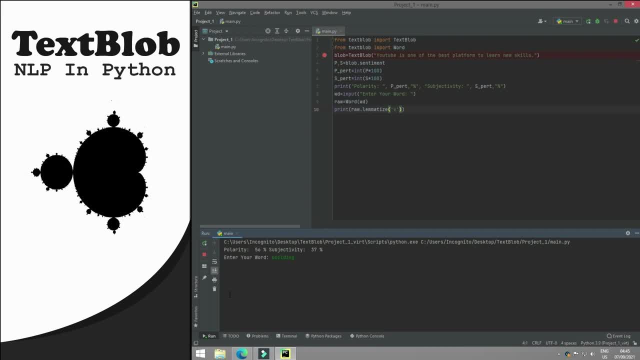 ings buildings, okay, and yeah, build is the lemur of building, okay. and now, if I run this thing again- and this time I will enter something else, like what? like vetted W, a ITED, vetted and it is performing its operation and, yeah, that is the lemur of vetted, okay. so this: 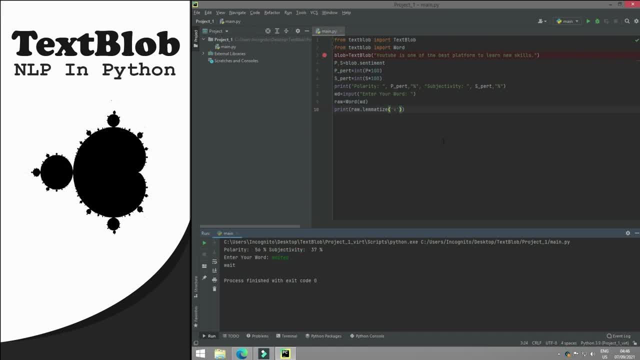 is how limit ization works in text blob and how simple it is. just by writing a single function, lemur ties, and it converts our world into its lemur form. okay, so I hope you have understood. so in this tutorial we will see how to check for spelling mistakes in a sentence using text block. 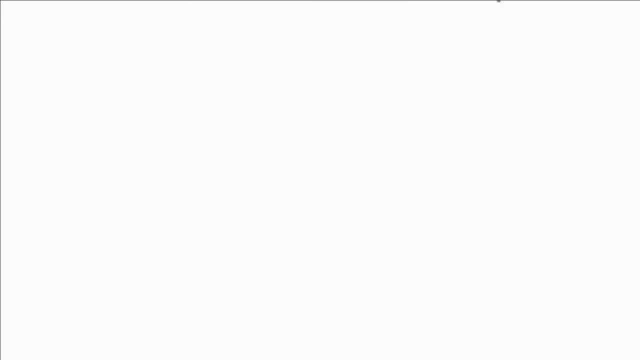 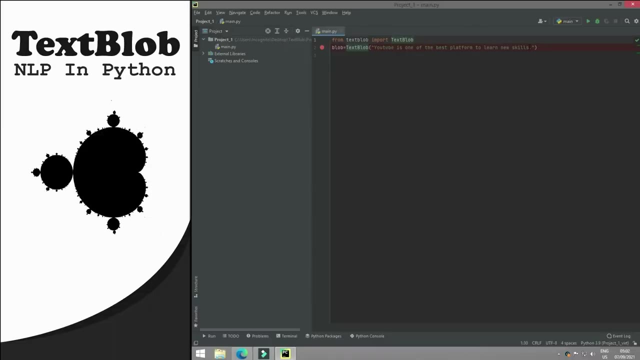 library. so let's begin the lecture, okay. so first of all, let's write here a wrong sentence, okay. so again, keep in mind, performing any task in text block consists of two things: okay: creation of your string. okay, and then performing operation on that string. okay, so first of all, let's create a wrong sentence. 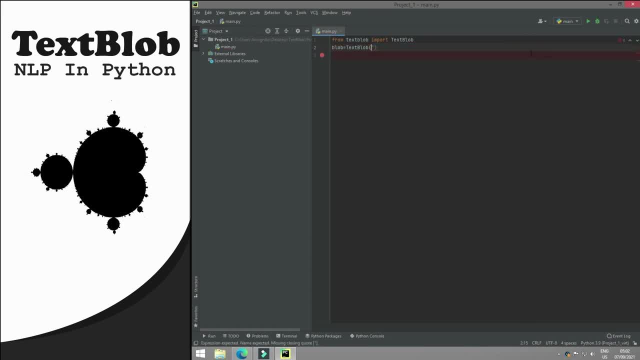 here, and in this case we are going to create a wrong sentence here. so first of all, let's create a wrong sentence here, and in this case I will go with like: I have good g-double-odd, good triple-odd, good spellings- s-p-e-l-i-n-g. I have word spelling okay, so now I need to perform a. 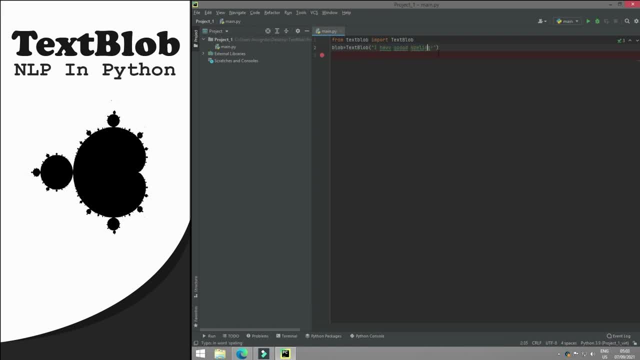 spelling correction operation on this sentence: okay. so it's very simple, just right. here I will substitute block correct in s-p-e-l-i-n-g text blob dot correct. okay, CRRR connecting block dot correct and our the cell this sting in naughty and descent variable and then, after print that variable, STNT sent and if I run it, yeah. 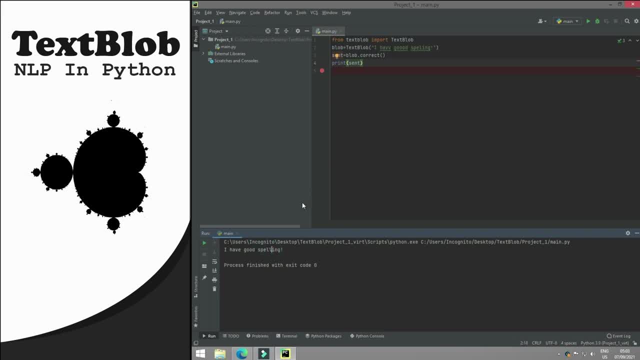 here is my correct sentence, and that is: I have good spelling text- blob. okay, so you can also check for the list of suggested words. okay, and you can also check its confidence level as well. okay, so it's very simple. instead of correct, or I will say that new variable LST is equals to BLOB, BLOB. 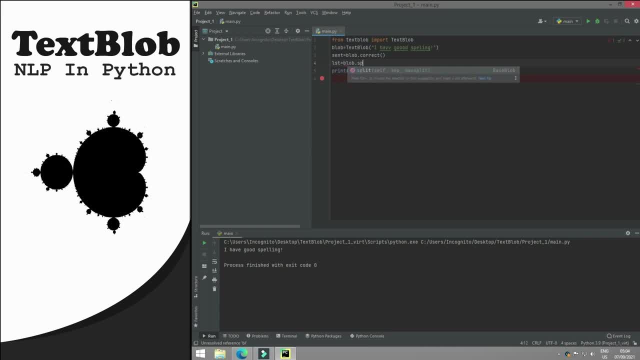 dot. I will say: spell check a, S, P, E, double L, span he pen, c, H, e, c, K. spell check okay. and then I will print heroic esos. pr translate: enter at print: επرا instrument, that list ㅠ ЛСТ. and if radha mail, if I Jordan will ill 갖고. 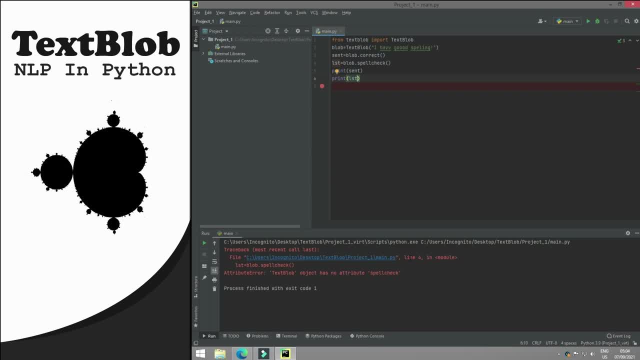 it. okay, so we got an error. basically, we need to define a certain world on which we want to perform that spell-check method. okay, so, let's see. okay, so, let's see. so, for example, i want to check this world. okay, the list of suggested worlds and its confidence for. 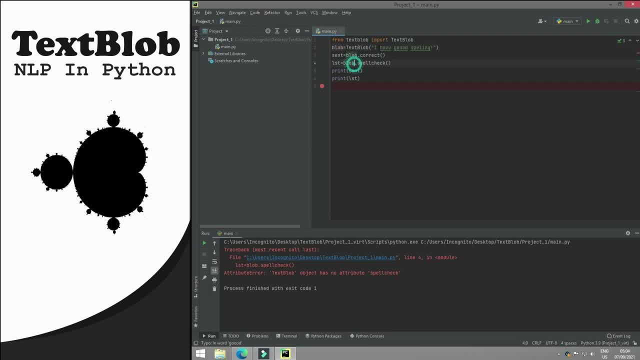 this word g, triple, o, d got okay, so it is at position zero, one, two. okay, so just right here: two and not two. we need to actually convert that thing into first tags and then we can check it. so just right here. but instead of converting the whole thing into tag, i will say blob dot words. 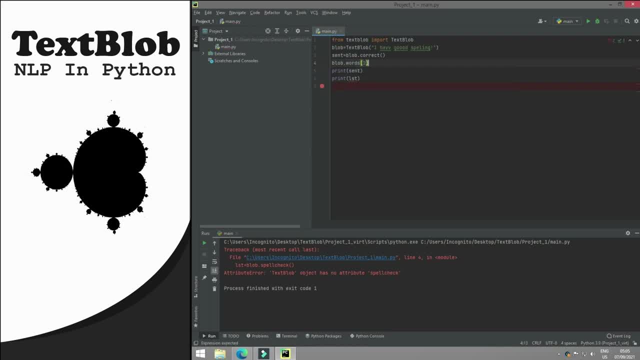 and then i will pass the index, which is two dot spell check, s, p, e, double l spell, c, h, e, c, k spell check. okay, and now it will work fine, and i need to uh save this thing in a lst variable and if i run it, yeah good. 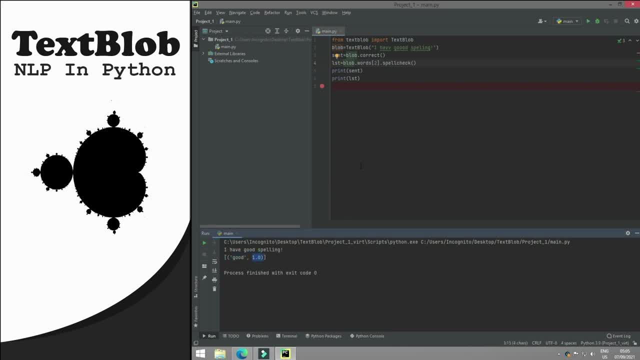 so so and for example: uh, let's go with the, let's change this thing, okay, and instead of good, i will call it like t r e t great, okay. and now let's check this world and, yeah, here is my list of all possible words and their confidence level. okay, so great. its confidence level is 0.5. this means 50 percent. 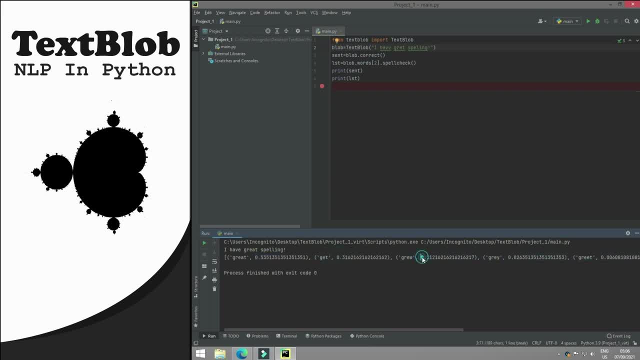 great is 30 percent, gree is 0.1. 60 percent. gree is 0.8. we in this means 10 and gray is uh just 20 percent. uh, pho example. if i perform spell check operation, you have noticed that it has depressed. 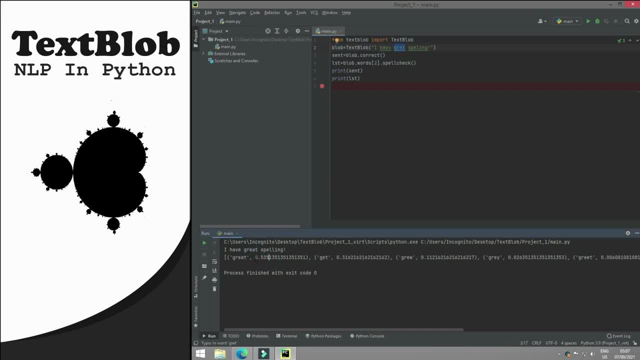 50 percent faculty secretive product marketing grade with grad because its percentage or its confidence level is highest in all the list. okay, so this is how you can check for us um confidence level and all suggested words. okay, so this is. writers wrote this against the standardinka when i create a written我是 ikke the word for and all suggested words. okay, i should use this when i do a CH to reduce all of you's values like protestance, to increase confidence, and there are many other suggestions. all um other lessons. okay, please do not neglect this video. so did not enjoy. notice content self as well. 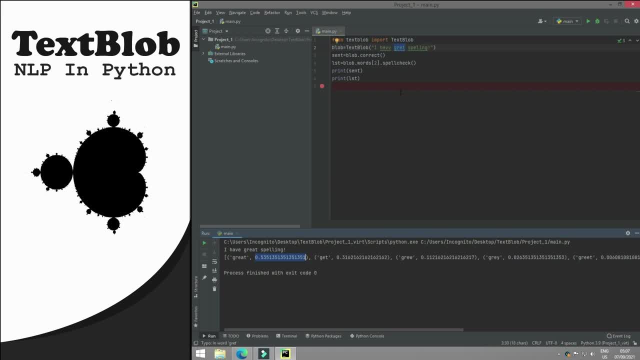 so i hope you have enjoyed this tutorial and just play with these things. okay, for example, convert that value into percentage. or you can actually make your own app, like grammarly okay, in which you will check for spelling mistake for noun phrases, mistakes for sentiment analysis, awards, inflection or limitization. okay, so you can create your own grammarly app as well. 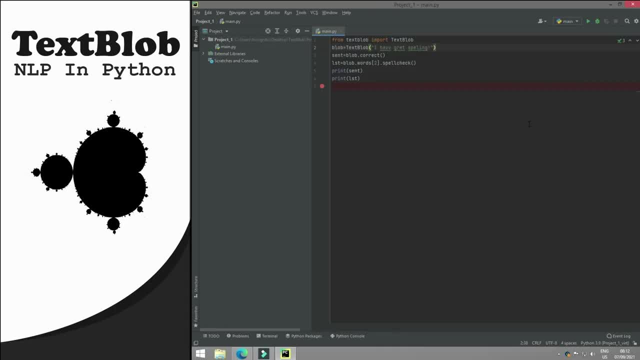 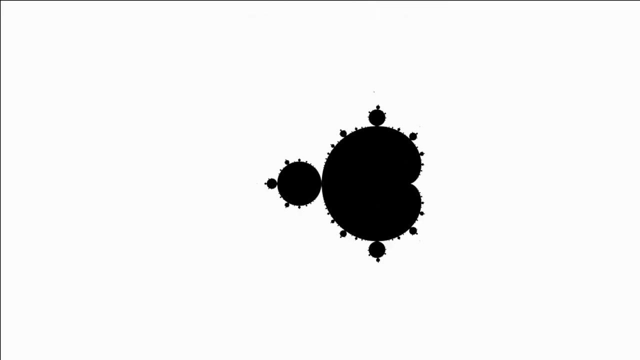 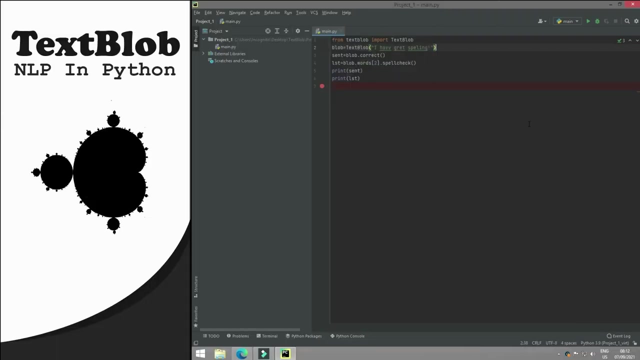 so in this tutorial we will see how to check the frequency of a certain word in a sentence, and we will also see how to check the frequency of noun phrase in a sentence. so let's begin the lecture. okay, so previously we have done how to check spelling mistakes in a sentence, and now 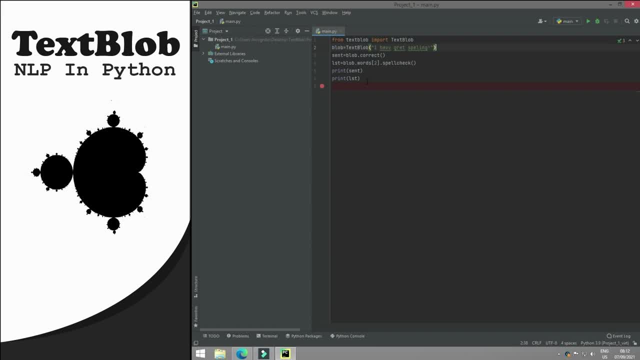 we will see the frequency, or how frequent this word is present in a sentence. okay, so it's very awesome. and there are two methods, okay, the first one is to use a dictionary and the second one is to use a method. okay, so first of all, we will go with the dictionary, okay, 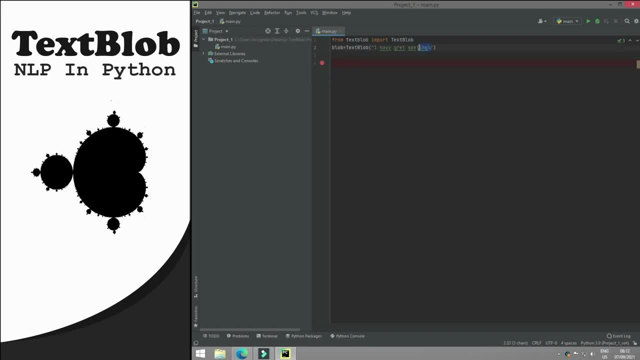 just remove everything and instead of this sentence, I have copied a sentence. okay, and this is okay, so just just make it together. this is my sentence, okay, and we will check, check this world, okay, eki, and we will check how frequent this world is present in this sentence. so first of all, I will go with dictionary. 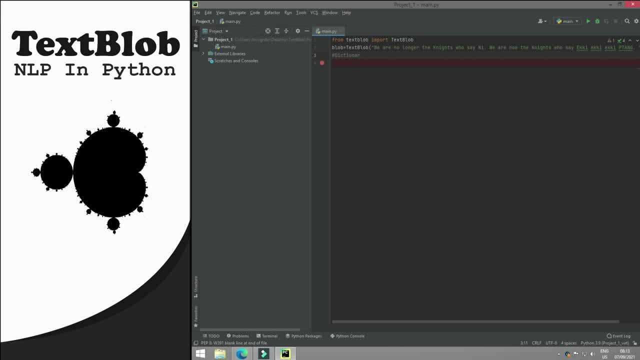 method: okay, dictionary in our dictionary. okay, and just right here. blog dictionary. okay and just right here. blog. okay and just right here. blog dot. world underscore count: okay, so this is basically dictionary and we need to define here a certain word. okay, and I will say like e, double K, eki and I need. 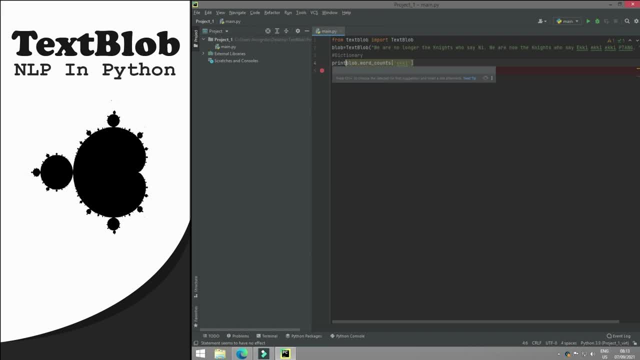 to print it. so just write print. okay, print it. and if I run it, you will see that this certain word is present three times. and yeah, this is my answer. we can use yes or no to check that, i'm sure. okay, so what I will do next? and is talking about other names. an example: 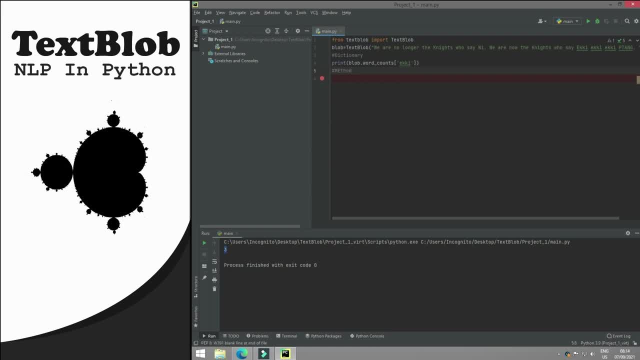 which is three okay, one, two and three okay. the next method is to use a built-in method- okay, so this is my third, and in this case we just need to write here: blog door to walls dot count, okay. so blog naar towards dormand. here we need. 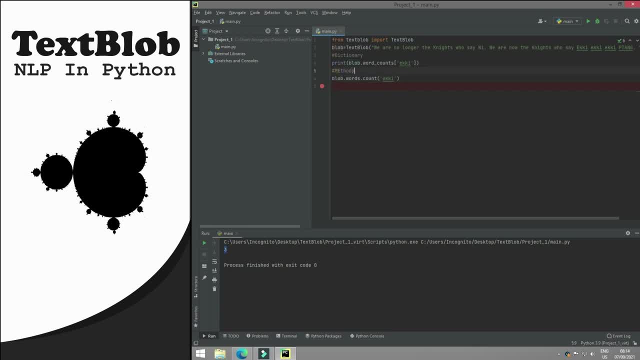 to pass our rule and that is a double KI eki and we need to print that world as print the amount as well. so, just right here, print, p r i n t, print, okay, print, and this will print three as well. okay, and yeah, here is three and here is three, okay. so one more feature that 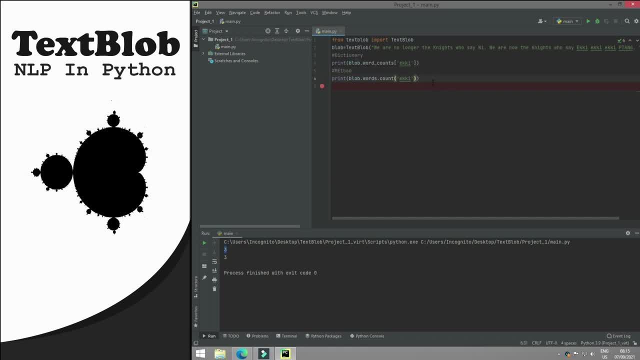 this method provide us is that can check for cache sensitive world as well. so, just right here, c a s e cache underscore s e n, s, i t i v e sensitive is equal to true, and now you will notice that it will return just two. okay, this is because this e key is present two times here, okay. 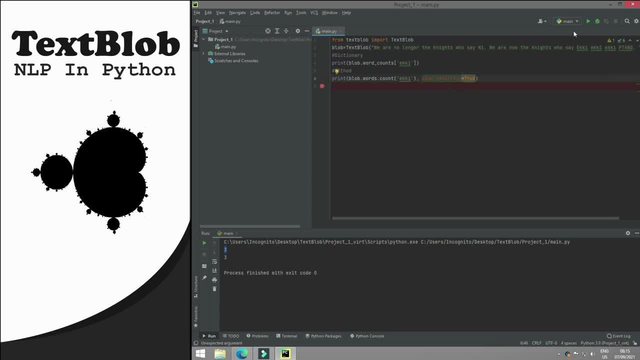 if i apply this cache sensitive to true, so if i run it, you will notice that our first answer will be three: okay, so we got an error and that is cache sensitive. okay, so sorry, we just need to remove this rounded brackets, okay, and put bracket here, and now this will print two here, okay, yeah, here. 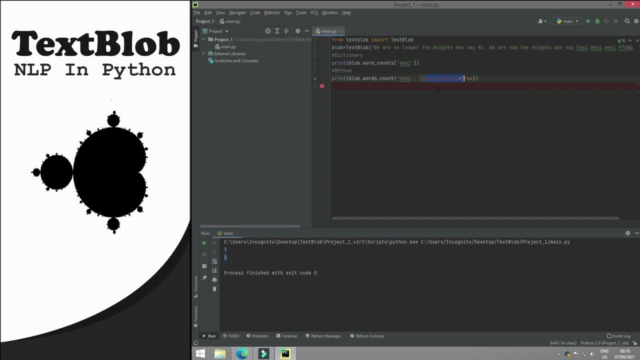 is two. okay, so this is how this cache sensitive value works. okay, so this is basically a boolean, and if i increase this e and then you will notice that it will now print one because it is present to one. okay, so, yeah, here is my answer. so this is how you can check how frequent. 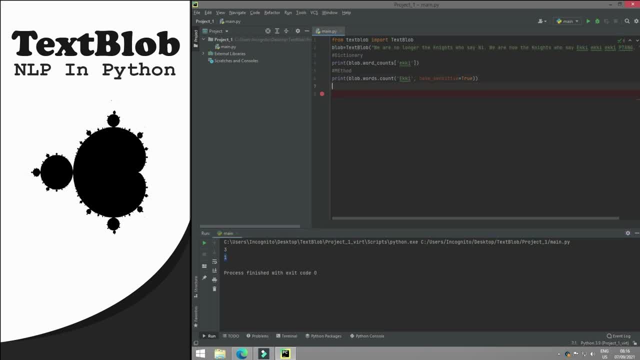 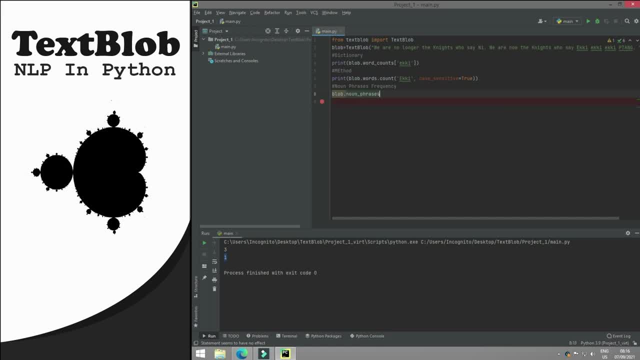 blob, dot noun phrases: dot count, okay, count, and we need to count what thing like nights? okay, and dot count and we need to count what thing like nights- okay, and we need to print it. okay, just right here. we need to print it. okay, just right here, print and just print this thing and if i run it, okay, zero. so 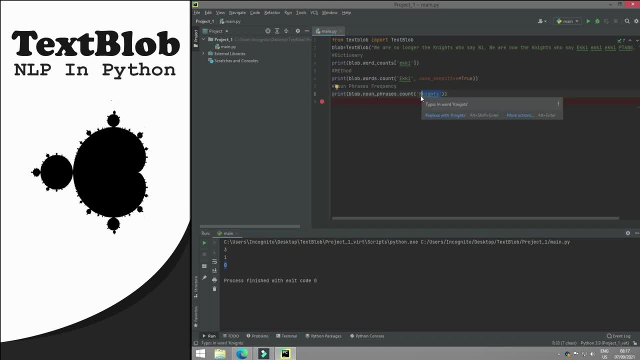 print and just print this thing, and if i run it, okay, zero. so basically knight is not our noun phrase, basically knight is not our noun phrase, okay, so now, first of all, let's print noun phrases. okay, so, okay, so now, first of all, let's print noun phrases. okay, so, just remove it. noun phrases, okay, and yeah. 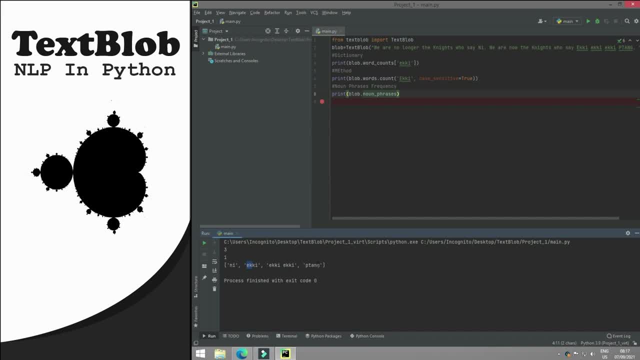 aroma contour. okay, and now i need to pass my phrase and that's okay. and now i need to pass my phrase and that's, that is p t a n g. okay, and you will notice that it will return three. okay, because this particular noun phrase is present three times in this sentence. okay, so it is processing and yeah. 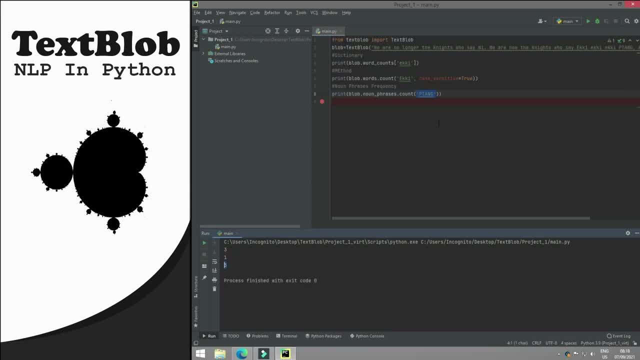 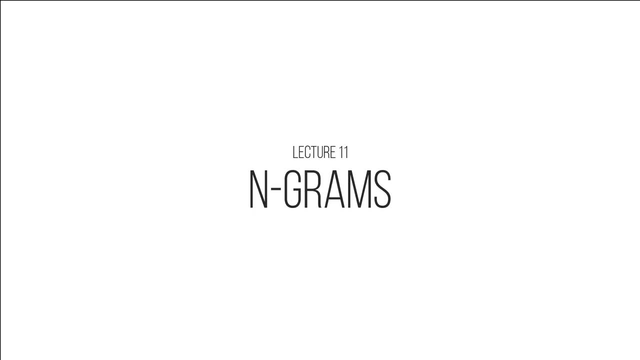 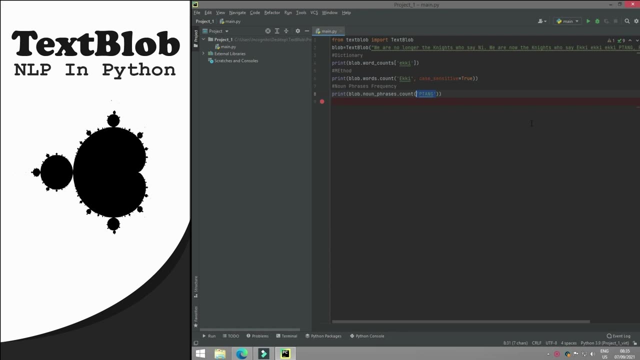 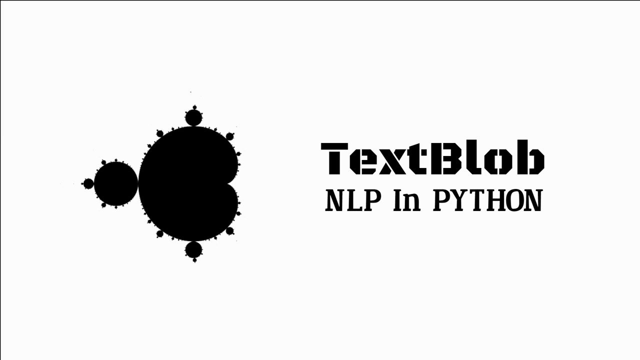 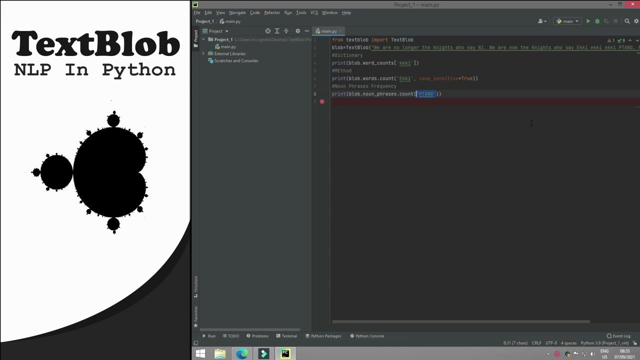 here is my answer. so this is how you can check for a noun, phrases frequency and words frequency. so i hope you have enjoyed this tutorial. so in this tutorial, we will see how to perform n grams method in text blob. so let's begin the lecture, okay, so first of all, uh, instead of jumping directly into the code, you just need to understand. 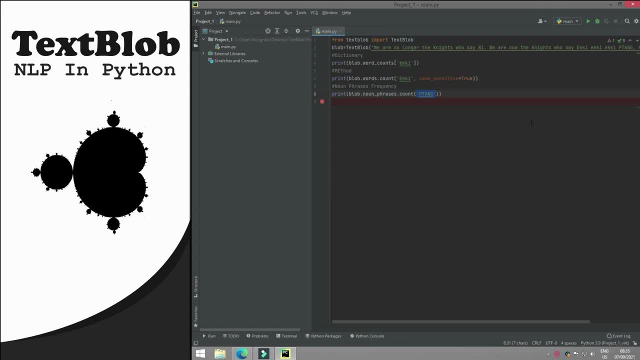 what is n grams? so n grams is one of the most important concepts in data sciences. okay, so it is very much important and it helps us in many scenarios. so, basically, n-gram methods, let us divide a sentence into n number of words. okay, so it divides a whole sentence into. 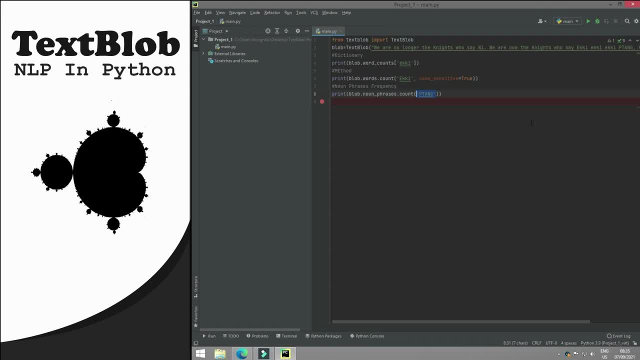 lists and each list contain n numbers of words which we will define later. okay, so in real-world problems, problems regardless of letters, we will describe words for each letter which are digital, and grams basically help us a lot. for example, according to a recent research, if we use three, 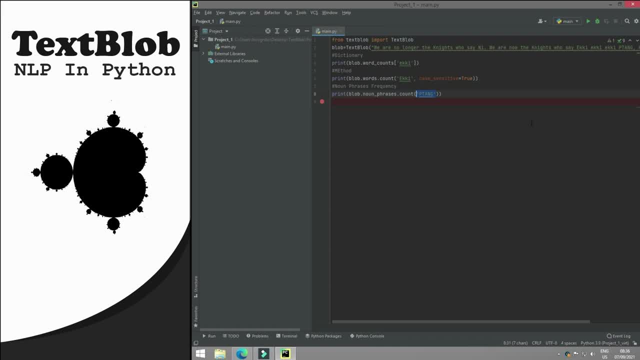 grams or four grams method. it helps us to filter scams, emails or, in most cases, two grams help us in data sciences. we use n grams in probability as well. okay, but i will not go deeply into it because i am assuming that you are an absolute beginners. okay, and all of these things will make 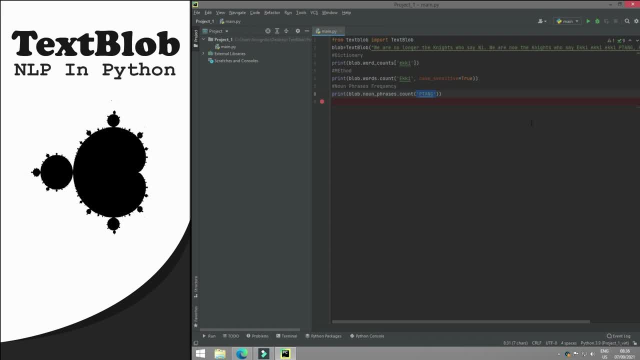 you confused, okay, but i will just show you how to perform n gram operation in text blob. okay, so you will get a better understanding. first of all. uh, just remove these things, okay, and i will perform n gram operation on this blob. okay, so you will get a better, a better understanding of n. 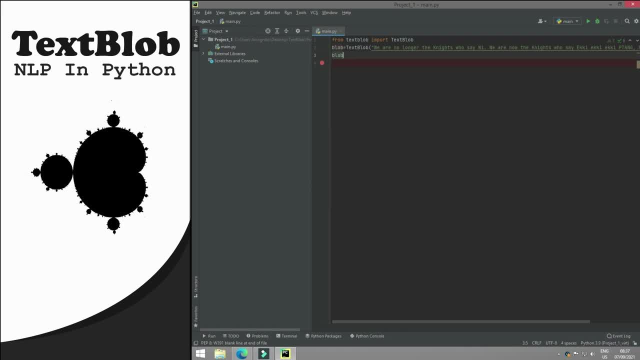 gram when we will do practical work. so just right here, blob dot n grams, okay, n grams. and now we need to do define the n value. okay, so this n gram basically represent n number of grams. okay, and we will define that value here and make sure that your value should be integer, not float, nothing else. 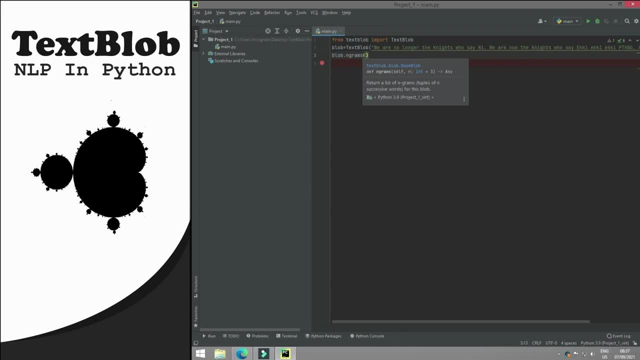 okay, it should be integer, for example. for now i will go with like three grams. okay, so just right here, three, and i will save the result in a variable and i will call it like: g is equals to, and now i will print g, we will get a list and then inside that list we will get sub list. okay, 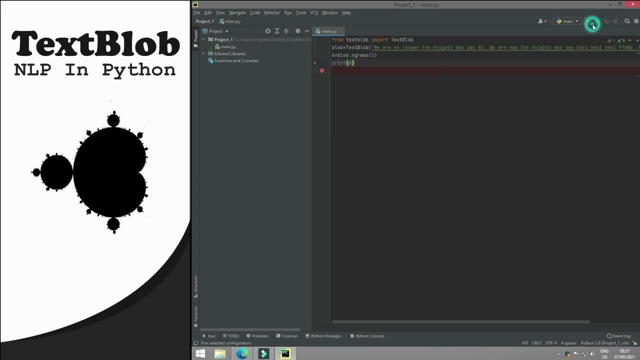 so like a multi-dimensional list, i think okay. so if i run it, yeah, here is my main list, okay, so here is my main list and inside that list i have sub list. okay, so this is my list number one, this is my list number two. this is my list number three. okay, so, uh, this three basically represents. 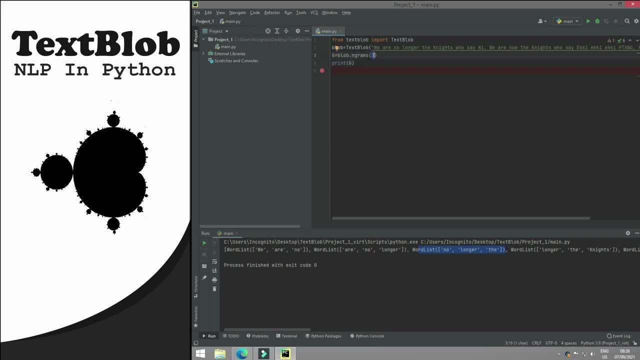 our g, g and you have noticed that, uh, this three has divided our this sentence into a list, and then inside that list we have further list, with each list words of three, okay. so, for example, just look at this list, we are no, okay, we are no, so we have three words. and then just 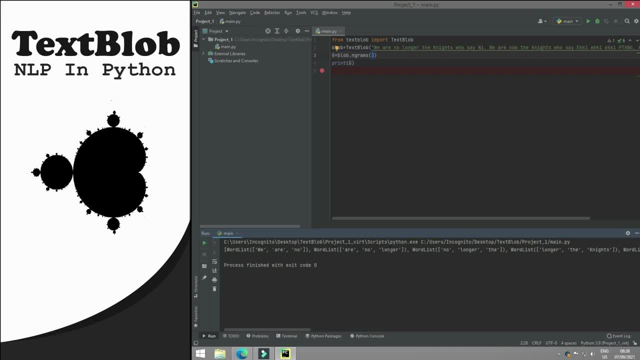 look to this sentence are: no longer it has three words. no longer the it's has three words and longer the knives. okay, so it has three words. so this is how n grams work. okay, so if i replace this three with two, you will notice that this list will have only two words. okay, so if 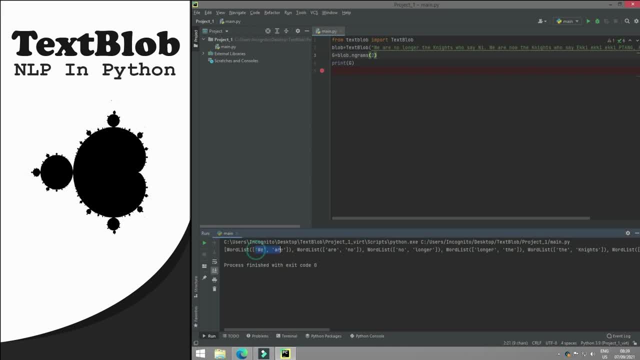 i run it okay. so now we we have only two words in the list, okay, so v r r, no, no longer longer d. okay, so this basically help us to filter uh scams, okay, or to find the probability as well, okay, so, uh, you can actually play with these lists, like you can find the total length of this list, okay, or? 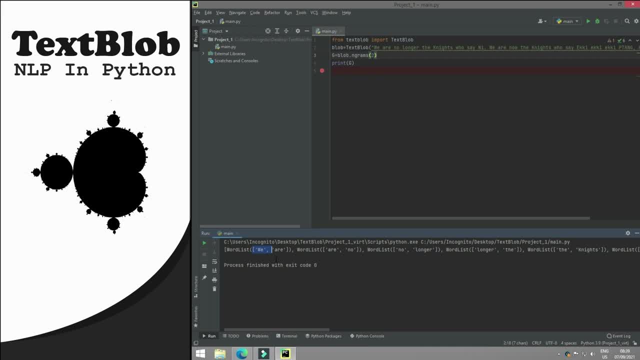 you can print each of these lists separately. you can perform certain type of operations on these lists, okay, so i hope you have understood. uh, what is n grams? okay, i know, i know that you still have so many questions regarding n grams, but keep these questions for your future research, okay? 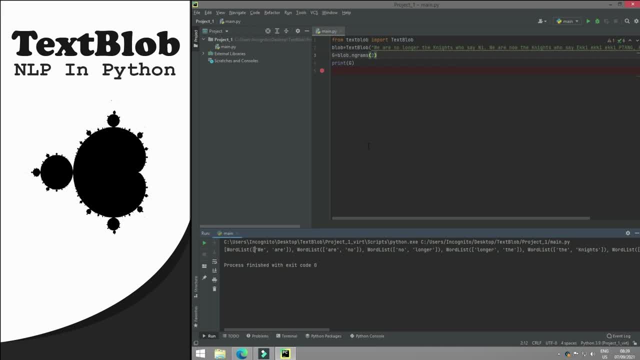 so keep yourself curious about uh and grimes, because this concept really help us in real world scenarios. so in this tutorial we will see how text blobs act like python string, so let's begin the lecture. okay, so first of all, uh, just to remove these two lines, and let's remove this sentence and write a. 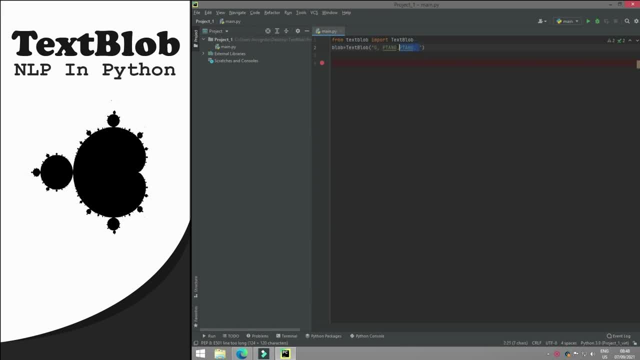 simple sentence. okay, so just remove it, and there i will write like this: t this is my simple s-e-n-t-e-n-c-e sentence. okay, so this is my simple sentence, and now we will see how these text blocks. so this is my text block, how these text blob act like python string. so it's. 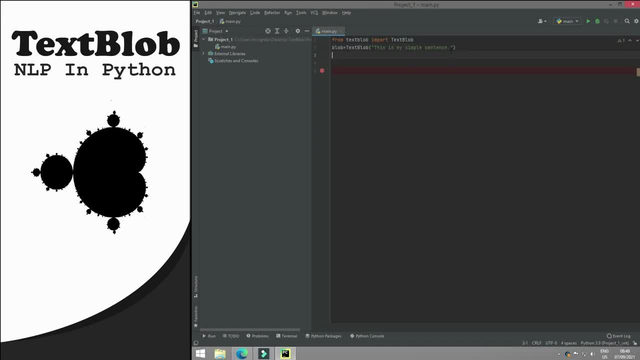 very, very simple. for example, for example, we, i want to convert this whole sentence into capital letters, okay. so i will say: uh, just write blob dot u double p e r upper, okay, and i will say that this sentence into a variable, i will call it like: up is equals to this. and now i will print: is up. 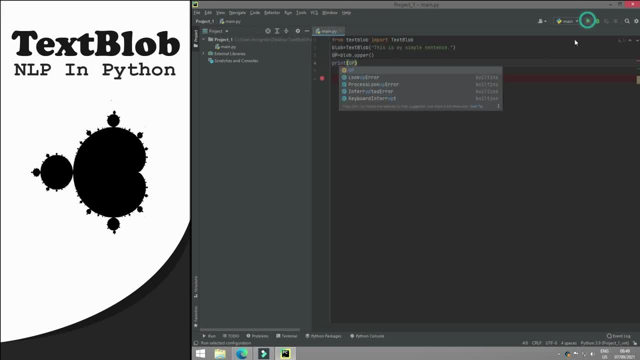 okay, so print up and you will notice that this upper method will convert my whole sentence into uppercase letters. okay, so this is my sentence. this is my simple sentence. okay, it's awesome. and now what i can do with this. i can actually find a particular word as well. for example, i want: 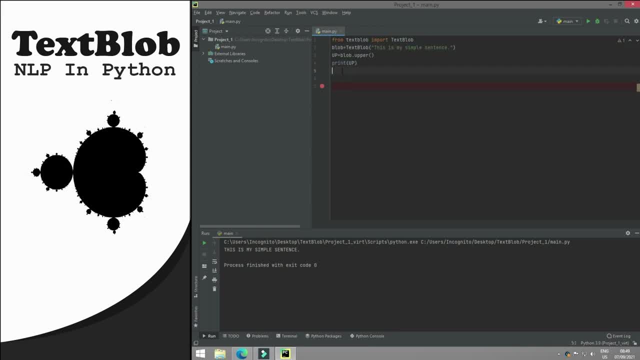 to find the position of this simple. okay, so i can write like blog, blog dot find, okay, blogfind, and i will define my word here. and that is simpl, is simple and you will notice. you will notice, for example, just print it for now and you will notice that we will get an integer value here. okay, and 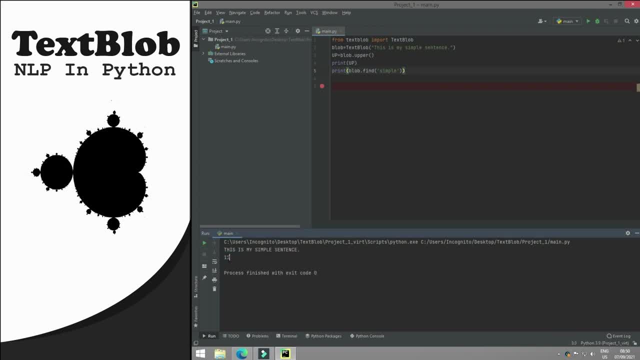 let me tell you why we are getting integer value. yeah, uh, it is, it is. uh, i saw. our answer is 11, so this means that the simple word is present at position 11. okay, and how this text plot calculated so it counts these characters. okay. so, for example, uh, t, one, two, three, four, five, space, just count the space. 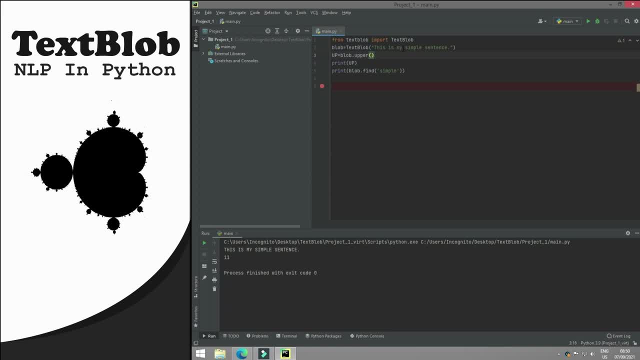 as well. okay, five, six, seven, eight, nine, ten, allow it, and yeah, here is my simple- okay, so, uh, it has defined our position, okay, so, uh, that's why we are getting this 11 here. okay, so i hope you have understood why we are getting 11, because this simple is present at this, uh, 11 position. but 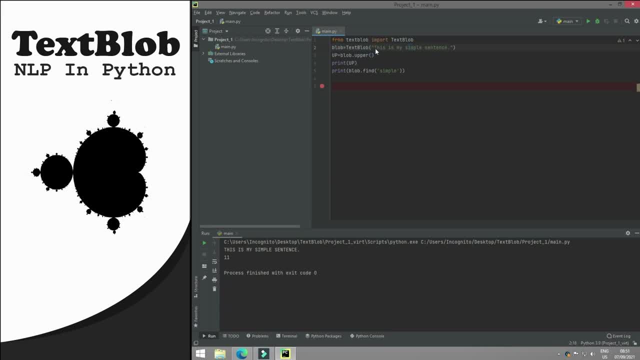 uh, sorry, i don't know why we are getting 11, because this simple is present at this uh 11 position. but uh, sorry, i counted this uh t from one. but uh, in this python everything starts from zero. so zero one, two, three, four, five, six, seven, eight, nine, ten and then eleven. so we are getting eleven. that's right, okay, so make. 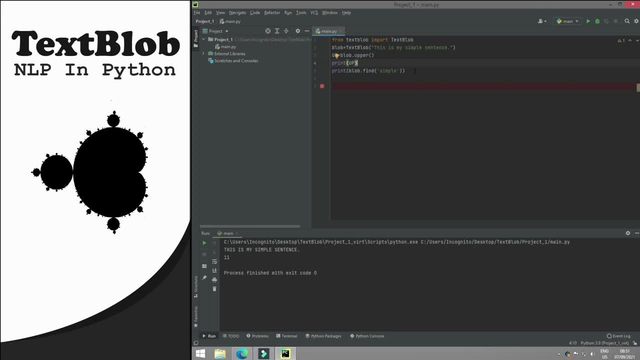 sure that you should count it from zero, okay, otherwise you will get a wrong answer, okay, and now you can actually uh compare two strings as well, for example. let's do some fun here. uh compare two strings as well, for example. let's do some fun here. uh, compare two strings as well, for example. 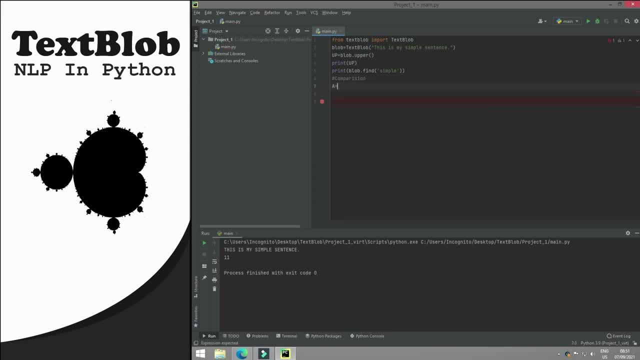 i have two blobs, okay, one is a, is equals to text blob, and i will pass apple here a double p l e apple here. and i have a next blob and that is b okay, and i will pass here banana b a double n a n a i. 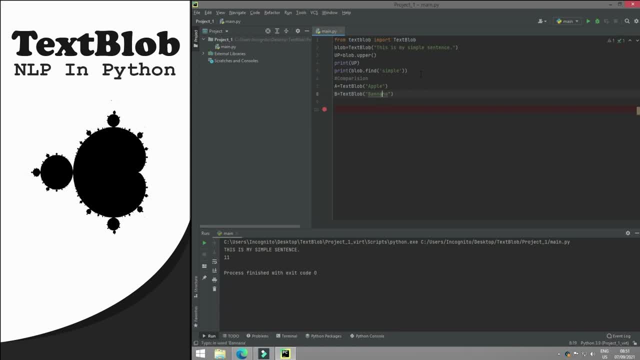 think this is a gross correct spelling: b, a and a and a. okay, banana, and i want to compare these two uh strings: okay, and if our b, if b is greater than a, okay, i print, i will print b. okay and n's and i will print, print a. so obviously, if you count the characters in 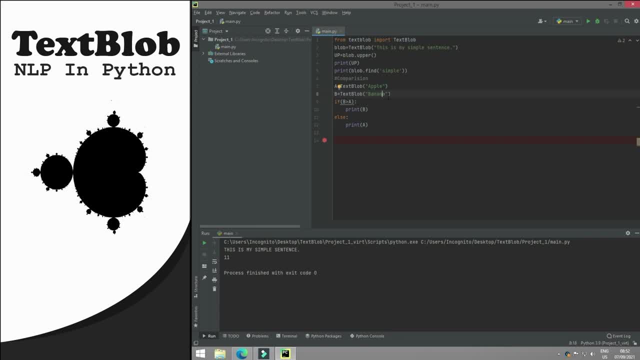 banana, you will find that the characters in banana are greater than characters in apple. okay, so if i run it, you will notice that it will print banana here and yes, so this is how you can compare two strings in text blob as well. so text blob has python string. 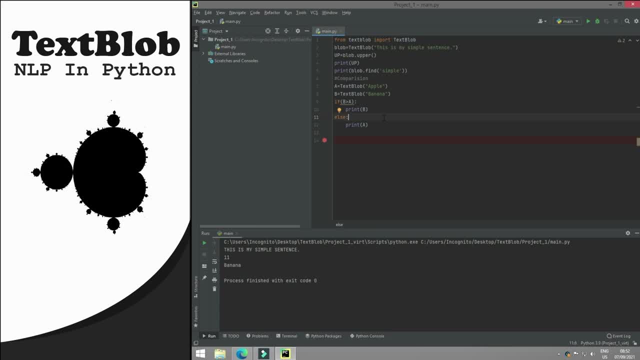 properties as well. so this was a short tutorial on how text blob behaves like python string, okay. so in this tutorial, we will see how to get the start and end indices of a sentence in text blob. so let's begin the lecture, okay. so just remove everything, okay, and let's increase the length of this sentence. so this is. 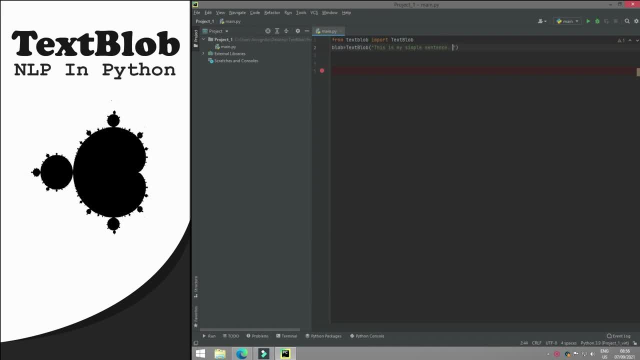 my simple sentence: and uh, uh, u b e, a u t i. beautiful is better than u? g? ugly. okay. and uh, by beautiful, not beautiful, beautiful is better than ugly. and i will say: uh, simple is better than uh complex, okay. so i have these three sentences and i want to 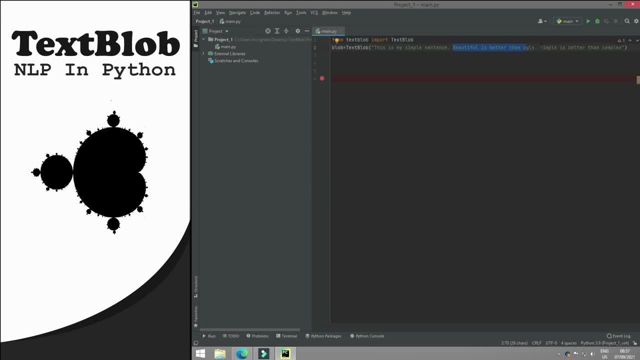 get the indices of all these three sentences: okay, the start indices and the end indices: okay. so first of all, i need to convert that text blob into sentences. uh, for example, and it's very simple, just write here: blob dot sentence or not, sentiments dot- s-e-n-t-n-c-e-s sentences- okay, i will save this list in s-e-n-t-s-e-n-t. 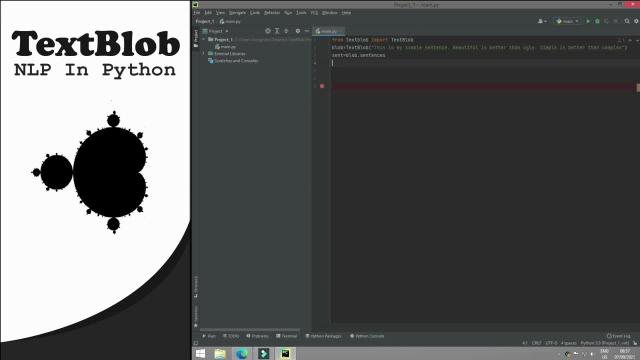 variable, okay, and if i print that variable, you will see that we will get a list, okay. so if i print it, yeah, so this is my list, okay. so this is my simple sentence. beautiful is better than ugly and simple is better than complex. so this is awesome. and now i need to loop through each. 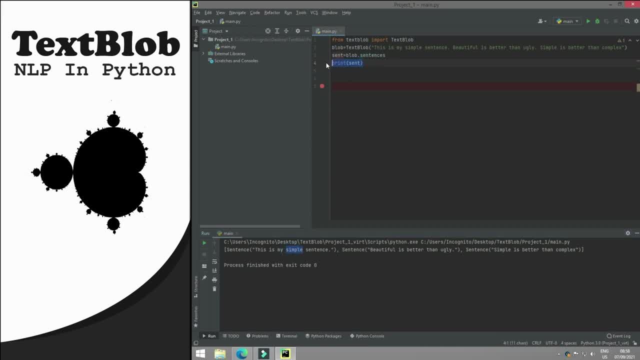 element of this list. okay, so, just right here, for uh s in s-e-n-t-s-e-n-t. okay, and i will. so this s will have you, uh, this sentence first, and then this sentence and then this sentence. okay, so, uh, this s has some other properties as well. like uh, i will just say that that st, which represents start, so 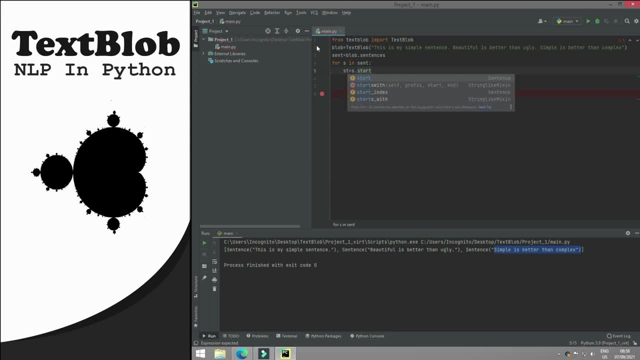 s dot start is equals to. i will print the start of. i will save the start of the sentence in this st variable, okay, and i will print the end s dot end of a sentence in this uh ed variable, okay, and then i will print it. okay. so, just right here, print and i will print the. 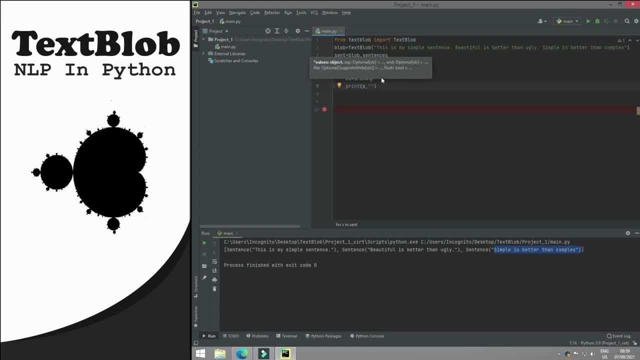 sentence first, okay, and then i will say s t a r t start, and then i will say s t okay, and then i will say end, and i will print the end of the sentence: ed, okay, and now let's run it. yeah, uh. so this is my sentence. this is my sentence and it starts from zero- okay- and ends at indices. 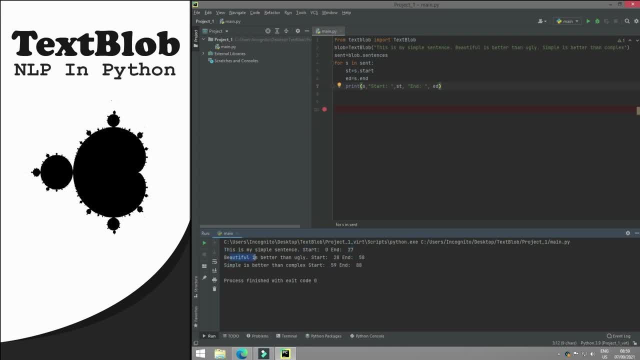 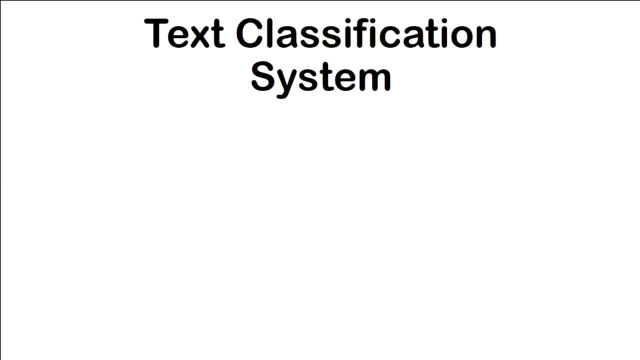 so this is how you can find the start and end indices of a sentence in using text blob library. so now we will start the development of our own text classification system. okay, so now we will start the development of our own text classification system. okay, so now we will start the development of our own text classification system. okay, you must be thinking that. 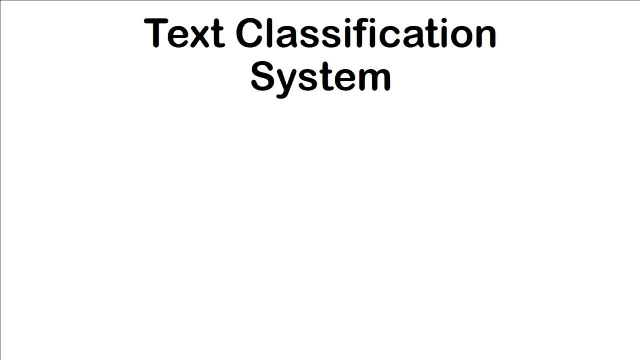 you must be thinking that. you must be thinking that why we need our own text classification, why we need our own text classification, why we need our own text classification system, system, system, because we are doing text classification, because we are doing text classification, because we are doing text classification from tutorial number one, then why we need. 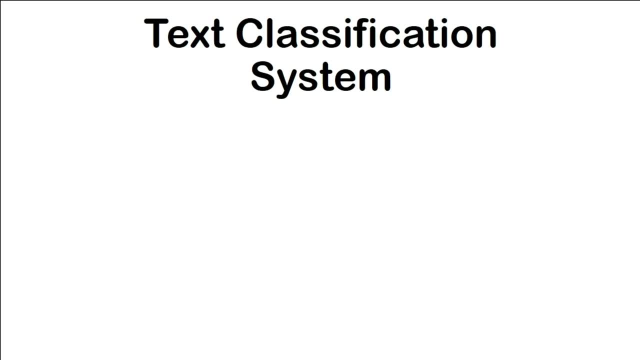 from tutorial number one, then why we need from tutorial number one, then why we need our own text classification system. so you, our own text classification system. so you, our own text classification system. so you have a very valid question. have a very valid question, have a very valid question and it's quite good if you are thinking i 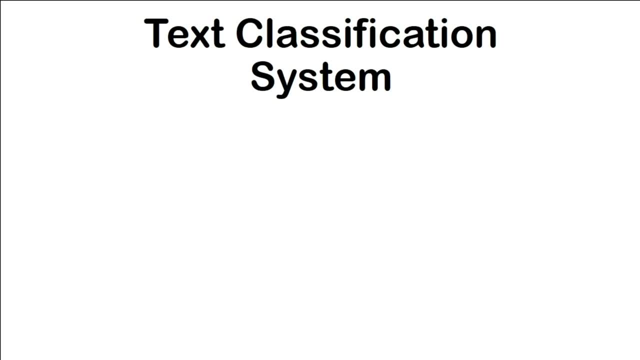 and it's quite good if you are thinking i, and it's quite good if you are thinking i really appreciate you if you have this, really appreciate you if you have this, really appreciate you if you have this question in your mind. so, question in your mind. so 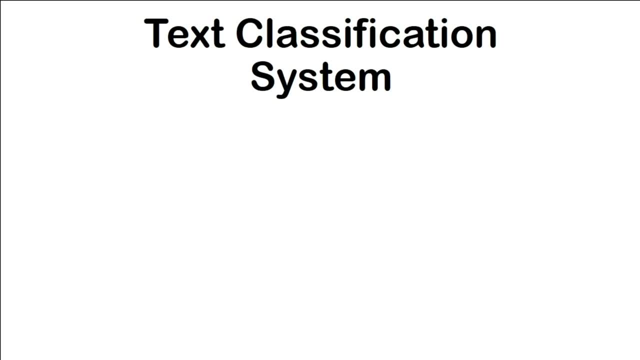 question in your mind. so, uh, we will first of all, we will develop. uh, we will first of all, we will develop. uh, we will first of all, we will develop this system, this system, this system by ourself. okay, so, we will develop this by ourself. okay, so, we will develop this. 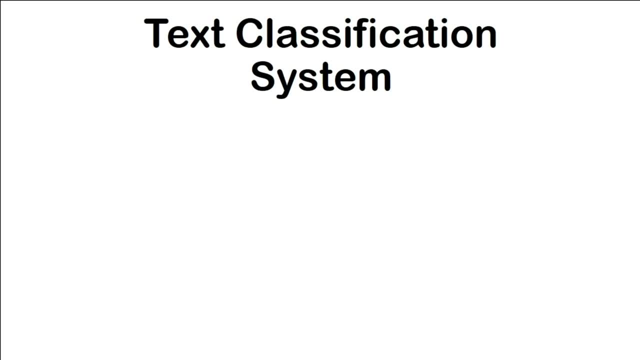 by ourself. okay, so we will develop this text classification system, text classification system, text classification system, and this will not really help you to, and this will not really help you to, and this will not really help you to understand some basic concepts regarding understand some basic concepts regarding. 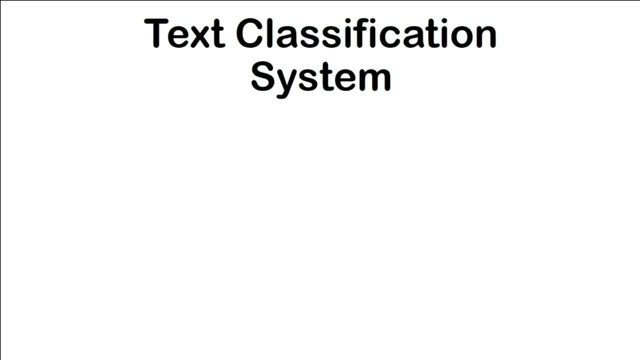 understand some basic concepts regarding machine learning: machine learning in natural language processing, but it in natural language processing, but it in natural language processing. but it will help you in further machine learning, will help you in further machine learning, will help you in further machine learning. okay, because you will learn what is a. 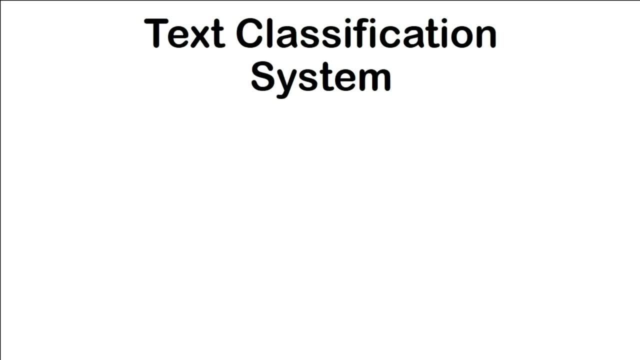 okay, because you will learn what is a. okay, because you will learn what is a model. okay, how to train a model or how model. okay, how to train a model or how model. okay, how to train a model or how to test a model: okay, so you will learn. 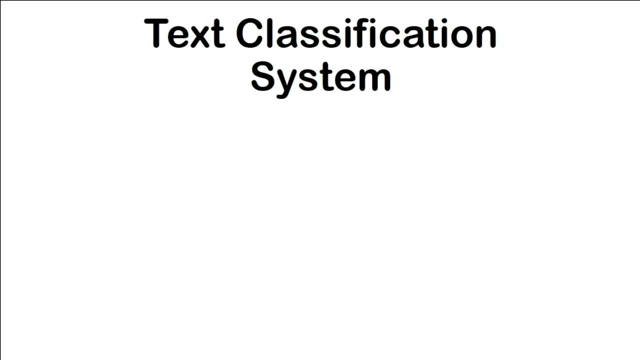 to test a model. okay, so you will learn to test a model. okay, so you will learn so many basic concepts regarding machine. so many basic concepts regarding machine. so many basic concepts regarding machine. learning in this text class, during the learning in this text class. during the learning in this text class, during the development of our text classification. 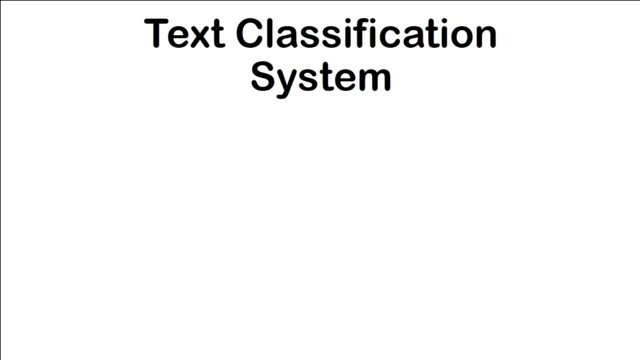 development of our text classification. development of our text classification system. okay, and the next question is how system? okay, and the next question is how system? okay, and the next question is how we will develop our own text. we will develop our own text. we will develop our own text classification system, so we will use a. 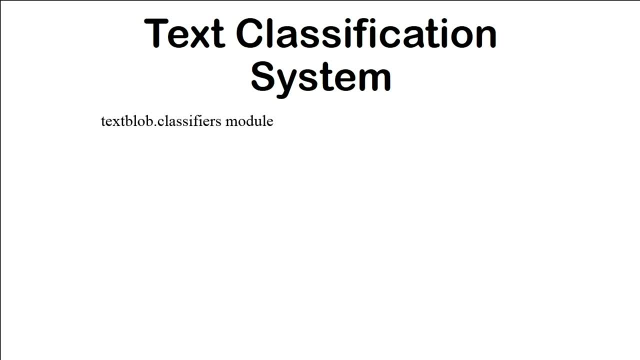 classification system. so we will use a classification system. so we will use a text block dot classifier module and it text block dot classifier module and it text block dot classifier module and it will really help us to develop our own, will really help us to develop our own. 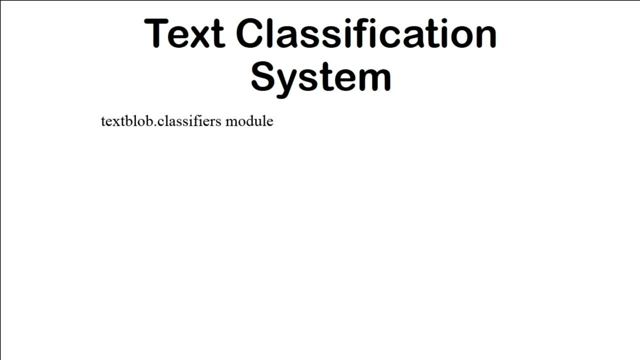 will really help us to develop our own text classification system. okay, text classification system. okay, text classification system. okay. and now you are thinking that what is a? and now you are thinking that what is a? and now you are thinking that what is a model, because i have used this words in. 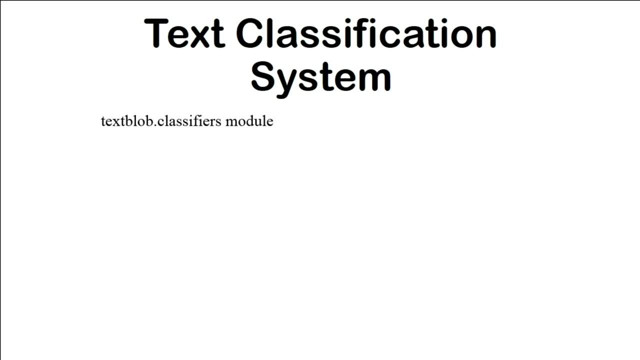 model, because i have used this words in model, because i have used this words in the beginning of the lecture. so what is the beginning of the lecture? so what is the beginning of the lecture? so what is a model? so a model is basically a file. a model, so a model is basically a file. 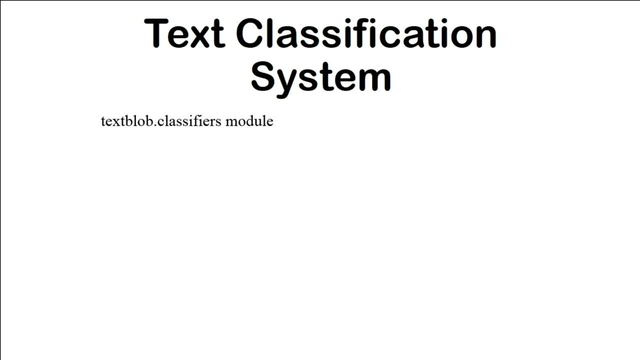 a model, so a model is basically a file. okay, so that will help us to recognize. okay, so that will help us to recognize. okay, so that will help us to recognize certain patterns. okay, after uh training certain patterns. okay, after uh training certain patterns. okay, after uh training it, okay. so, in simple words, uh, if i say 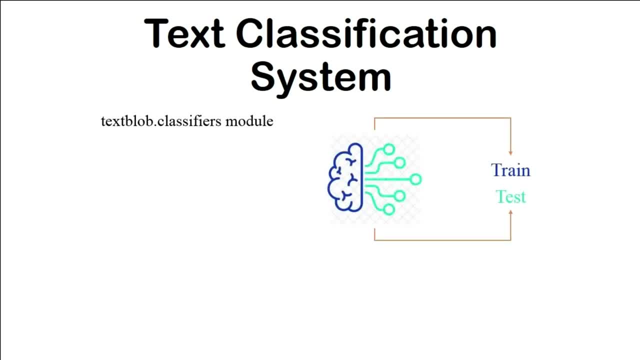 it okay. so in simple words, uh, if i say it okay, so in simple words, uh, if i say: a model is just like a brain, okay, so we, a model is just like a brain, okay, so we, a model is just like a brain. okay. so we first train the brain and then we test. 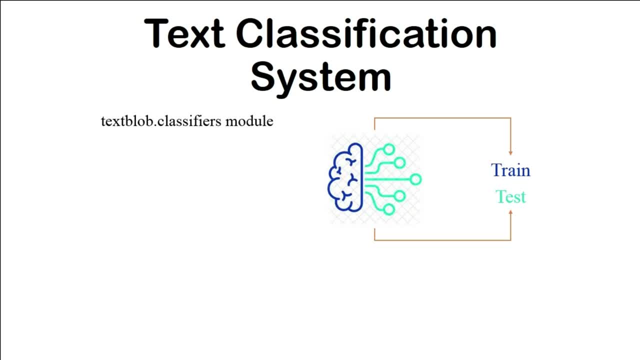 first train the brain and then we test. first train the brain and then we test our brain. okay, so at level zero, our, our brain. okay, so at level zero, our, our brain. okay, so at level zero, our brain, or our model, is just like a brain, or our model is just like a. 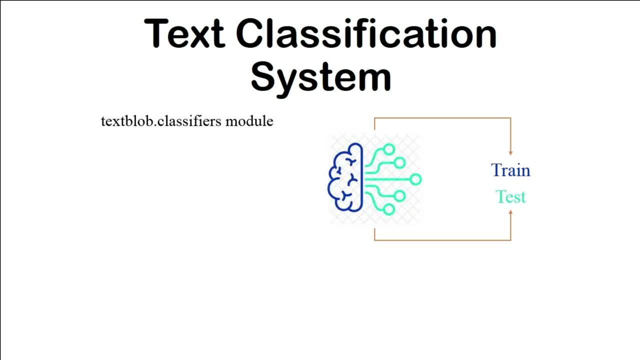 brain, or our model, is just like a brain of a child- okay, and it knows brain of a child- okay, and it knows brain of a child- okay, and it knows nothing about anything- okay. it knows nothing about anything- okay, it knows nothing about anything- okay, it knows nothing how to perform operations- okay. 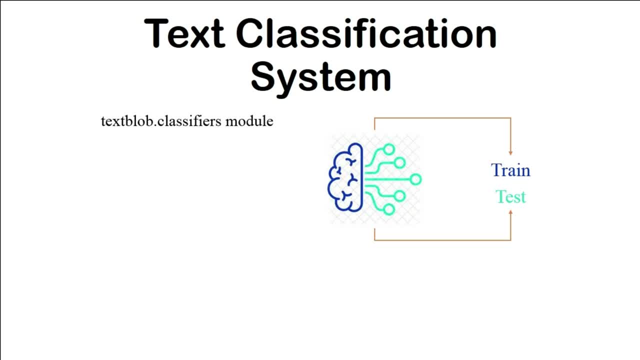 nothing. how to perform operations- okay, nothing. how to perform operations- okay, and how to check for certain conditions and how to check for certain conditions and how to check for certain conditions- okay, and everything else. so, first of all, okay and everything else. so, first of all, okay and everything else. so, first of all, we train this model by providing data. 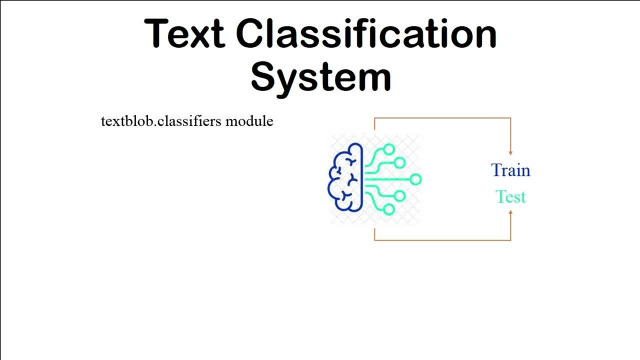 we train this model by providing data. we train this model by providing data and providing answers okay, for example. and providing answers okay, for example. and providing answers okay, for example, we will provide a sentence and our model. we will provide a sentence and our model will tell us whether this sentence is. 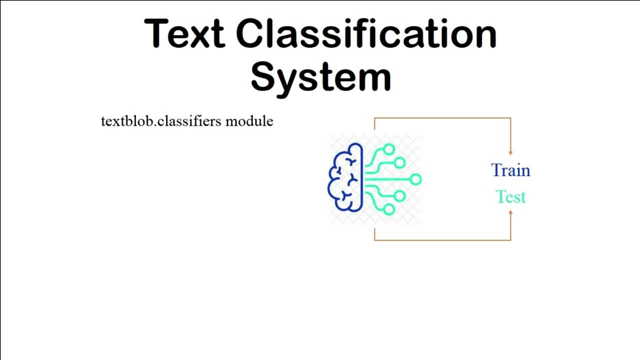 will tell us whether this sentence is, will tell us whether this sentence is positive or negative. okay, like sentiment positive or negative. okay, like sentiment positive or negative. okay, like sentiment analysis: we have done before, so we will analysis. we have done before, so we will analysis. we have done before, so we will develop our own custom sentiment analysis. 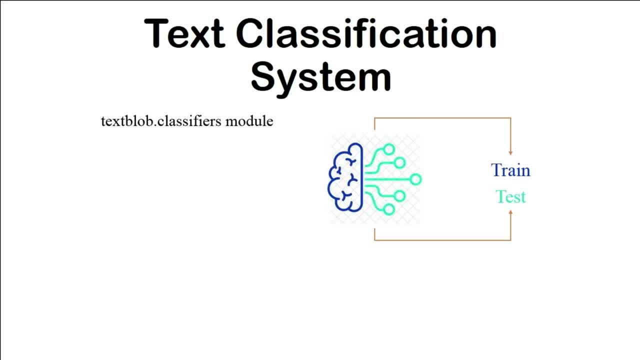 develop our own custom sentiment analysis, develop our own custom sentiment analysis system. okay so, first of all in training system. okay so, first of all in training system. okay so, first of all in training section. we will provide sentences and we section, we will provide sentences and we section: we will provide sentences and we will also provide answers. okay, so we will. 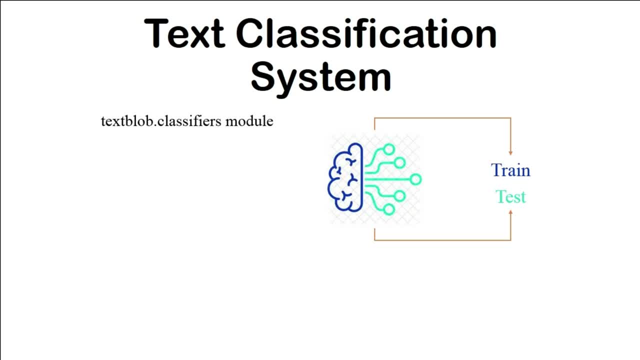 will also provide answers. okay, so we will will also provide answers. okay, so we will write a sentence and we and we will write a sentence and we and we will write a sentence and we and we will tell that this sentence is positive. then, tell that this sentence is positive, then. 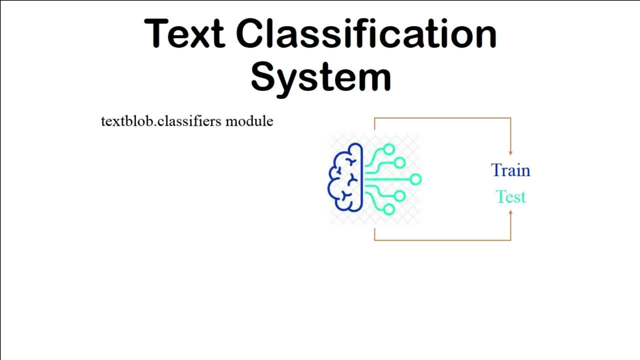 tell that this sentence is positive, then we will provide an other sentence and we will provide an other sentence and we will provide an other sentence and we will say we will say we will say this sentence is negative. the more we this sentence is negative, the more we. 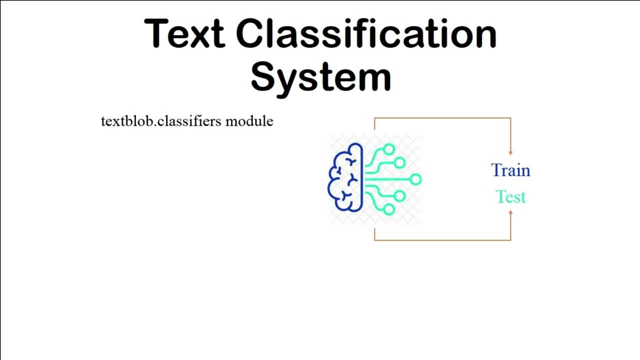 this sentence is negative. the more we will provide data to the system, the more will provide data to the system. the more will provide data to the system, the more we will make our system accurate. okay, so we will make our system accurate. okay, so, we will make our system accurate. okay, so i hope you have understood what is. 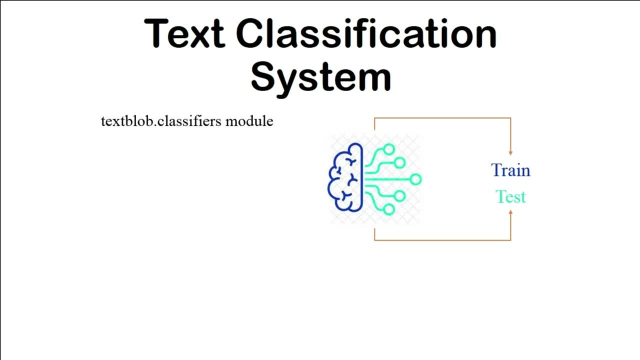 i hope you have understood what is. i hope you have understood what is training, and then we will test it. so we training, and then we will test it. so we training, and then we will test it. so we, then we will, then we will, then we will ask a user to enter any sentence. okay, 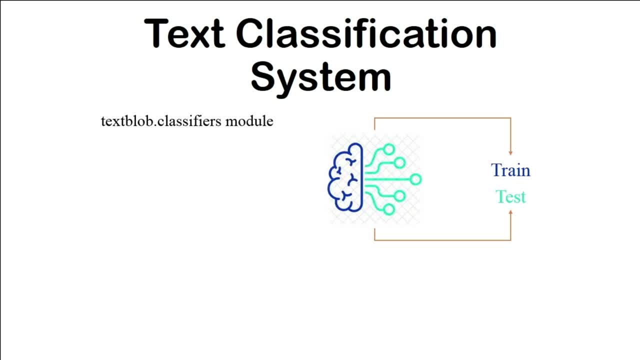 ask a user to enter any sentence. okay, ask a user to enter any sentence. okay, and we will tell that whether your and we will tell that whether your and we will tell that whether your sentence is positive or negative. okay so, sentence is positive or negative, okay, so. 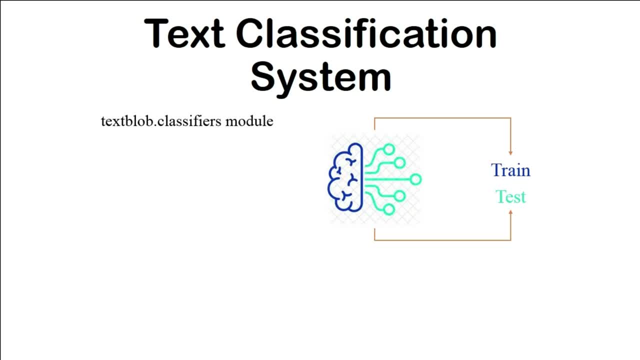 sentence is positive or negative. okay, so this is how a model works. so it is like, this is how a model works. so it is like this is how a model works. so it is like an artificial brand. okay, and it actually an artificial brand. okay, and it actually. 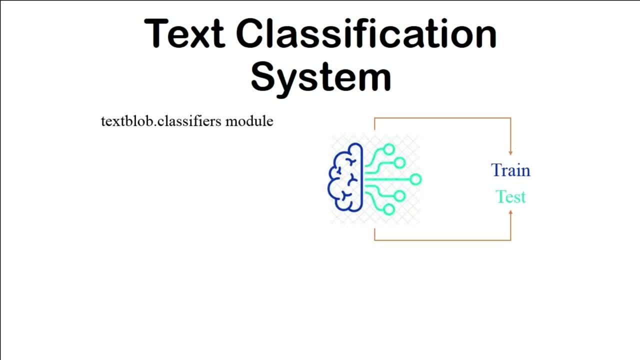 an artificial brand, okay, and it actually makes decisions and we do not need to makes decisions. and we do not need to makes decisions and we do not need to uh explicitly tell uh the system, whether uh explicitly tell uh the system, whether uh explicitly tell uh the system whether this is positive or whether this is. 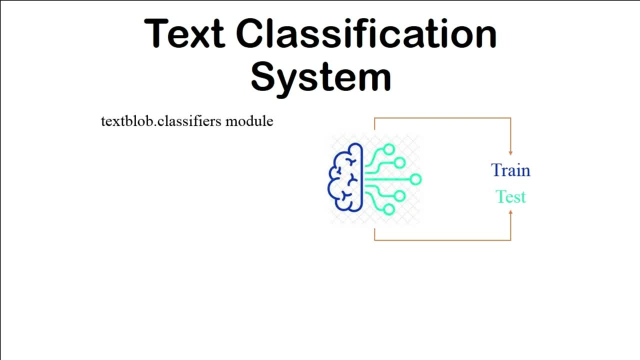 this is positive or whether this is negative. all the decisions are made by machine. this model itself, okay. so i hope you have understood what is a model, and now the next question is- and that is what you will learn- so you will basically learn how to load data from files, okay, and you will also learn how to create a model. then how? 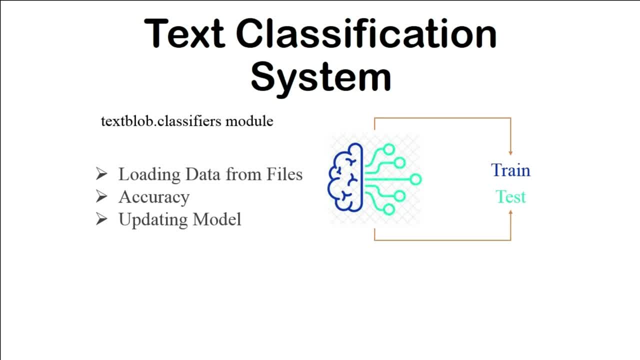 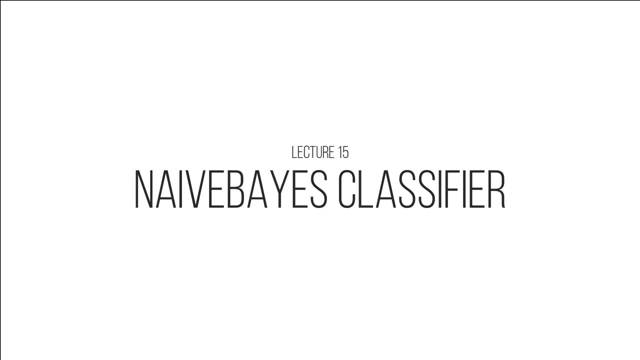 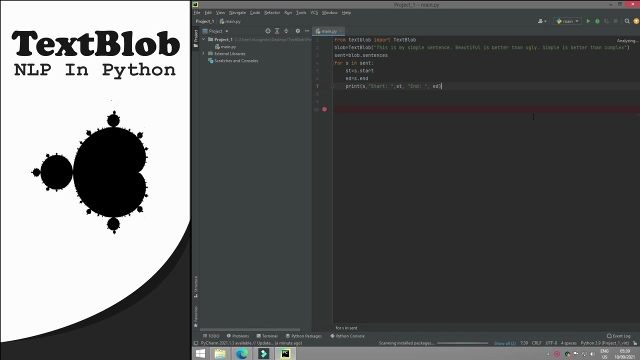 to check the accuracy of the model. okay, and you will also learn how to update a model. so i hope you have understood the basic concept regarding our text classification system and from the next tutorial, we will actually start the development of our own text classification system. in this tutorial, we will start the development of our own text classification system and in this, 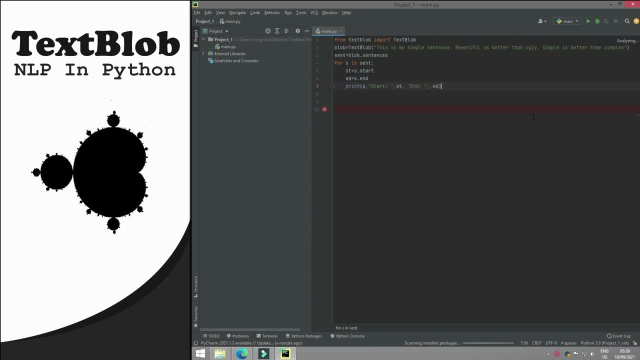 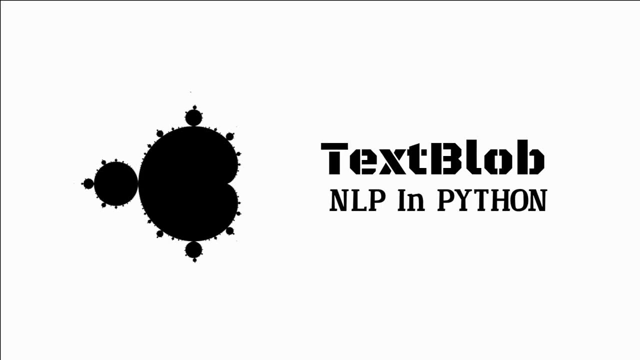 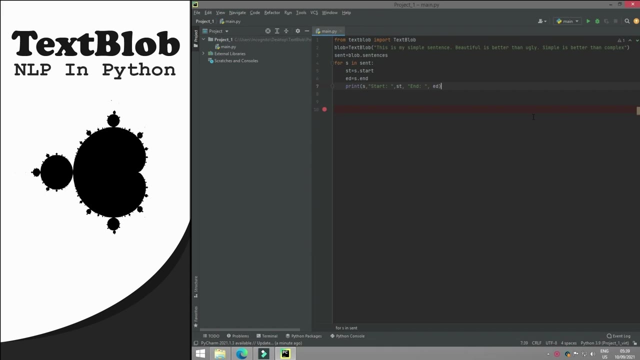 tutorial. we will see how to load data, okay, and then we will see how to create a classifier, so let's begin the lecture. so, so, first of all, we need to create a classifier, okay. so in this case, i will use a built-in text block classifier, and that is nevbay classifier. and now you are thinking that, what is a nevbay? 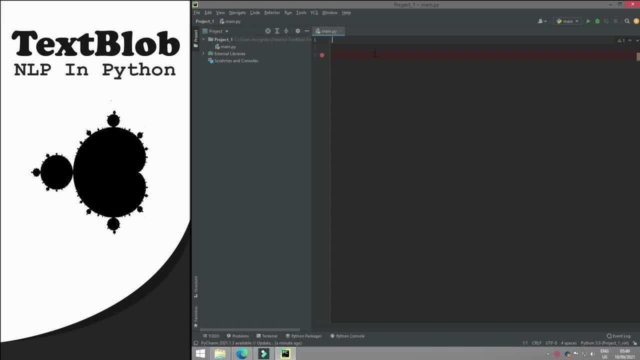 classifier. so it is basically a probabilistic machine learning model that is based on bayes theorem. so if you know, know base theorem, then well and good, but if you don't know base theorem, then i will not explain it because i don't want to make you confused. okay, i'm assuming that you are absolute beginner, having 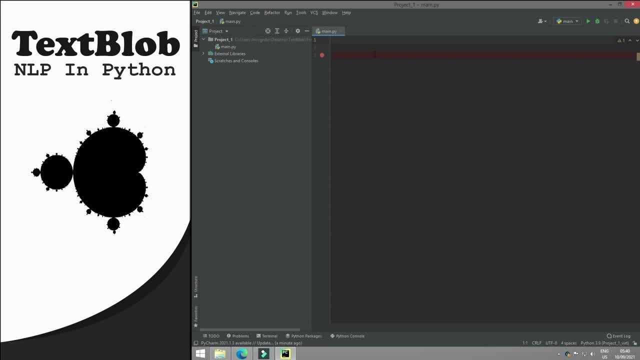 no knowledge of machine learning. okay, and that's why i will not go in theorems or anything else. i will make accepted a course on all these basic concepts regarding machine learning and i will explain all of these theorems there. okay, but i will not explain base theorem here, okay. 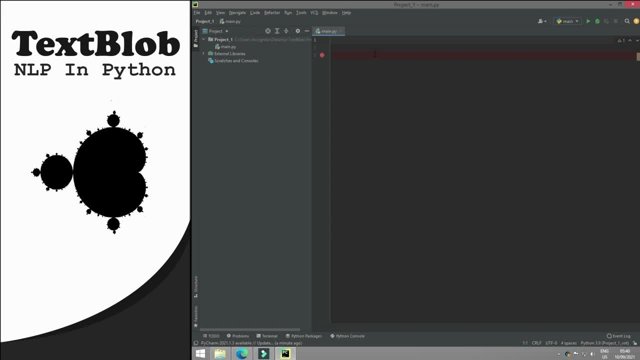 because this will make you, uh, confused, so i will just directly go to practical work. so first of all, we need to import our model or our classifier. okay, so, just right here. from text blrb, from text blob: dot classifier: import naiv nav back classifier. okay, so the above one. okay, so now we have imported. 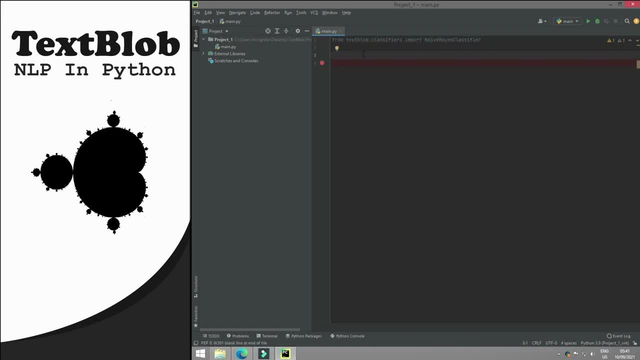 our nav back classifier. okay, and now we will create a model. so, for example, i will call it like: model is equals to nav and a, i, v, e, nav or sorry, nav back classifier. and here, inside this classifier, we need to pass a data set. okay, so we need to train this model. okay, so that it will make a 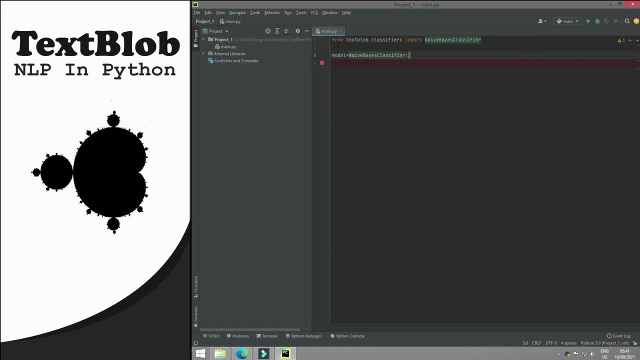 or accurate decision. so now we need to log out our data. so let me mention here creating class C, CNA, double si fi er, creating a classifier, and now we need to load our data and or a di? ng loading the ATA, loading data, okay, so we need to data set. okay, and why we need to data set our 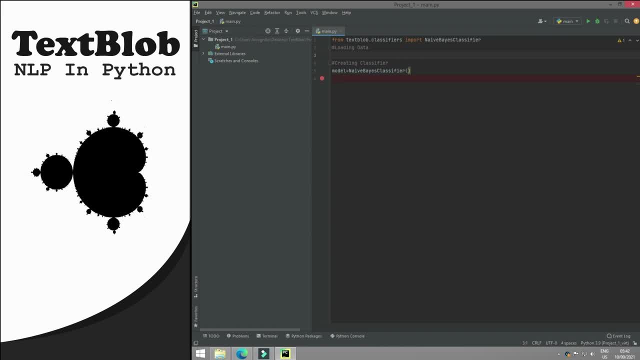 first data set will be our training data set, okay, and it will train our model, okay. and then we need a second data set and that will be our testing data set and with the help of that testing data set we will test our model. okay. so I have just type here: TRI and train, okay, you can call anything, okay. so it's just. 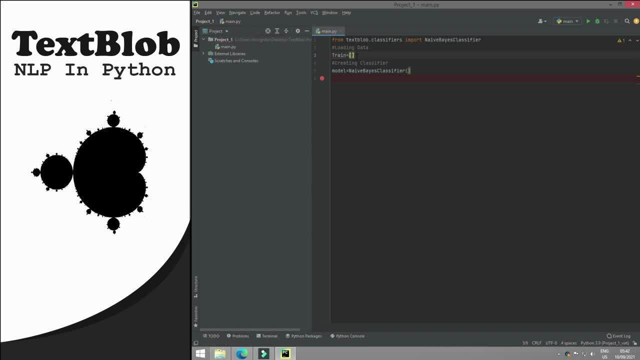 a variable name and you must must make sure that your data should be in form of a list, okay. so, for example, inside this list, I will pass my sentence like I love send W a sandwich, okay, and then this sentence will be P or S positive, okay, so. 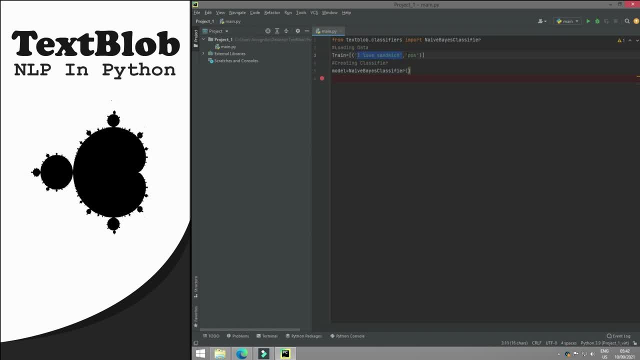 this is my one, this is my sentence, okay, and this is my answer, okay, and then put both of these things in these rounded brackets and now let's create a second sentence and in this case I will make it a negative. I do not like what. I do not like burgers, or yeah, view RGR burgers. okay, and just make it. 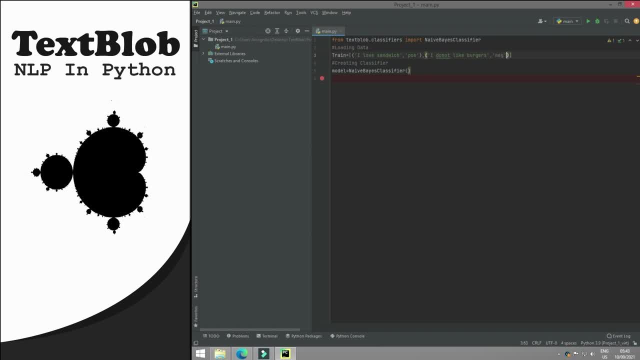 negative and eg negative. okay, so this is, this is how you can actually create a training, a data set. okay, and now we need to create our testing data set. just just right here, test is equals to, and your testing that I should. data set should be of type list as well. okay, put rounded brackets. 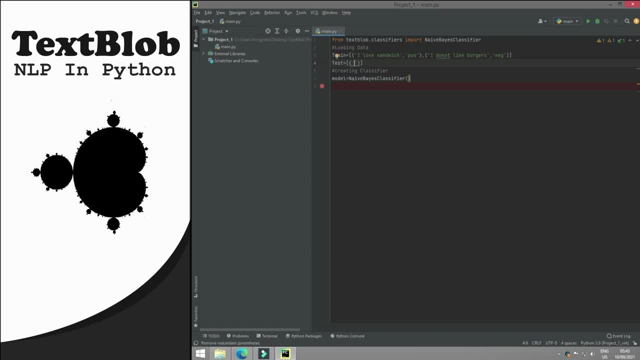 here and just pass your sentence. for example, my testing. I like birds. okay, and you are thinking that why I am writing here positive. okay, let me explain it to you later. okay, and I will write here: I, I had, okay, I had what I know double la, la, la, la, la la la lolly pops. okay, and I will make this sentence negative. okay, 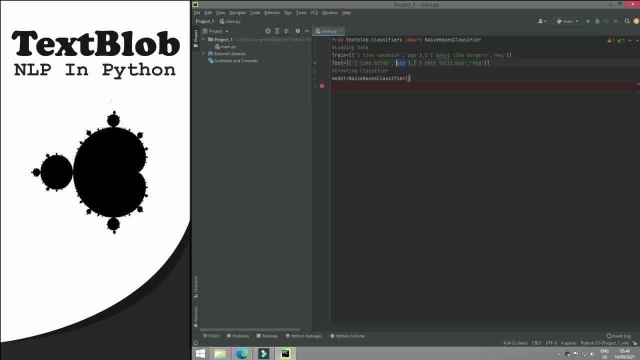 now you are thinking that why I'm writing here positive and why I am writing here negative, it is a testing list. okay, so why I need answers? because, with the help of this testing list, we will check the accuracy of our model. okay, so we we will actually pass this testing list when we want to check the 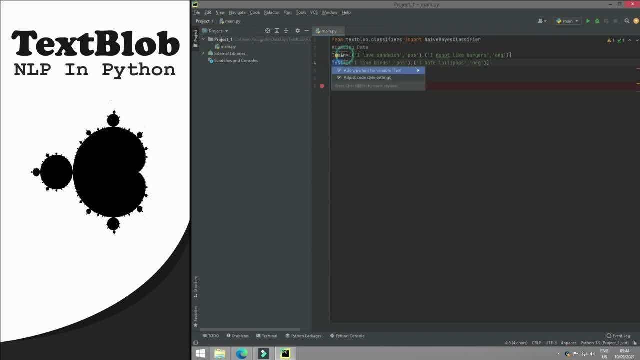 accuracy of our model. otherwise we will try our model, okay, with the help of this list, and then we will get input from users, okay, and it will tell whether your sentence is positive or negative. but when we want to test the accuracy of our model, then we pass this test, okay, and it will make a decision based on these lines and 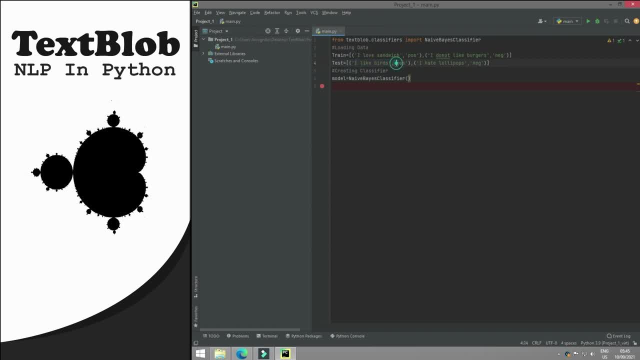 then it will compare its decision with the answer which we have written here and it will tell whether I am accurate or not, or whether I am 80% accurate or 90% accurate or 100% accurate. so I have written these two sentences here. so I have mentioned in the previous lecture: the more you. 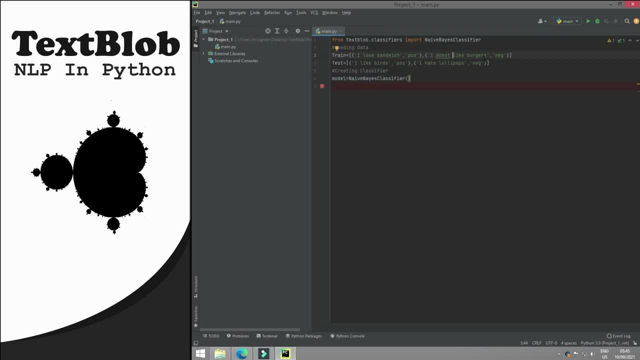 will provide data to the model, the more it will learn new things and the more it will become accurate. okay, so I have copied two data sets- the training and the testing data sets- and I will paste it here. okay, so this is my training data set. okay, and this is my testing data. so just remove it and just 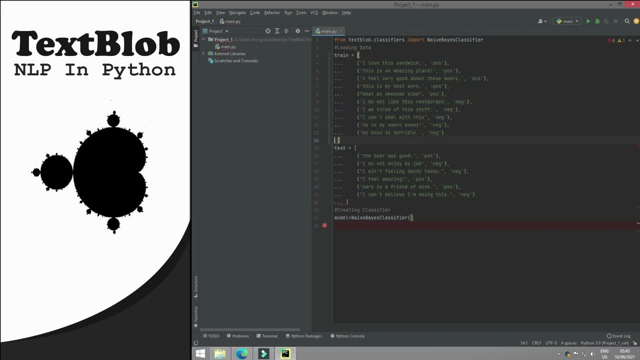 remove these lines here, okay, and yes, everything else is good. okay, so this is my training data set. okay, yeah, it is a lace and it has the sentence. okay, yeah, it's a piece of text, but I have written here these two sentences here and inside this sentence right here, it has several sentences and inside these sentences I have written the answer. 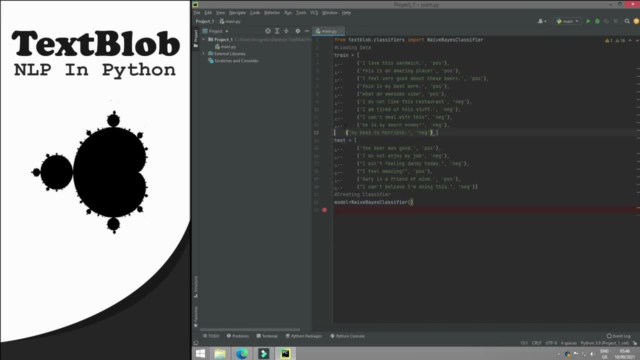 of these sentences. okay, and now this is my testing list. okay, so I have these sentences and I have written the answer of these sentences. okay, so it's good, it's good, so let me remove these things, okay. okay, so I have rearranged my training data set and testing data set, and now we will pass our decision. 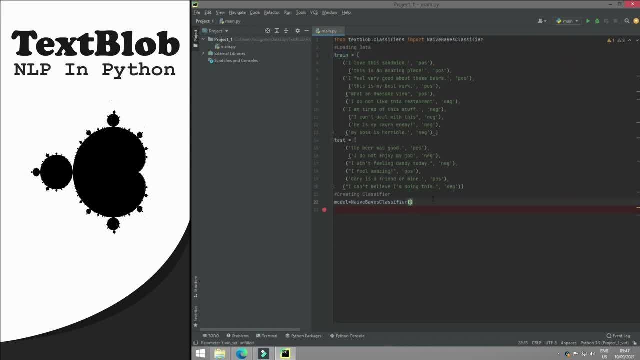 this training that i set to this model. so, just right here, t-r-a-i-n train, okay, and now our model will train itself whenever we run it. okay, so, if i run it, everything is processing and you will see nothing. okay, so you will see nothing because we are printing nothing. okay, okay, so it has finished. 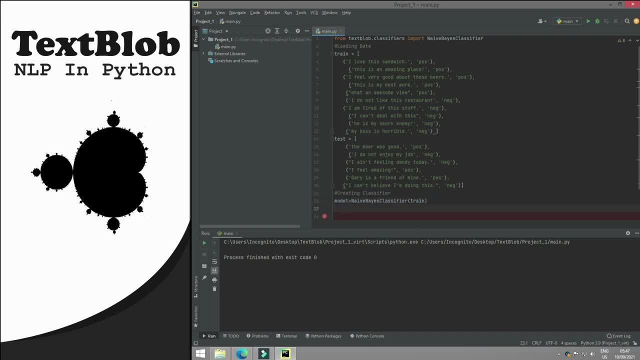 okay, so now. now, if i say print, print, m-o-d-e-l, let's see what we will get. okay, so all right. it is saying that our classifier this never classifier and trend on 10 instances. so these are my instances. okay, so one, two, three, four, five, six, seven, eight, nine and ten. okay, so 10. 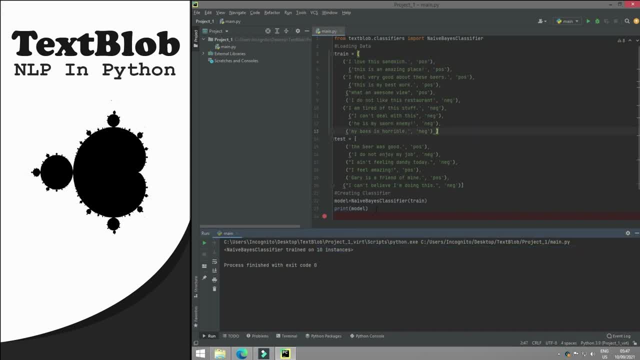 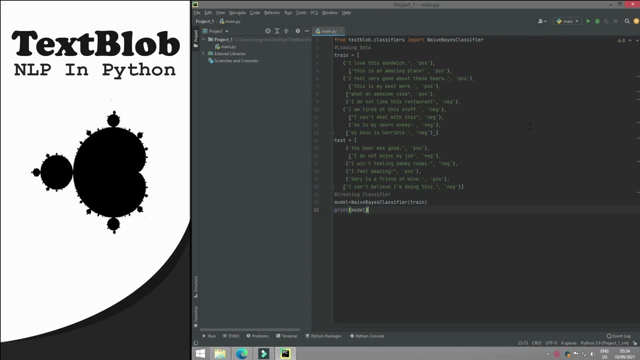 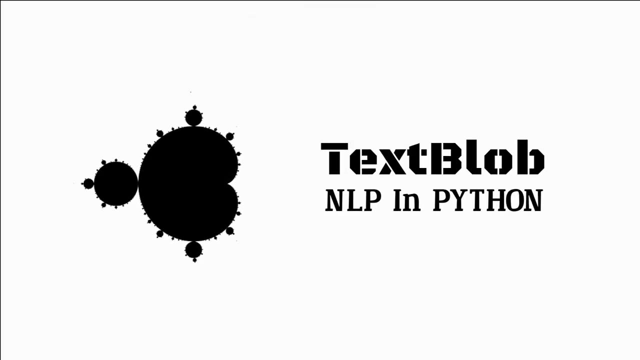 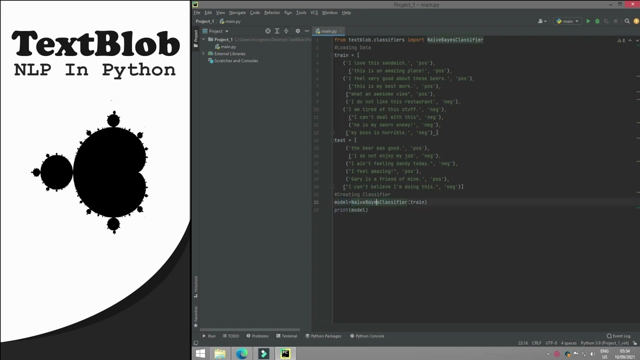 instances. so awesome, you have trend your model. so in this tutorial we will see how to classify text using our own classifier. so let's begin the lecture. okay, so previously we have created our model, okay, using this nav back classifier, and then we are passing our data set. okay, and now we will see how our model is acting. 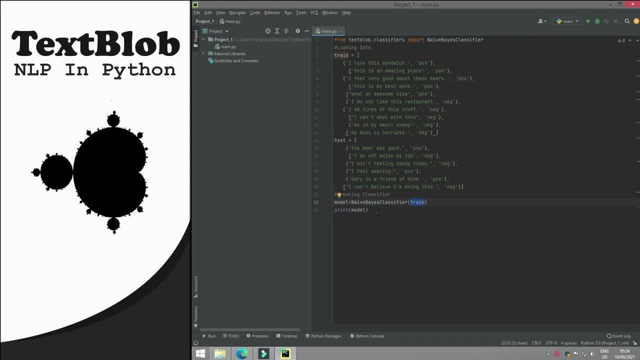 okay, so let's see how our model is acting. okay, so, let's see how our model is acting. okay, so, whether our model is accurate or not. okay, so it's very simple. for example, uh, i will uh pass a sentence to my model, okay, and i will print the result in this result variable. okay, so, just right here. model. 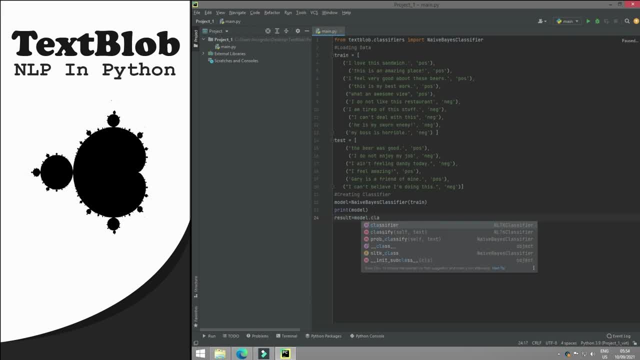 dot. uh, what i say: classify, model dot. classify. okay, we need to classify our text. and here i will pass my sentence, for example: uh, this is an m-a-z-i-n-g classifier. okay, so we are going to classify our text. uh, this is an m-a-z-i-n-g classifier. okay, so, this is an m-a-z-i-n-g classifier. okay, so we need to classify. 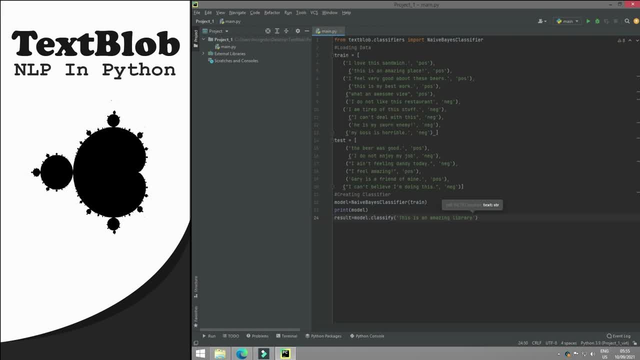 amazing and I be RA. alright, this is an amazing library and we want to check whether our this sentence is positive or negative. okay, so just print of a result. okay, re stl t result. and we know very well this sentence is positive. so let's see whether our model is accurate or not. and yes, of course this sentence is. 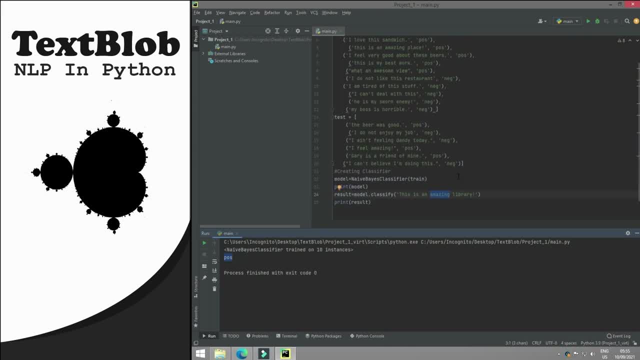 positive. this means that our model is quite good. okay, so, and let's try another sentence. okay, or you can actually get input from user as well. for example, I will get input from user or can input, and I will say: inter your se NT and see: enter your sentence. okay, and I will. instead of passing your sentence, I will 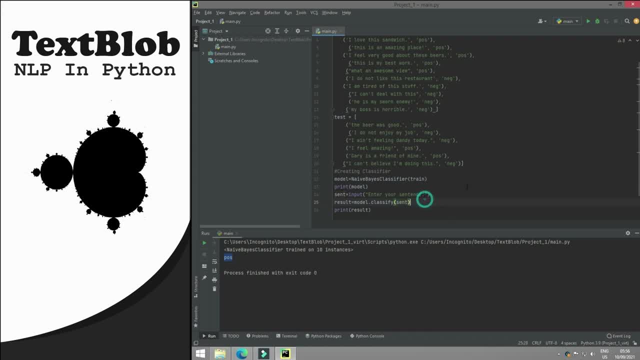 pass my SC and sent you variable. and now let's run it. okay, enter your sentence. for example, I had, or I do not, do not like a derpy, alias apples, okay, and it should print negative because it's a negative sentence. so let's run it. and yeah, here is my. 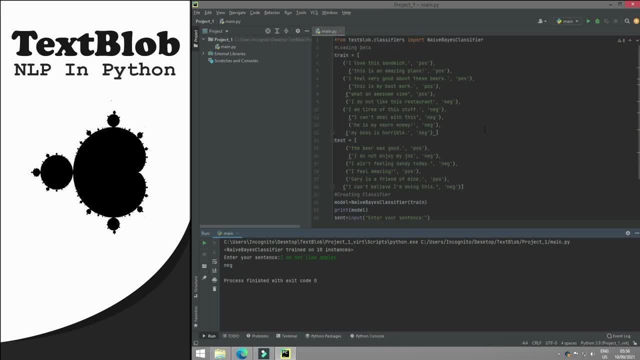 answer and that is negative. so this means that our model is quite good, okay, and the more you will provide the data, the more it will become accurate. so you can actually check the probability or the confidence level as well. for example, let's here I will say: like what you are, like probability p or. 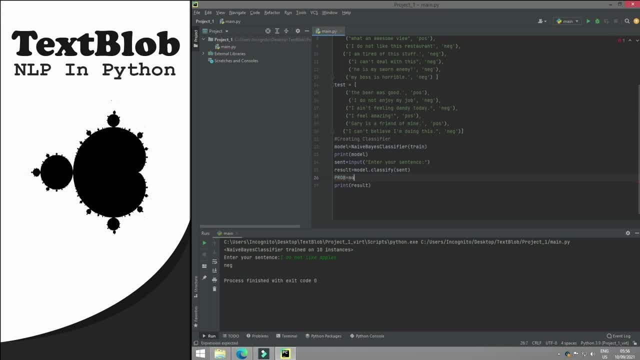 ob prop is equals to m od el model dot prop classifier. okay, so prop classifier, and here I will pass my sentence: SE and decent variable- okay, and I will type my sentence: scnt sent variable. okay, and here I have a sentence. okay, and then, let's OK, I want to check the probability of my this sentence. 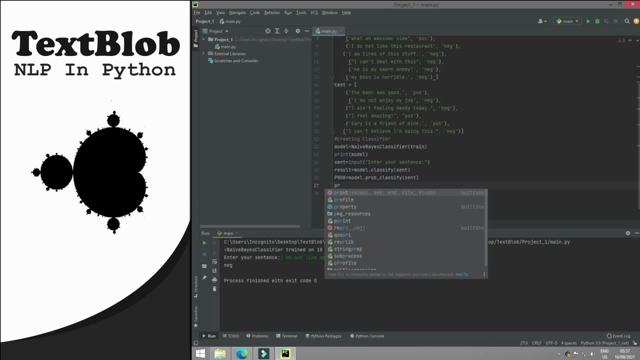 OK, and now I need to print P-R-I-N-T. print prob dot prob OK. so what is prob dot prob? So basically we are classifying our, or we are testing the probability, and this probability class basically returns two things or two instances. 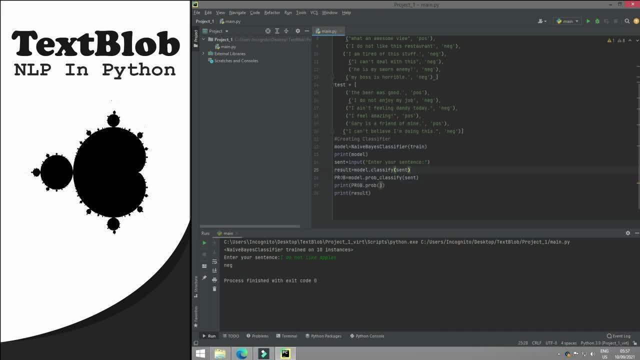 OK, the positive probability and the negative probability. And in this variable now we have the positive probability and negative probability. And to check the whether, to check our positive probability, OK, we will pass here P-O-S positive. OK, so it will print our positive probability. 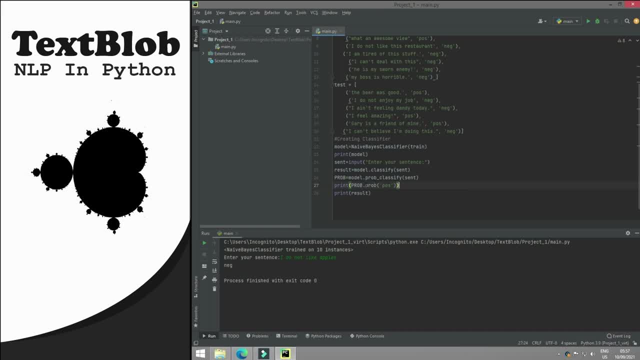 And if I pass here negative, it will print our negative probability and how we can access that probability. For this purpose we are using This prob function. OK, so for just remember, put to this prob classify and pass your sentence, OK, and then through that variable we can access this prob class or this prob function. 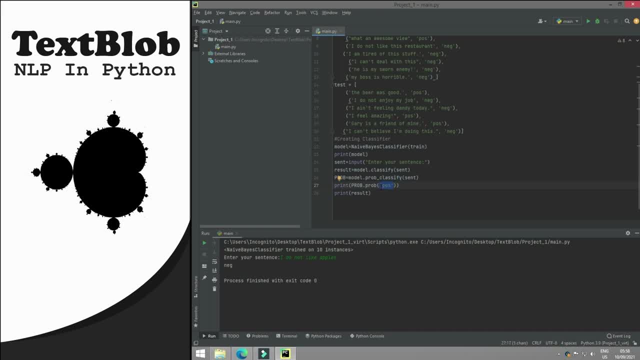 And inside that function just pass whether you want to check the positive probability or you want to check for the negative probability. OK, so let's try both of them. OK, so print P-R-O-B prob dot And then I will pass. negative energy negative. 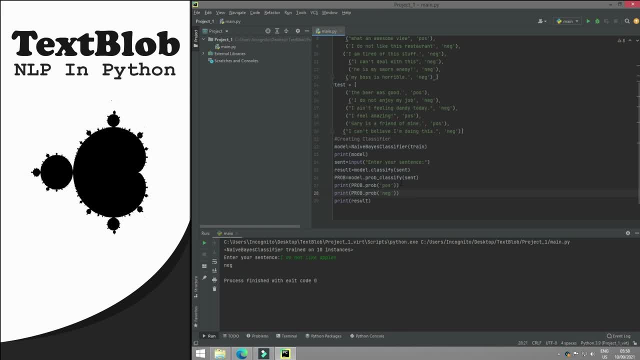 OK, and these values are between zero and one, So let's run it And just pass our sentence. For example, this is an amazing, amazing B-Double-O-K book. OK, so just enter. OK, so this is my positive probability. 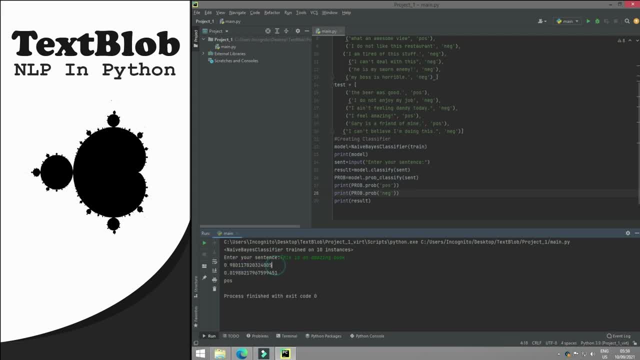 And this is my negative probability. OK, so zero point nine eight is my positive probability And that's why it is showing that this sentence is positive. OK, and this is my zero. point zero nine is my negative probability And that's why. 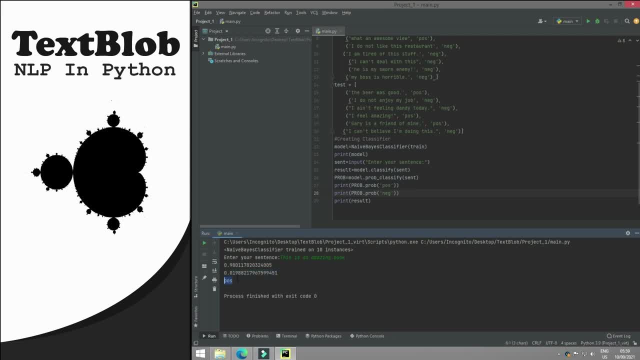 Yeah, of course it is positive, still positive, because our negative probability is much, much, much smaller than our positive probability. OK, so this is how you can check for the probability And you can Classify your sentences. OK, so awesome. 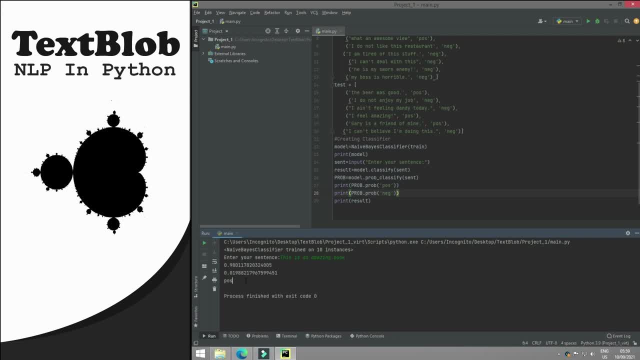 You have made your own sentiment analysis system. OK, so you can convert these probabilities to percentage as well. For example, I will assign a variable to this line, OK, and then I will multiply that variable with one hundred. OK, and to avoid these long numbers, 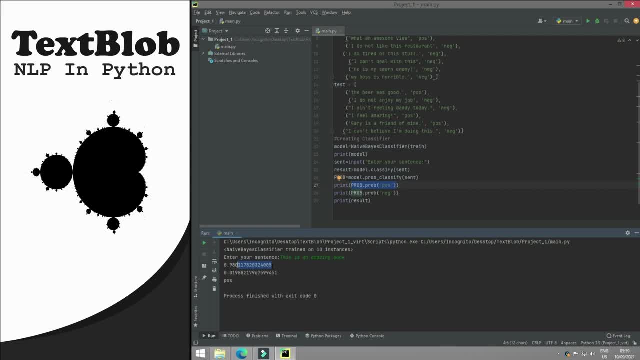 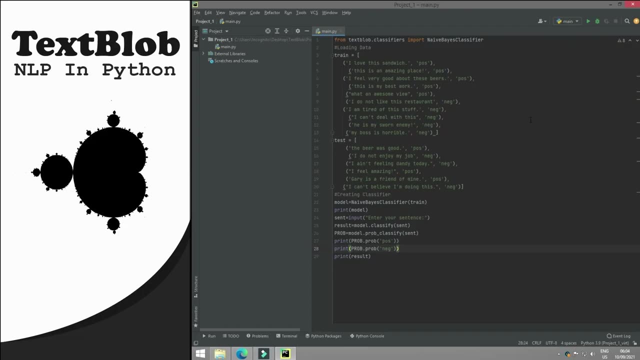 OK, I will convert that result into int. OK, so we have done everything previously, So you can use this, The same logic, to convert this value to percentage. OK, and you can print the probability in percentage for a better output. OK, so in this tutorial we will see how to classify the sentence which we have passed to our text about class. 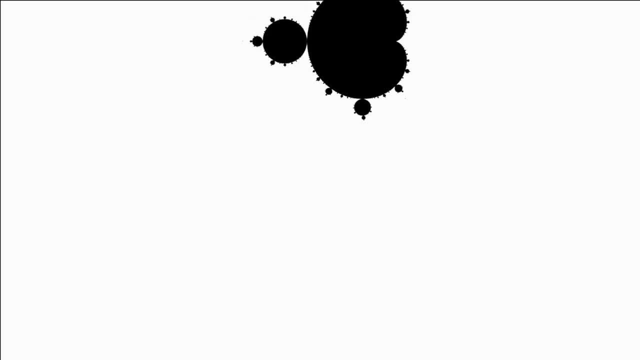 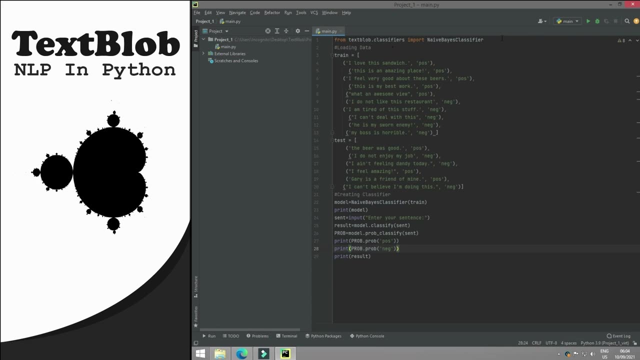 So let's begin the lecture. First of all, let's create our text. OK, so I will call it like my blob is equals to txt text, be a lobby blob, OK, and I need to import it. So from text blob I import text blob. 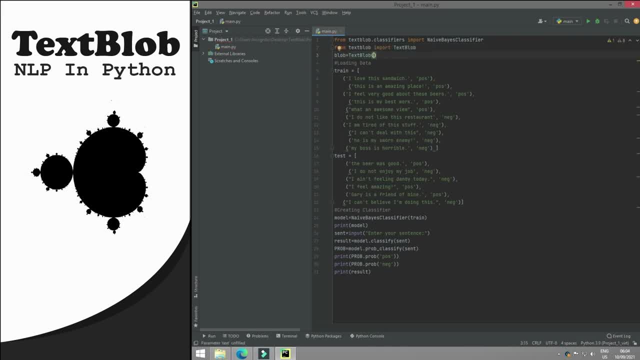 OK, so this is my text, blob class. And now inside this class, let's pass a sentence: OK. so for example, I love be a double n, a, b, And if I love banana, OK, but I had, or I do not like adobe alias apples. 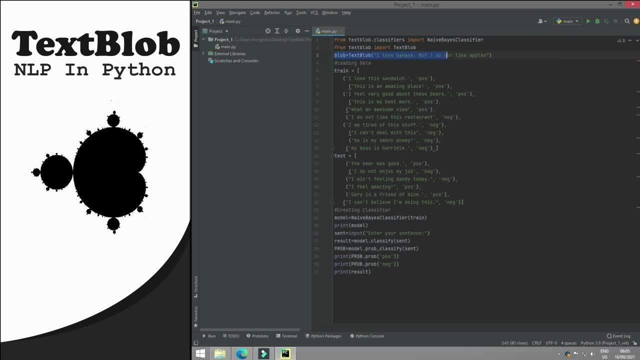 OK, so this is my blob text blob, And now I need to classify this blob using our this model. OK, so just shift this sentence down. OK, just cut it and just put This sentence right here. OK, and now I need to use my this model to classify this text. 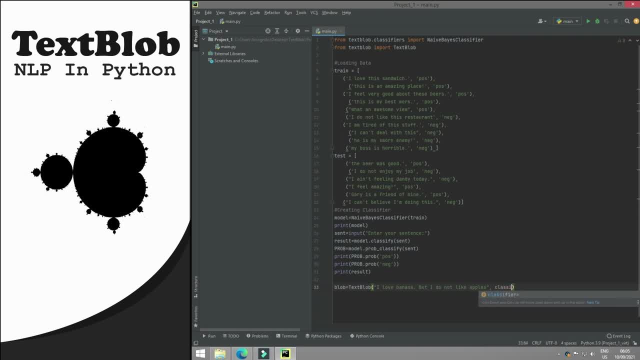 OK. so just right here, See, and at the balance, I classifier is equals to, and then pass your name of the classifier, And in this case, my classifier is this: model OK. so just press your emoji e and model OK. and now I need to classify this text. 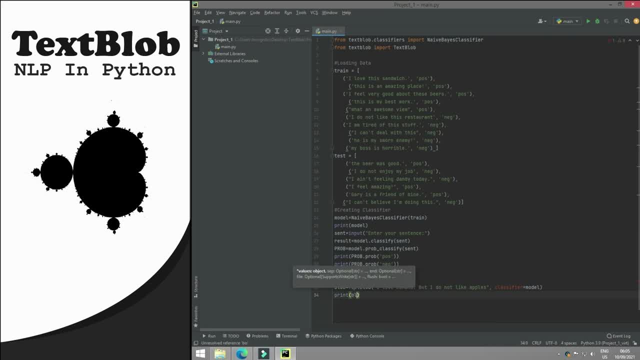 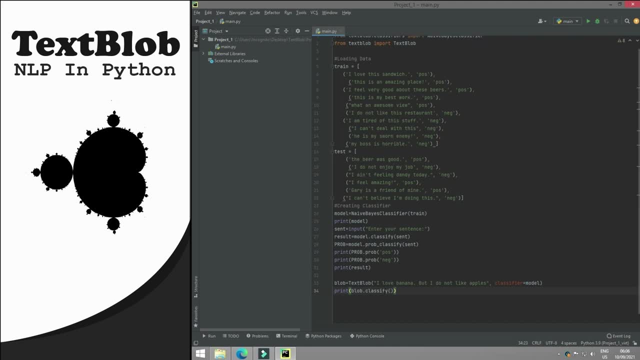 So just right here below the end of the blob dot, classify OK, And I need to To print it. So what are you expecting? Will it return positive or negative? Because my this sentence is positive but my this sentence is negative. 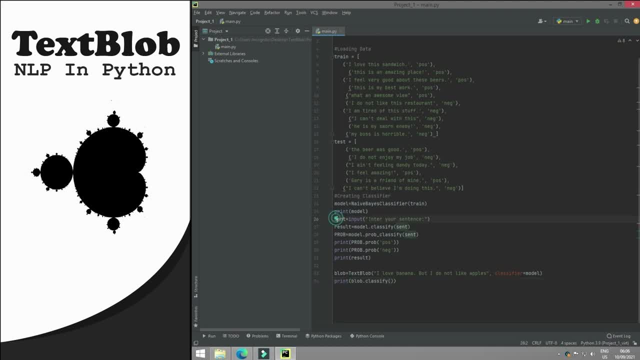 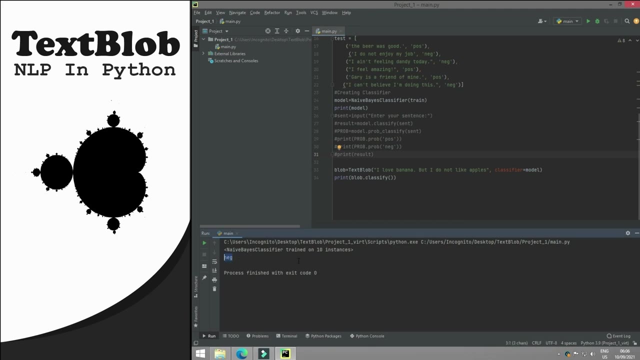 But before I run it, let's comment these sentences. OK, so let's comment everything here, OK, OK, so that we will get our output. OK, so, yeah, I want this sentence is negative. OK, so how And why our this sentence is negative. 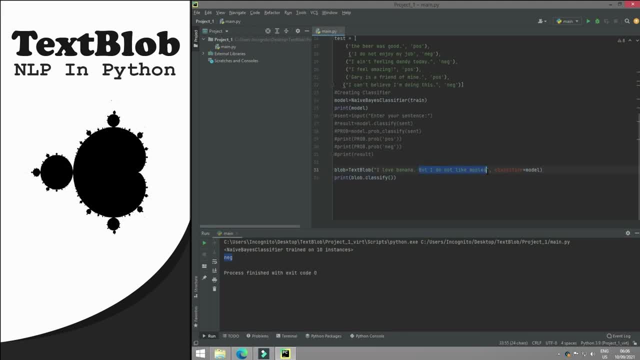 This is because the negativity of this sentence is higher than the positivity of this sentence OK, and that's why we are getting negative. So one of the major advantage of this text blob is that we can actually check or we can classify our sentences separately. 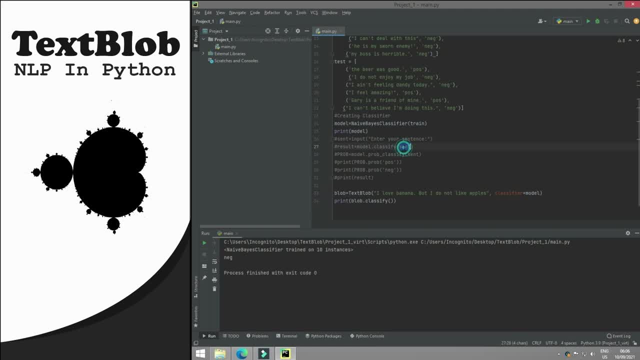 So if I pass my sentence here directly into plus five, we cannot test them. OK. so even if I use Or write a paragraph, OK, or if I pass my whole paragraph to this classify function, OK, it will classify the whole paragraph, not the separate sentences of the of this paragraph. 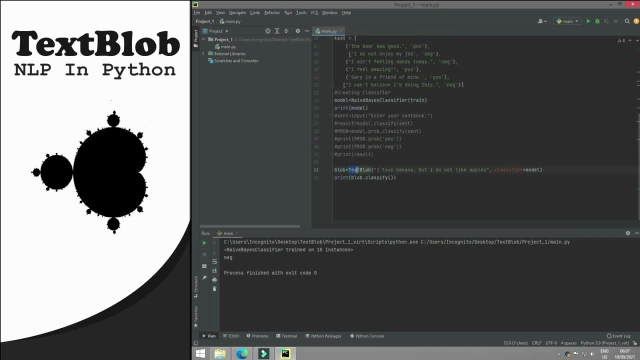 OK, but using the text blob we can loop through all these sentences, OK, and then we can check or we can classify that these sentences separately. So let's loop through these sentences. So I will write here, for as the end is in. 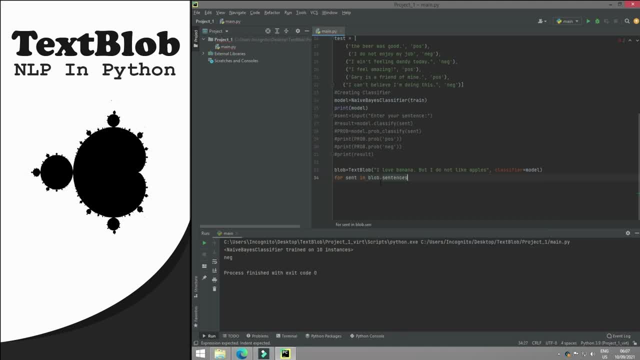 Blob dot sentences: OK. so I will loop through these sentences, OK, and first of all I will print that sentence and then I will tell the user whether this sentence is positive or negative. OK, so just try to send dots classify. 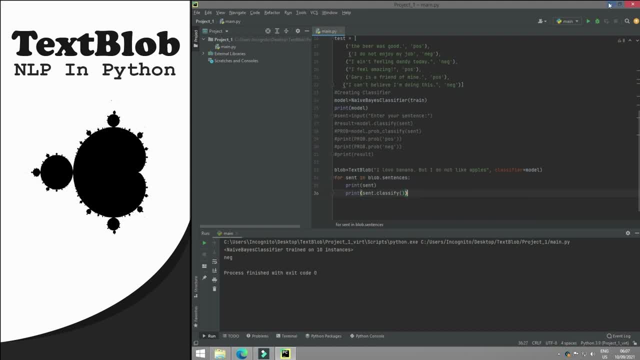 OK, and now I need to classify this sentence. OK, so if I run it. OK. so my I love banana is positive, It's cool, And I do not like apples. OK, so my I love banana is positive, It's cool, And I do not like apples. 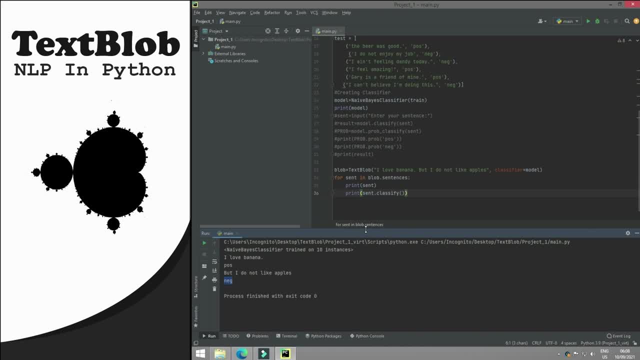 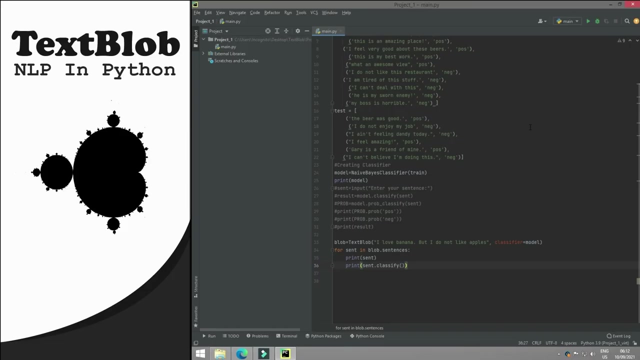 is negative: OK. so this is one of the major advantage of this approach: using this text blob class, or can then passing our work of sentences or even a paragraph here and then looping through different sentences and then classifying each sentence separately. So this is one of the major advantage of this approach. 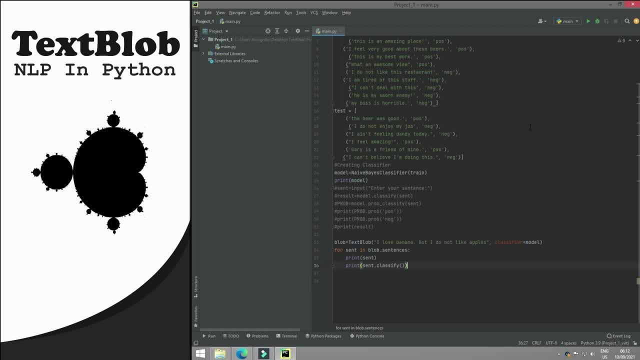 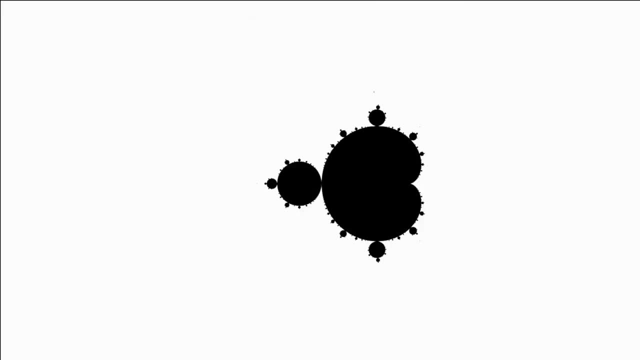 Woo-hoo. this is one of the major advantages of this approach. in this tutorial, we will see how to check the accuracy of our model and then how to update it. to update a model, so let's begin the lecture. okay, so first of all, let's. 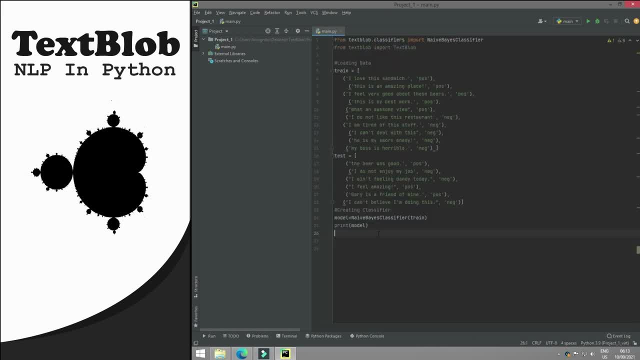 remove these things. okay, so just remove it. and now I hope that you are now thinking that why we have created this text data set. okay, let me answer you this question now. we will use now this data set to check the accuracy of our model. okay, so how we can check the accuracy of our model? so it's very, very. 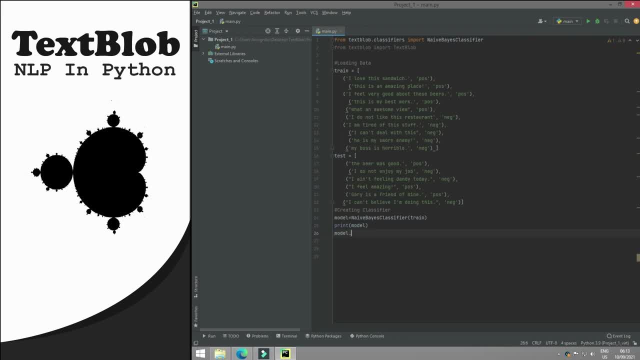 simple as you just need to write here: model dot a double-c- you accuracy- okay, and inside this accuracy we need to pass our this test data set. okay, so just passed. pass it here. te st test: okay, so it will return our value and integer value or not an integer value, a float value- okay, and we. 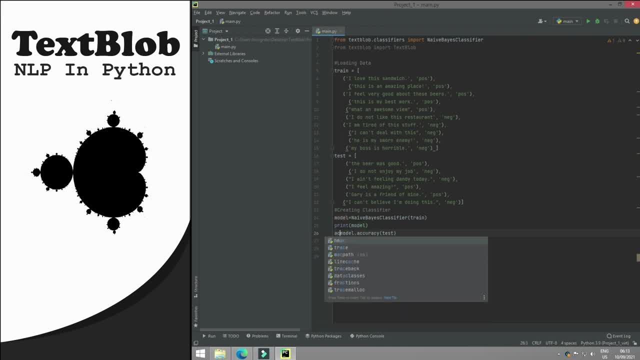 will save that value inside this, like I will call it inside this variable, okay, and now I will print this variable, okay. so, but I think before running the application, let's convert this value to percentage, okay, so that we will get a better output. so I will call: a double C is equals to a double C multiplied by. 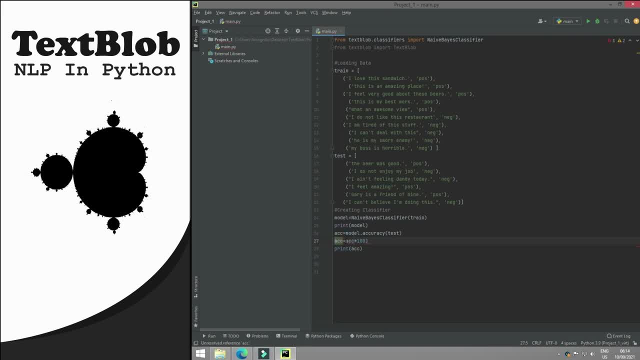 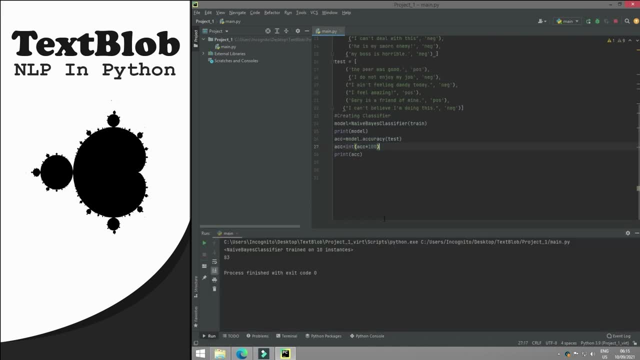 100, okay, and then I will convert that value to int- i NT- and then I will print a double C. so let's check the accuracy. okay, so our model is 83% accurate. so this is very cool, this is very awesome. so this is how you can check the accuracy, just 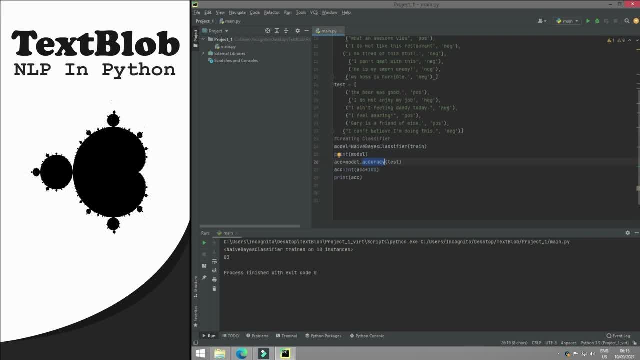 use this accuracy function and pass the data set, our de testing data set, and this will tell you how much accurate your model is. okay, now let's update our model. okay. so just right here, updat, update. okay, and i will update our model. so updating a model is very simple. just right here, model dot up, update. okay, inside this update, we 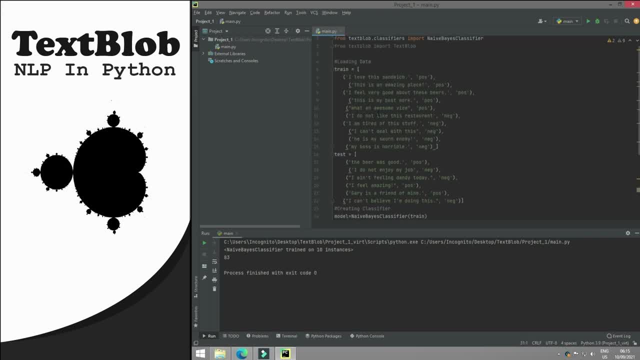 will pass our new data set. okay, so i have copied a new data set and i will paste this data set right here. okay, so this is my more data. okay, and this is also a list having uh sentence and its answer: okay, and i will pass this. more data here. more data, okay. and now i will check the accuracy of 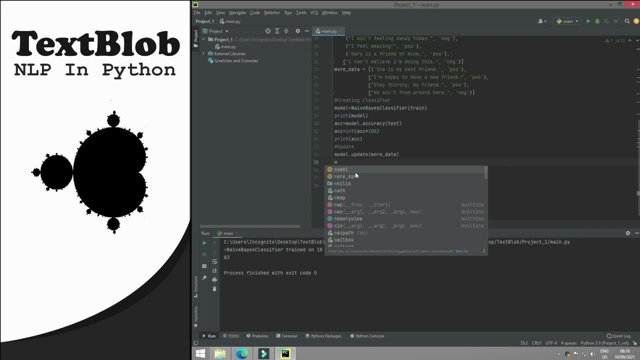 my this model okay, so just right here. model dot awc. accuracy okay, and just pass here: test okay and i will save it. copy and paste is equals to this, and just copy these two lines as well. copy and just paste it, not text. test, test okay. so, uh, i hope this will increase the accuracy of my model and yes, 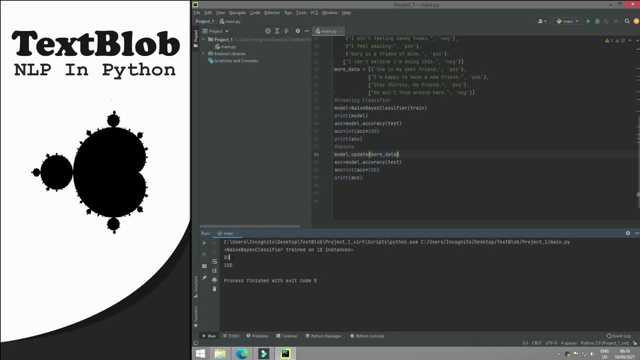 previously our model is 83 percent accurate, okay, and now the accuracy of our model is 100 percent. so you have made a text classification system. so in this tutorial we will talk about sentiment analyzer. and now i know very well you are thinking that we have done sentiment analysis, then why we need a sentiment analyzer, so i will. 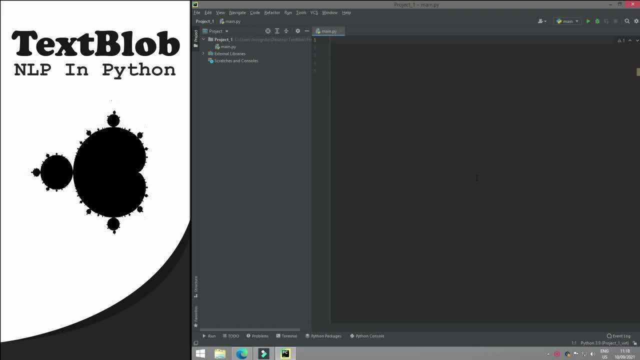 answer this question in this tutorial, so let's begin the lecture, okay. so, uh, basically you have a very valid question, so let's begin the lecture, okay. so basically, you have a very valid question and that is: we have done sentiment analysis and now why we need sentiment analyzer. so this is: 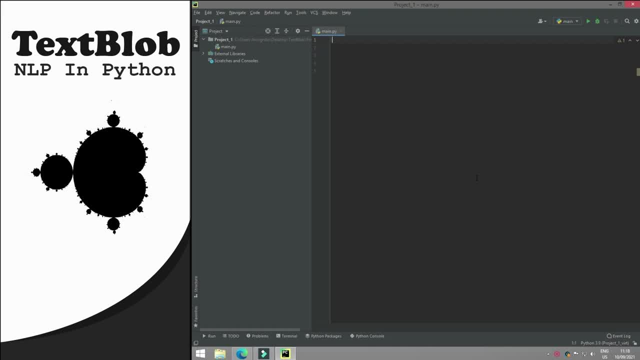 basically an advanced tutorial, okay, so let me tell you the secret, and that is text blob dot. sentiments module provide us two different type of sentiment analyzers. okay, so one is. one is pattern analyzer- okay, and that is based on pattern library, so it is a natural language processing library for python. 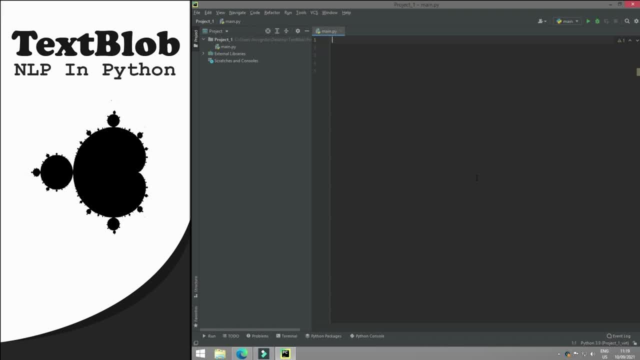 and the next analyzer that we have in this text dot sentiments module, is navba analyzer. so this is a nltk library classifier, okay, and this. the amazing thing about this navba analyzer is that this analyzer, or this classifier, or this model is trend on movies review- okay. so 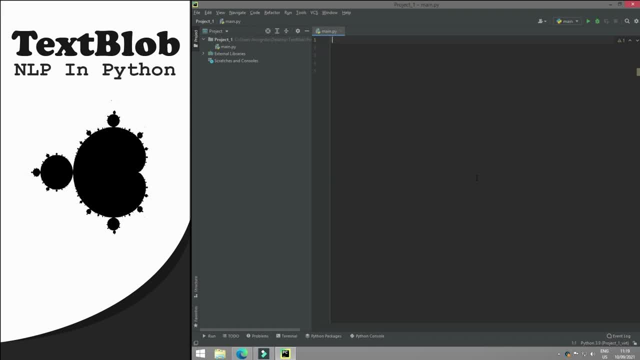 this is an awesome thing. okay, regarding this navba analyzer, so the default analyzer for sentiment analysis, as we have done previously, is pattern analyzer. okay, so we have done our analy, our sentiment analysis, with patron analyzer and now, in this tutorial, we will use our navba analyzer, which is based on nltk. 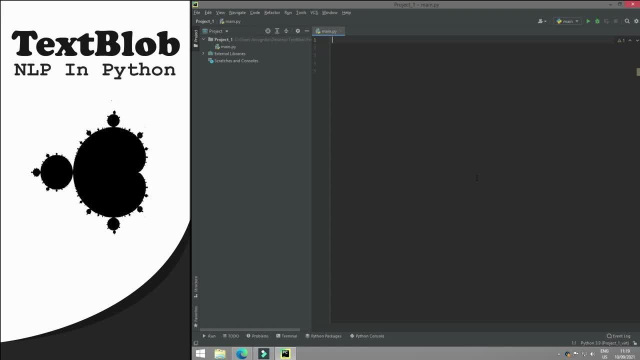 library. uh, let's start the coding. so first of all i need to import my text block class. okay, so just right here, from text blob: i m p o art. import v l o b v l o b. import text blob. okay, and now we need our sentiment. 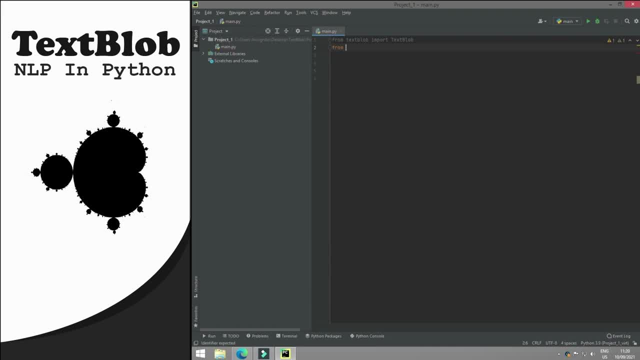 analyzer, and that is from text text: blob dot sentiments: okay. import navba analyzer: okay. so this is again based on your navba analyzer. so this is again based on your navba analyzer. okay. so this is again based on your know very well, uh, base theorem: okay, which is a probabilistic theorem. okay. so now. 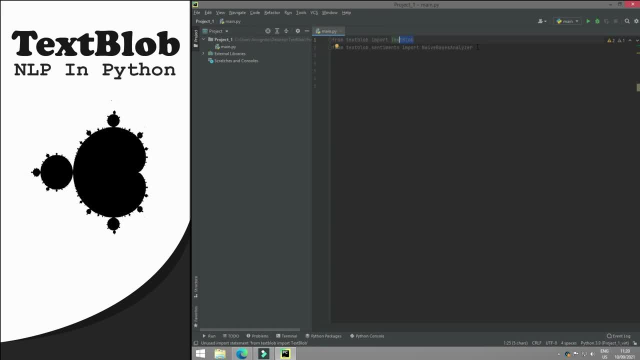 we have my text blog class and my and i have my this navba analyzer and let's create a blob. okay, so blob v l, or the blob is equals to uh text blob. okay, and here i will pass my sentence like: uh, this is an amazne. 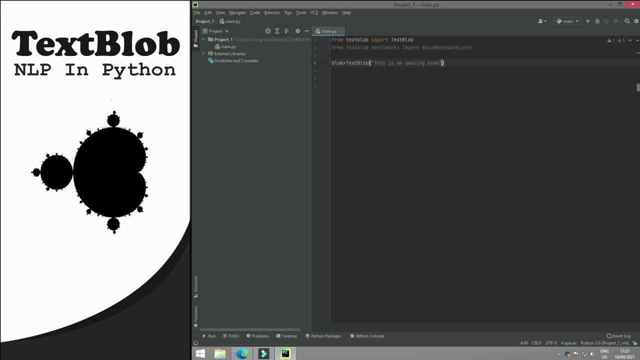 um me세요 b كرةiano. okay, this is an amazing book. okay, and i will. now i will override my analyzer. okay, so the default analyzer is a pattern analyzer. okay, but i want to override it. okay, so i will explicitly define my analyzer. so, just right here, and a analyzer is equals to an ive nav analyzer. okay, and put: 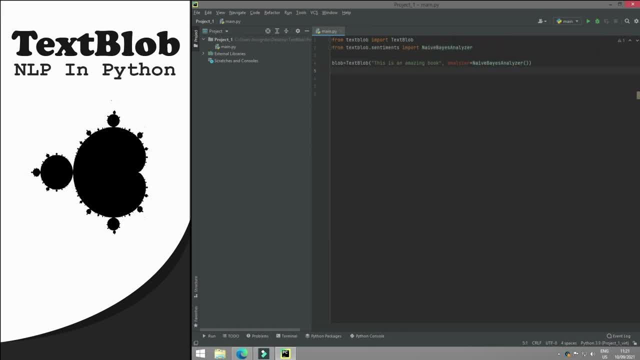 rounded brackets. okay, and now it's very simple. we have talked about this thing just right here: blob b-l-o, blob, blob dot. sentiment: okay, sentiment, and it will perform my sentiment analysis. just print it, okay, and you will notice that my pattern analyzer was returning. i think two things. 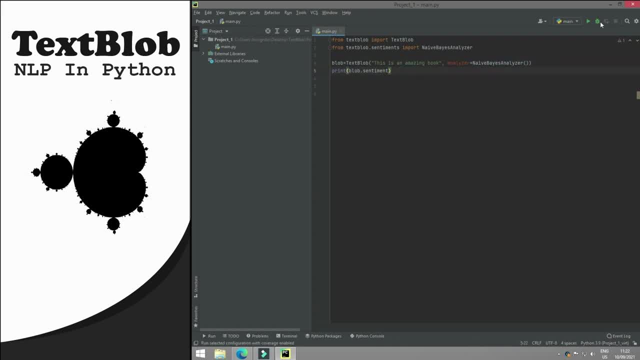 but this analyzer basically returns three things, okay. so if i run it, okay, so this basically. this analyzer returned three things: the classification, the p underscore positive and then p underscore negative. so classification tell us whether this sentence is positive or negative. so this sentence is positive, okay, and this is the positive percentage. 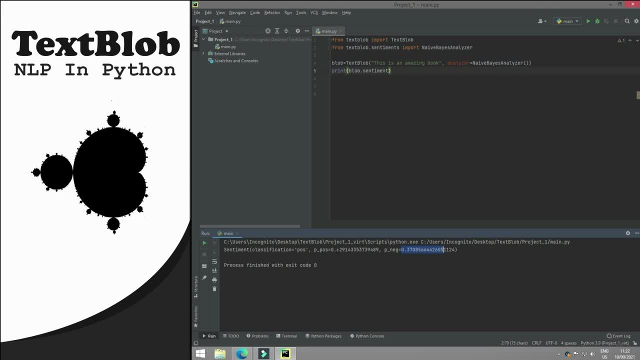 okay, and this is the negative. so actually, this is not in percentage. this is a float value and its value is between zero and one. you can convert these values, okay. so, for example, for example, i do not want these values. okay, i just want to print this classification. 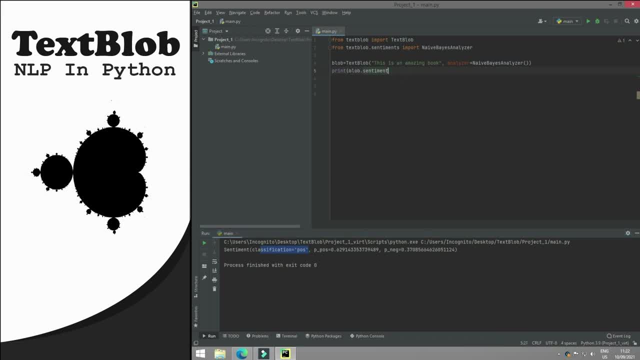 value. so it's very simple, uh, first of all, uh, just uh, uh, store the value. r-e-s-u-l-t result is equals to send blog, blog dot sentiment, okay, and then print uh r-e-s-u-l-t result, dot uh classification c-l-a-l-l-s-i-f-i-c-a-t-i-o, and make sure that you are 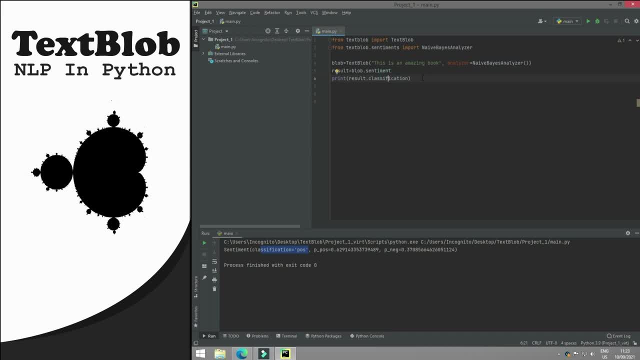 showing that p-under towards in the cl-and this is negative, kind of. let's take another point of reference. you have a letter, but for now, just by placing your in the cl-and, we have three answers. okay, for example, i just typed this… name or, and this name should match. okay, so there is one more way i'll tell you that. 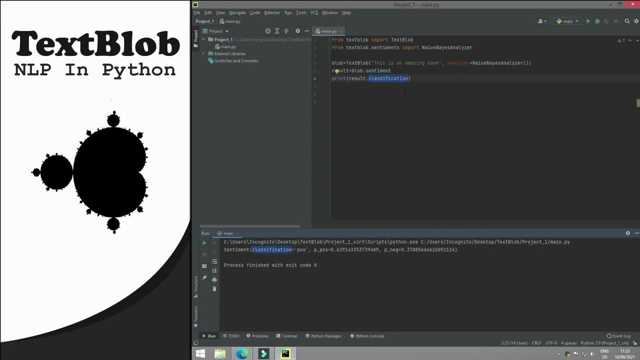 letter. but for now, just type this name as it is, or you can copy it and then paste it here, and if i run it, it will now print just the value of classification. okay, okay, so here is my output and that is positive. so this sentence is positive and you can print the. 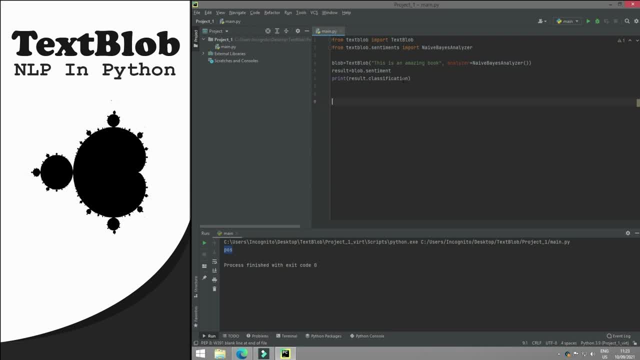 p underscore positive value as well, and the p underscore negative value as well. uh, but there is one more of printing all of these values, and that is: you have noticed that when we run this function, it returns three things: the classification, p underscore positive and p underscore negative. 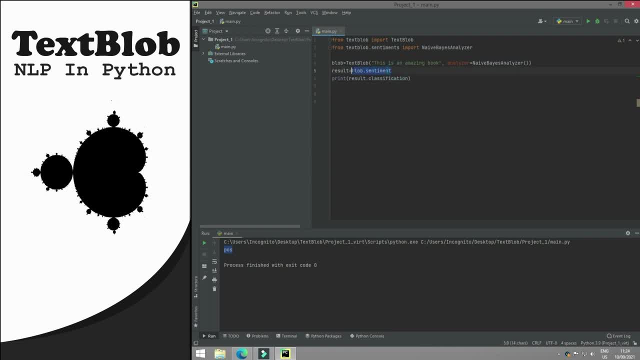 so instead of storing all of these values in this single variable, i will create three different variables. so just write here results or result will be my classification variable, and for p underscore positive i will go with positive variable, and for p underscore negative i will go with negative variable. okay, and now, instead of writing here result dot classification, you just 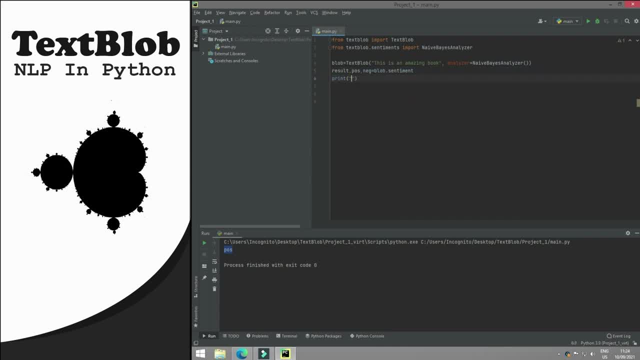 need to write here result, like, for example: i will say r-e-s-u-l-t result- okay, and i will print result here and then in the new line: okay, in new line i will say: uh, you positive. okay, and i will print my positive value here and then in the next new line i will say: 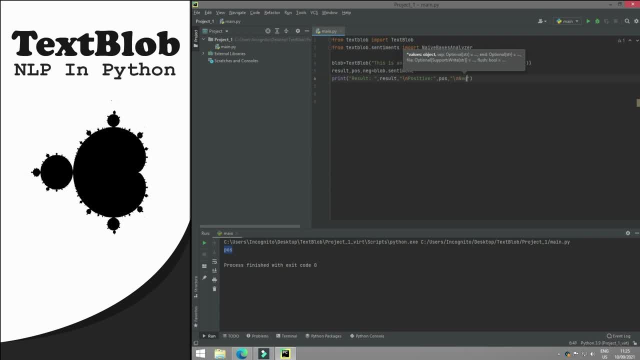 negative, n-e-g-a-t-f. negative, and i will print my negative value here: n-e-g. okay, and now you will notice that it will print three values here. okay, so this is my output. okay, so my result is positive. my positive value is 0.6 and my negative value is 0.37. so this is awesome. so i hope you have. 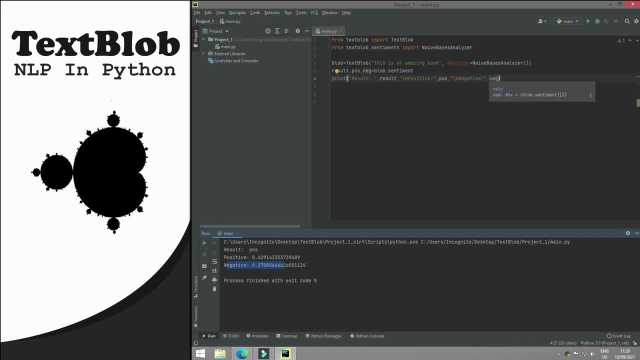 understood about sentiment analyzer. so just keep in mind there are two types of analyzer: the pattern analyzer, the nav base analyzer. so pattern analyzer is our default analyzer and you can overwrite the default analyzer just by defining on analyzer here. and then everything else you know very well. so in this tutorial we will see how we can use nltk tokenizers in text blog. so let's begin the 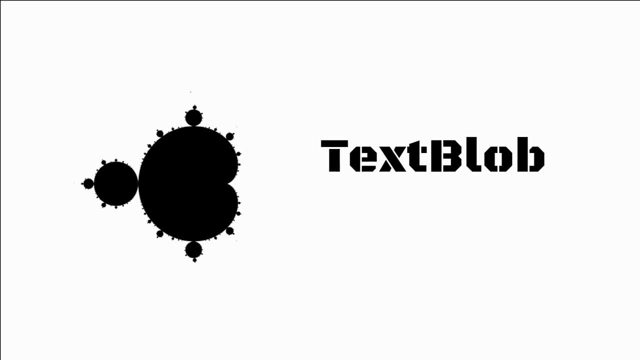 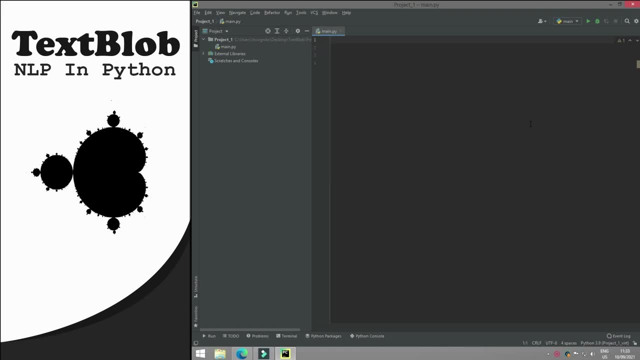 lecture. okay, so we have done a tutorial on tokenization where we were using dot volt function- okay, but in this tutorial we will see how we can use nltk tokenizers- text blob. so first of all, let's import my text blob class. okay, so from text blob, import, import text blob. okay, so, text blob, it's awesome. and now I need to. 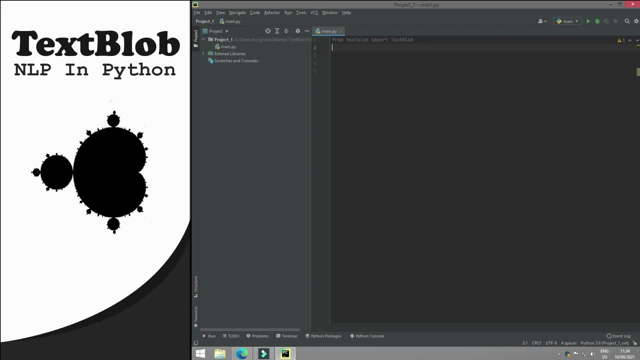 import tokenizers, different types of tokenizers, from NLTK library- okay, so just right here. from NLTK- okay, and NLTK dot T- okay, and tokens tokenize. and from NLTK- dot tokenize. I need to import different types of tokenizer, like, first of all, let's go with tab tokenizer- okay, so, tab tokenizer, and I would use my tab. 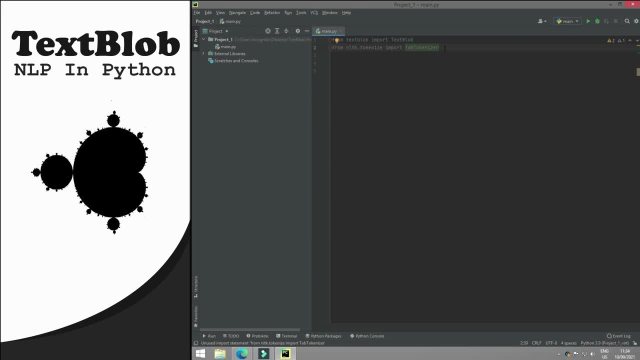 tokenizer to to separate or to slice my sentence. okay, so I will click on the tab tokenizer and I will click on the tab tokenizer and I will create a blob of text. here blob is equals to text, blob- okay, and I will pass my sentence here. for example, this is a sentence, okay, and now slash T. so this: 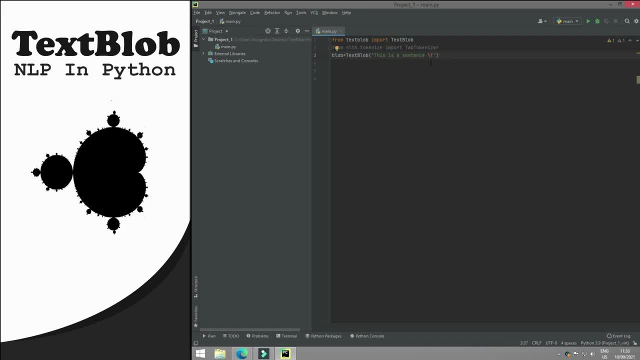 slash T represent tab. okay, so this is a sentence: slash T, which is very simple. okay, so, which is very simple. okay, so, which is very simple, and now we need to override the default tokenizer. okay, so, which is very simple, and now we need to override the default tokenizer. okay, so, 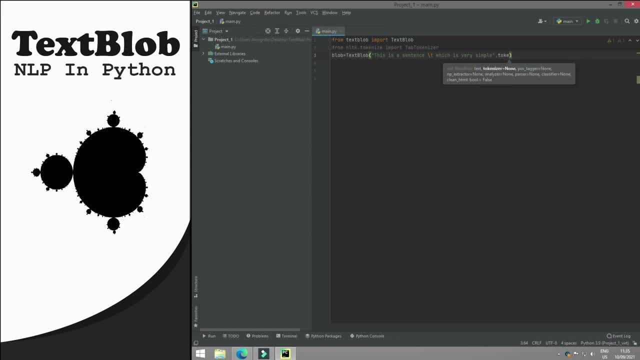 just right here to okay and tokenizer, okay. and now we need to define our just right here to okay and tokenizer, okay. and now we need to define our tokenizer here. so in this case, our tokenizer is this tab tokenizer, so just tokenizer here. so in this case, our tokenizer is this tab tokenizer, so just. 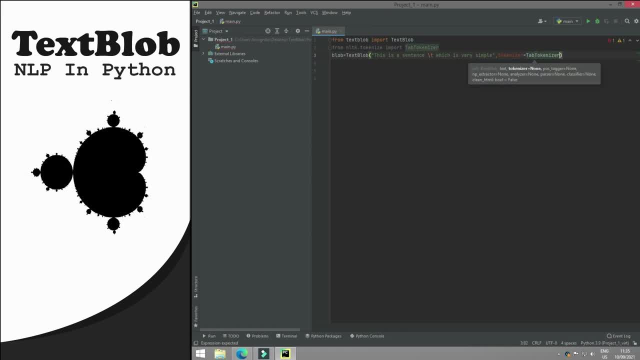 right here, tab tokenizer. okay, tab tokenizer. and make sure that this tab right here, tab tokenizer. okay, tab tokenizer. and make sure that this tab tokenizer is a class. okay, so just put rounded brackets here. okay, so now we. tokenizer is a class okay, so just put rounded brackets here. okay, so now we. 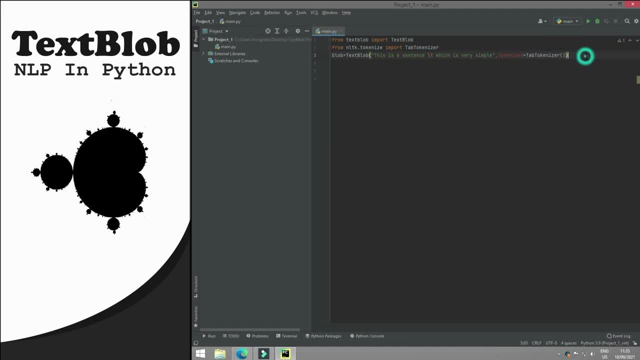 have overrided our this tab tokenizer- okay. so now we have overrided our this. have overrided our this tab tokenizer- okay, so now we have overrided our this. have overrided our this tab tokenizer- okay, and let's tokenize this sentence. 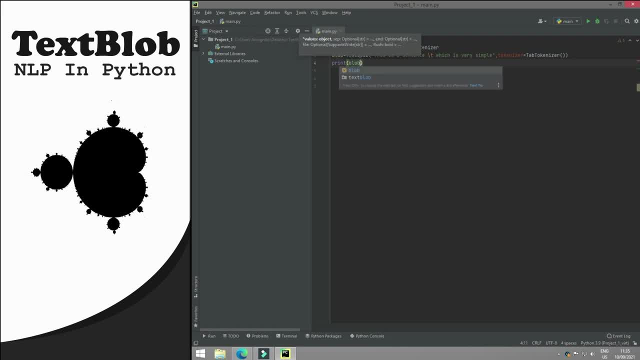 tokenizer- okay, and let's tokenize this sentence. tokenizer- okay, and let's tokenize this sentence. so just print it. print blob dot. so just print it. print blob dot. so just print it. print blob dot. t-o-k-e-n tokenize- okay, so it's cool. t-o-k-e-n. tokenize- okay, so it's cool. 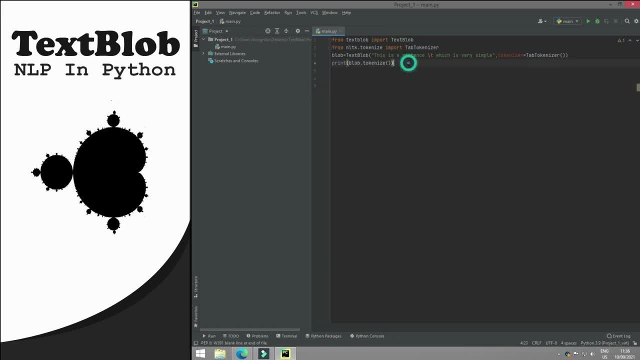 t-o-k-e-n. tokenize. okay so, it's cool. okay, so if i run it, you will see that. okay so, if i run it, you will see that. okay, so if i run it, you will see that in a single list, we will have only uh. in a single list, we will have only uh. 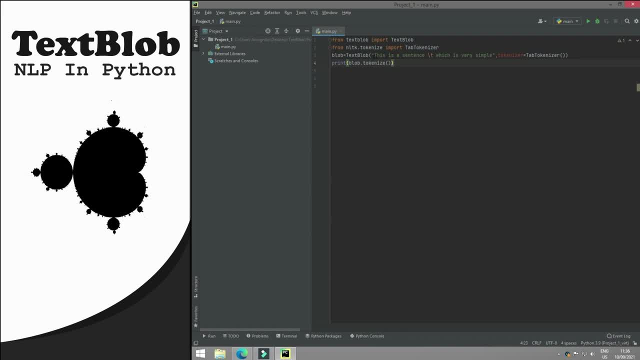 in a single list. we will have only, uh, two, what i said, two values, okay, so one, two. what i said, two values, okay, so one will be this, okay, and then you one will be this: okay, because we are using tab tokenizer and it will slice my sentence right there, okay, so if i run it, you will see we will have a list. yes, we. 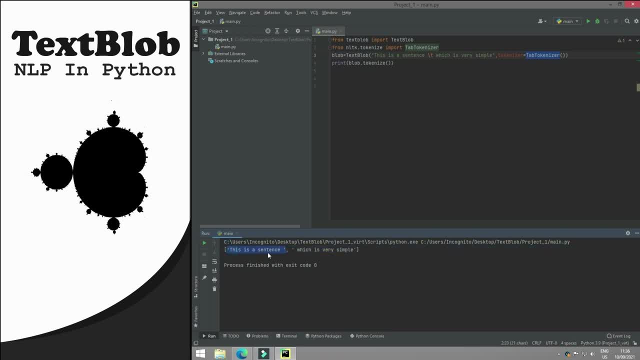 will have a list and it has only two values. okay, this is a sentence, and then this is my next sentence. okay, our next value. so this is how you can use nltk tokenizers for tokenizing a sentence in text block. so there are a bunch of other tokenizers, like, for example, if i write here: 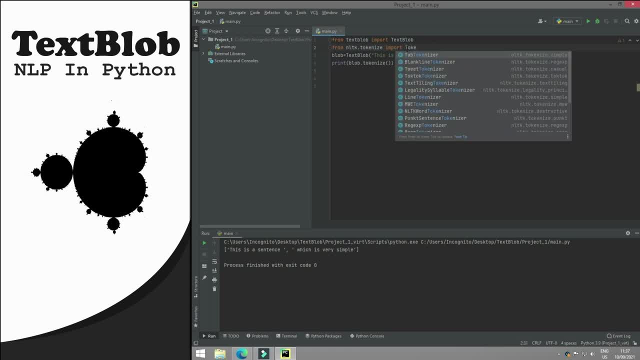 tokenizer. so you can see that we have this tab. okay, sorry, this tab tokenizer. blank line tokenizer. okay, this tweet tokenizer, talk talk tokenizer. text styling tokenizer. so we use these different types of tokenizers in different scenarios. for example, let's go with this blank line tokenizer, okay, and just remove this tokenizer and i will write here: blnk, blank. 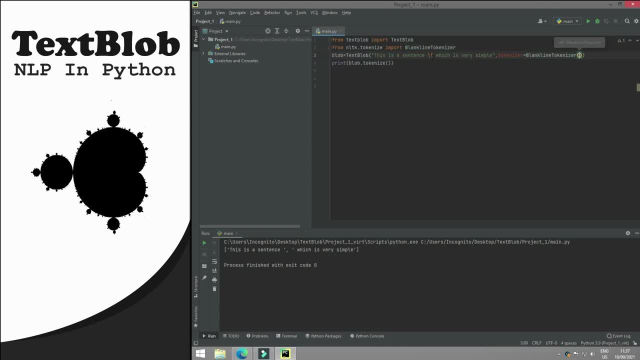 line tokenizer and put the rounded brackets here and instead of slash t, i will say slash n and again slash n. okay, so this n will separate my this sentence, okay, and this n will move my this sentence to new line and this n will create a blank line. okay, so make sure that you put double. 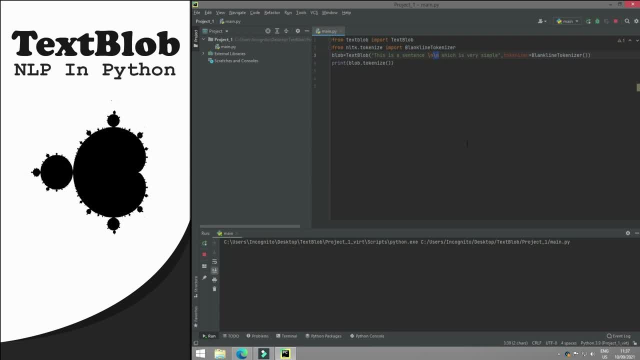 slashes here and then you will get your required output. okay, and yes, this is a sentence and which is very simple. for example, if i remove this one slash and then you will notice that it will return a list with only one object or one value and it this will be this whole sentence. okay, so if i run, 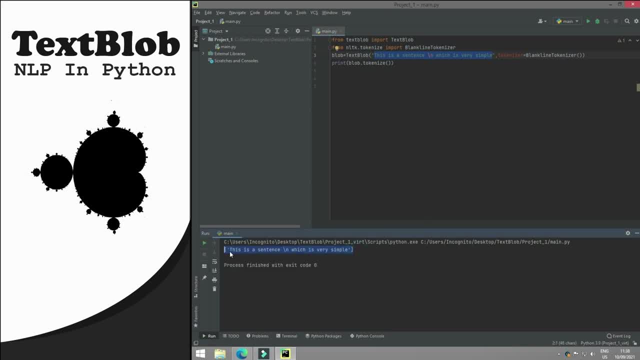 it, you, okay. so this is a list and it has only one value. this is because we have used a blank line tokenizer and in this sentence we do not have any blank line. okay, so make sure that you put to double n here. or, for example, let's put double n, double n here as well. double n, okay, and let's 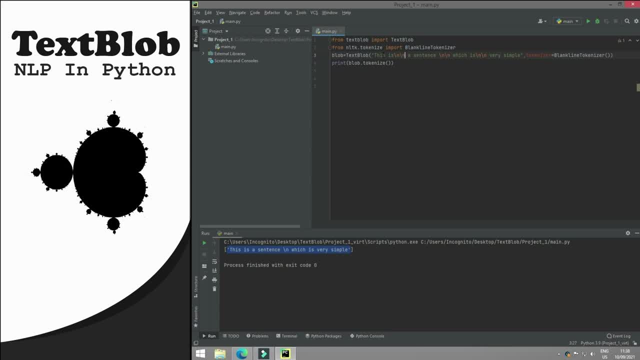 put double n here as well, slash and slash, and now it will return one, two, three, four, four values. okay, so, if i run it over here, okay, so this is our sentence, which is very simple. so this is how you can use nlt tokenizers in textblock. so in this tutorial we will talk about 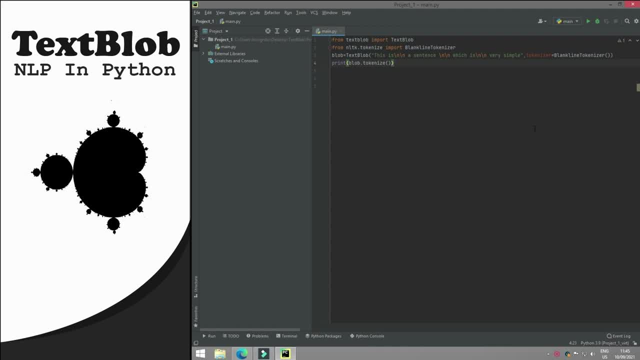 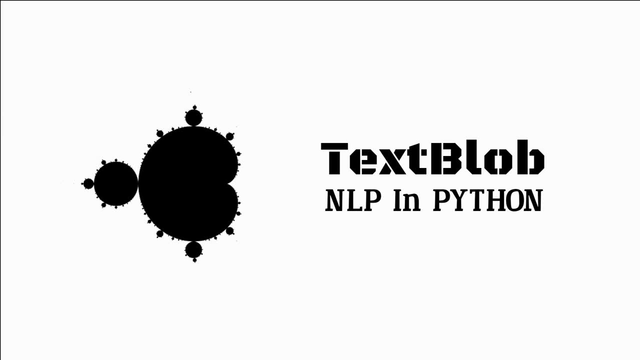 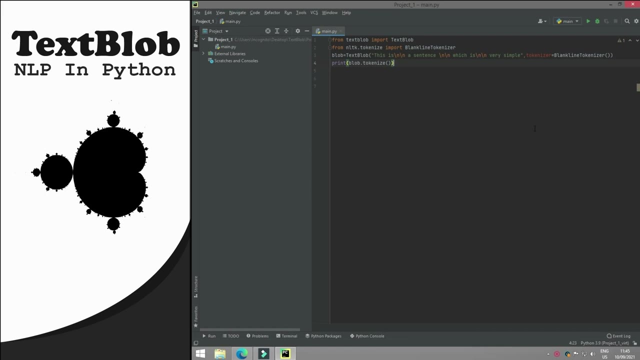 noun phrase extraction again, yes, again. so let's begin the lecture. we have talked about noun phrase extraction previously, okay, but in this tutorial we will talk more about noun phrase extraction. so basically, the text blob dot np extractor module provide us two different classes for noun phrase extraction. one is this: fast npx extractor. 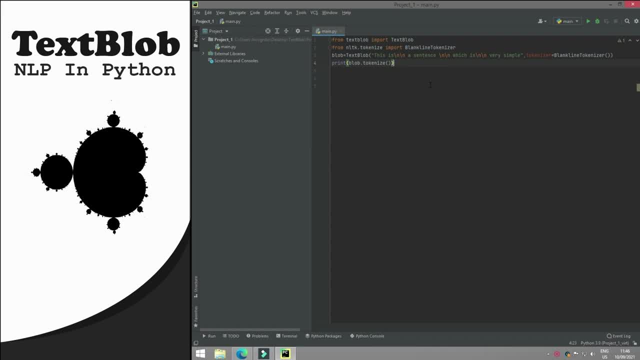 which is the default extractor for noun phrases, and we have an other extractor and that is kernel extractor. okay, so i hope i will pronounce con correct and that is c? o n double l kernel. okay, kernel extractor. so we will override the default extractor and use this kernel extractor. let's. 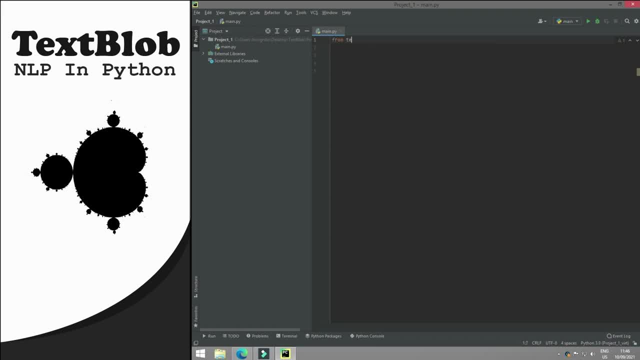 remove everything. okay, just remove it. and right here, text blob i. i m p o r to import text blob class. okay, so it's cool. and now we need to import our noun extractor. so just right here, from text blob: dot np. text b l o b dot np. extractor. import c o n double l. 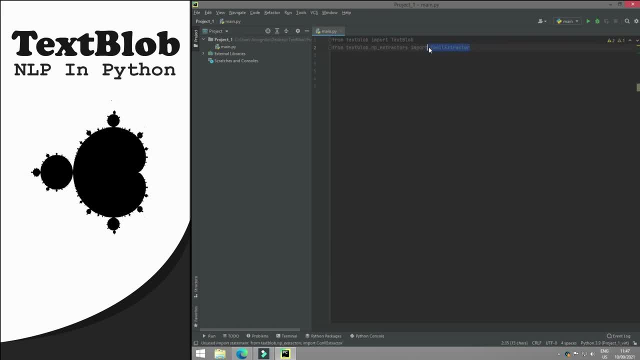 extractor, and now we will use this extractor to extract our noun phrases. okay, so just create our blob here. blob is equals to what text? blob, okay, and just right here the sentence: this is a noun PHR phrase as the NT. and sentence: okay, I like red apples, or red apples a double PA, the Arab apples very much okay. and now let's. 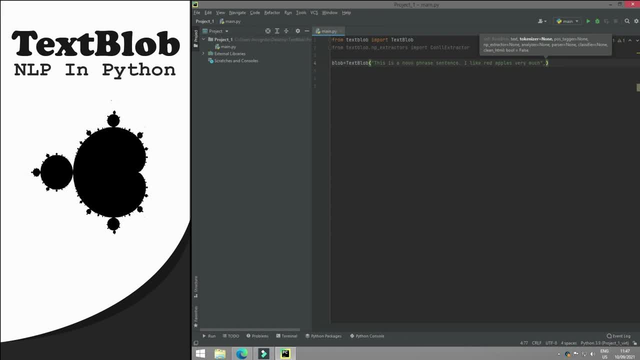 overwrite the default noun phrase extractor. so just right, here noun phrase extractor is equals to C or n. double L O'Connell extractor. okay, and put the rounded brackets again, because this is a class. okay, and make sure that you should put round brackets here, otherwise it will throw an error. 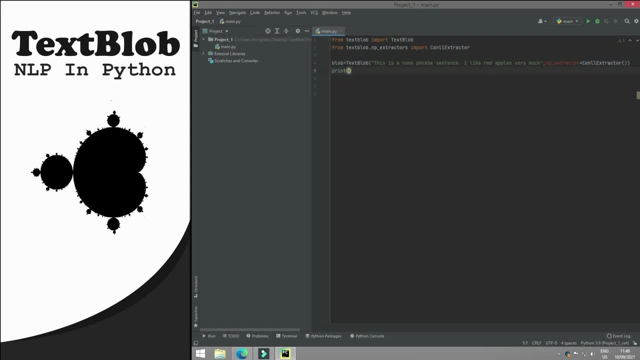 you can. now we need to print noun phrases, so blob dot noun phrases, okay. so if I run it, okay, so noun phrase sentence is my only noun phrase in this sentence. okay. so, for example, instead of this, let's write Python, okay, pytho, and so Python is. 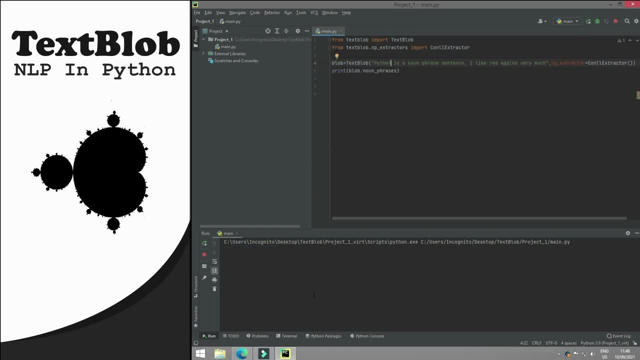 also my noun phrase, so if I run it it will print Python as ok. okay, so, yes, python. python is my noun phrase and noun phrase sentence is again another noun phrase. okay, in this tutorial we will talk about part of speech tagging. okay, and how to overwrite the 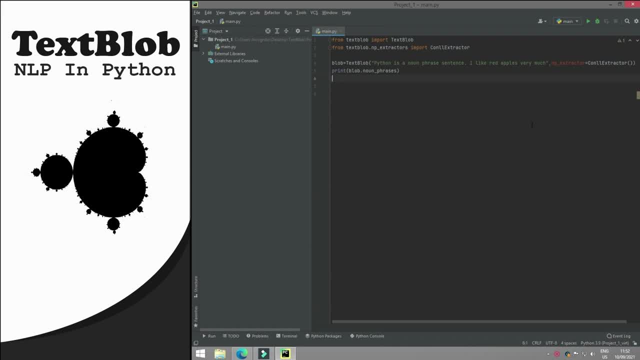 default part of speech tagger, so let's begin the lecture, okay, so first of all, this is my sentence. okay, and this text blob actually provide us two different types of part of speech tagger. one is based on patron library and the other one is based on nltk library. this so the parts of 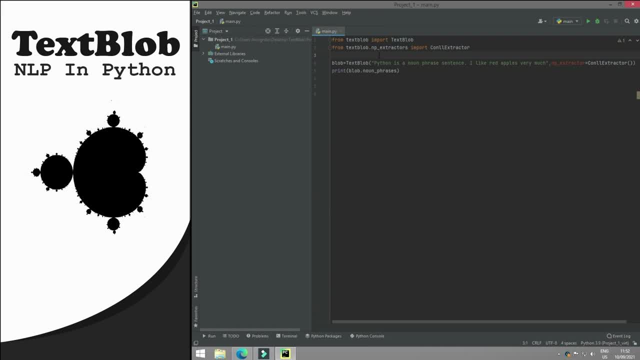 speech tagger which is based on patron library is called patron tagger, and this is our default tagger, and the one which is based on nltk library is called nltk tagger, and this nltk tagger actually requires numpy. okay, so we will install numpy, so it's very simple. 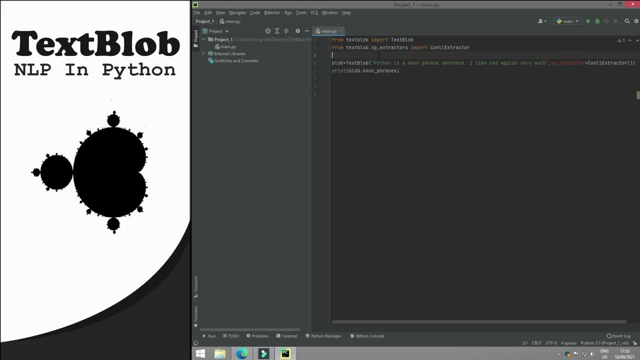 in the term, we will open our terminal and we will just type pip, install numpy. and if you already have numpy then you do not need to install it, okay, so let's first of all let's import our tagger, and in this case we will import nltk tagger, because patron tagger is our default tagger. so 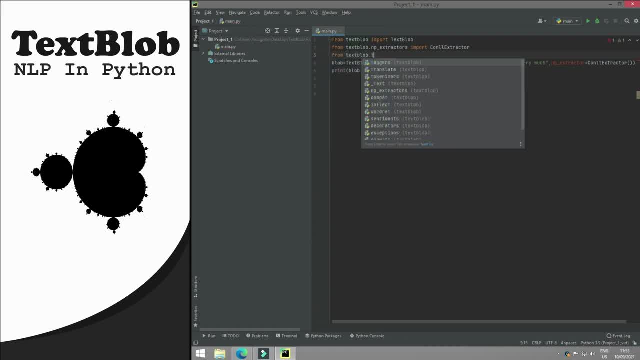 from text blob dot t, a, double g, er taggers: import uh, nltk. nltk tagger. okay, and instead of np, extractor. now i will write what i will write. i will write pos, okay. so pos basically represents parts of speech, okay, and that's why it is. it's not the abbreviation of position, okay, so this: 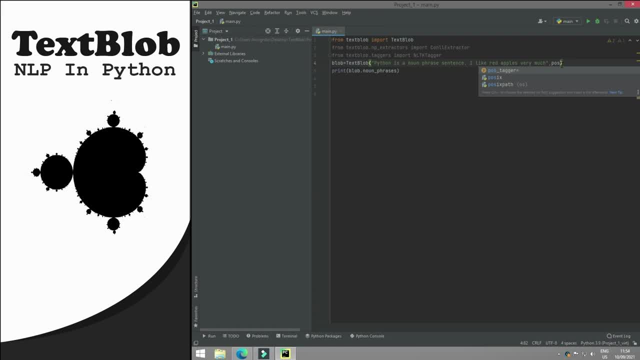 is actually the abbreviation of position. okay, so this is actually the abbreviation of position. abbreviation of parts of speech. okay, so p-o-s underscore t-a-double-g-e-r tagger is equals to an l-t-k tagger. okay, and just put rounded bracket here and now in this. 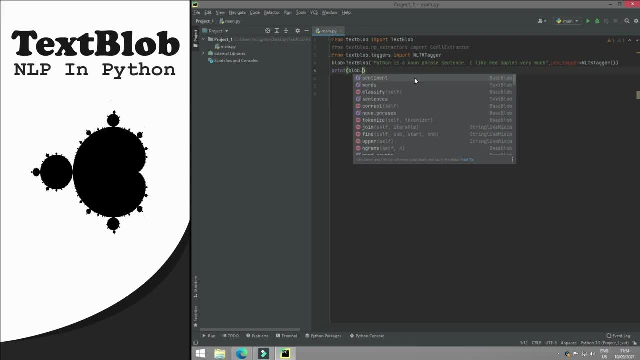 there i will write blob dot. uh. what text? okay, blobtags, yes, blobtags, and if i run it it will okay. so we got an error. that is a list of object. okay, so this basically return a list. so do not put these rounded bracket here. okay, so this is my list, and python is my noun, is my word, uh is. 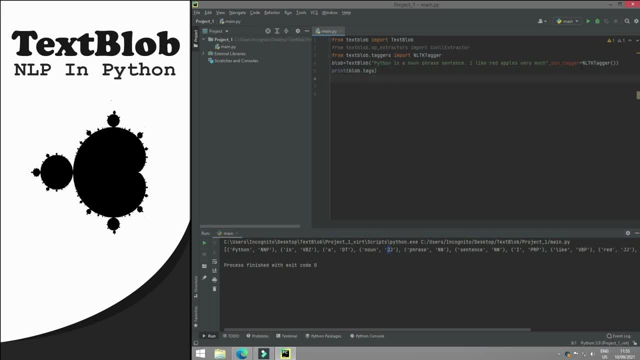 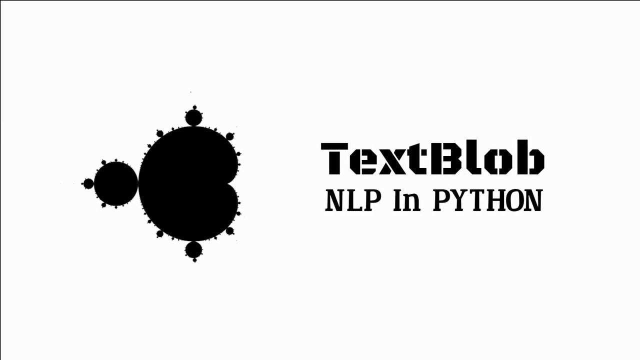 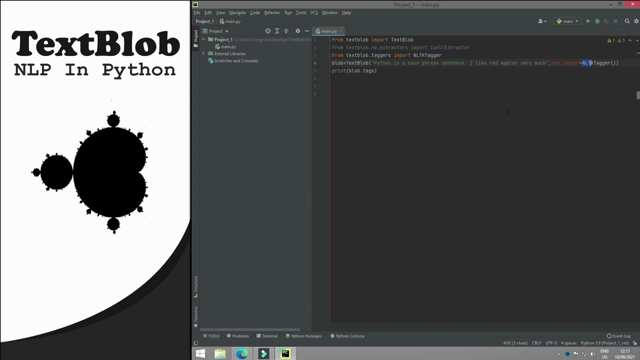 my dt, and this is how you can actually overwrite the default noun tagger using this nltk tagger. okay, you have enjoyed this tutorial. have enjoyed this tutorial. in this tutorial, we will talk about blober, so let's begin the lecture, okay, so before i talk about blober, or before you understand the concept of a blob, 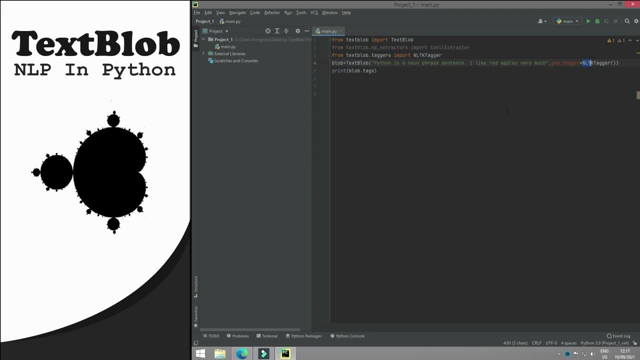 it is very important to do some practical work regarding blob. okay, and that is why we combine two types of object, one and another, and also, this method is going to be salt, and you have enjoyed this tutorial, f you have enjoyed this tutorial. in this tutorial, we will talk about blober, so let's begin the lecture. 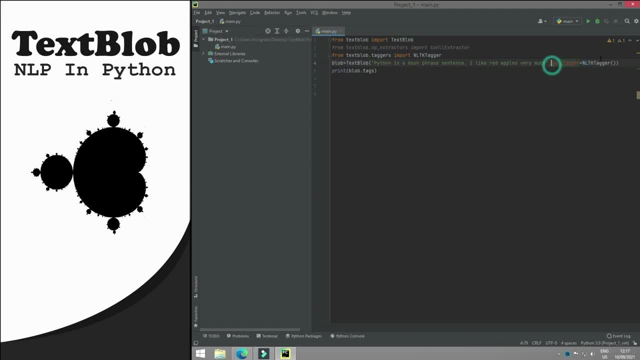 is, for example: for example, I have this post tagger here, okay, and I have another blob, like, I will name it like blob2- okay, is equals to text blob, okay. and then I will write a sentence. this is this is a simple sentence, okay, and now we need to define our post tagger, default post tagger here, copy it. 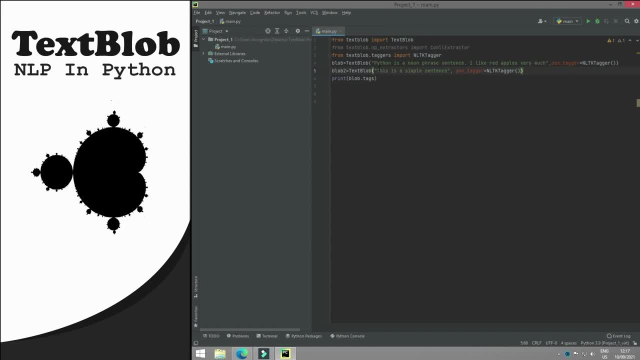 and paste it here. so defining the properties for different blobs- okay, from for different text blob is quite difficult task. for example, in many scenarios you will have your own custom post tagger, you will have your own custom sentiment analyzer- okay, and you will have so many text blobs, okay. so it. 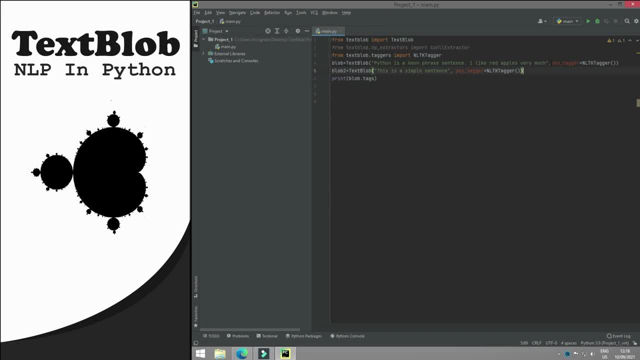 becomes very difficult to define your own post tagger- okay. and now we need to define our text blob. okay, and we need to defined text blob- okay. so it becomes difficult for us to define each of these proper properties separately in this text blob. so we need such a class in which we will define our these. 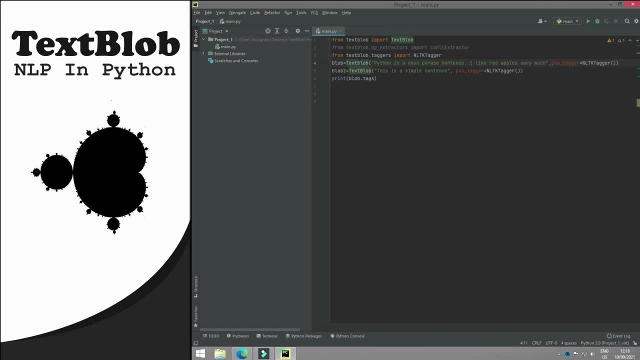 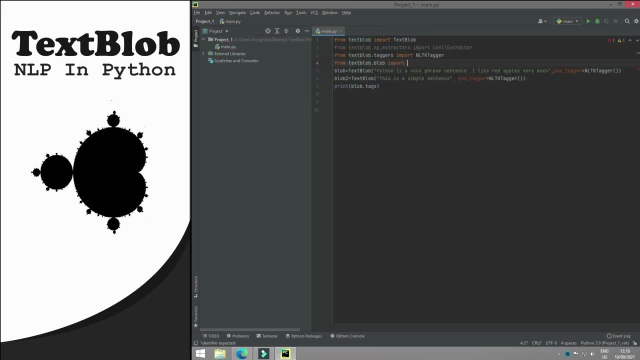 dot BLO blob. from text dot blob- import BLO blobber. okay, import blobber. and now this blobber will allow us to define these properties globally and whenever we will use the variable assigned, that we will assign to this blobber. whenever we use that class, it will automatically apply these settings. 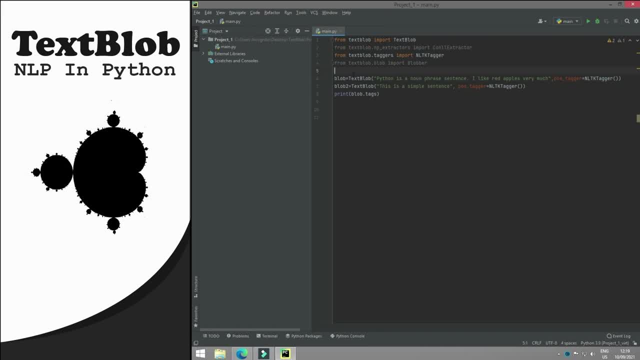 to all the sentences. okay. so what does it? what does it mean? it means that, for example, I will say custom underscore, TB, TB. this means that the text blob- okay, custom text blob- is equals to BLO, BLBER, blobber. okay. and now, inside this class, I will define my these properties. for example, just remove it and just cut. 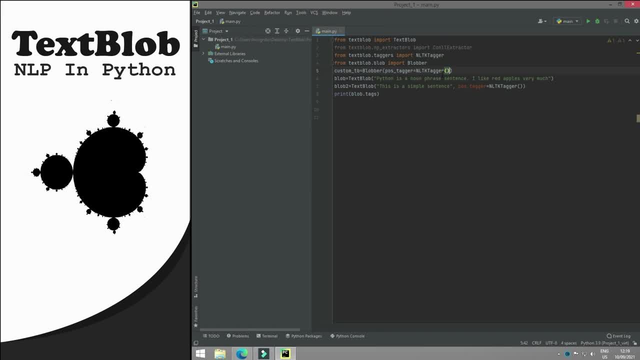 it, cut and paste it here, okay. and for example, I have my own analyzer and a ly analyzer is equals to like. for example, let's import an analyzer here from text blob dot sentiments: import which analyzer should I import an L and a nav base analyzer? okay, so I have my. 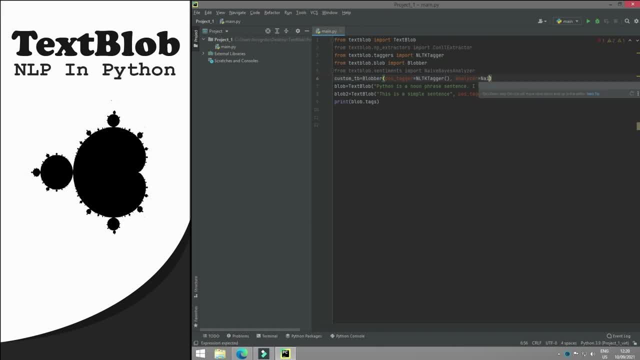 this nav base analyzer and IVE nav base analyzer here. okay, and now I need to apply these properties to all these text blobs. so now, instead of using text blob, I will use by this custom text block. so what does it mean? it means that we just need to remove this, and right here, see STOM custom text blob. okay, and now. 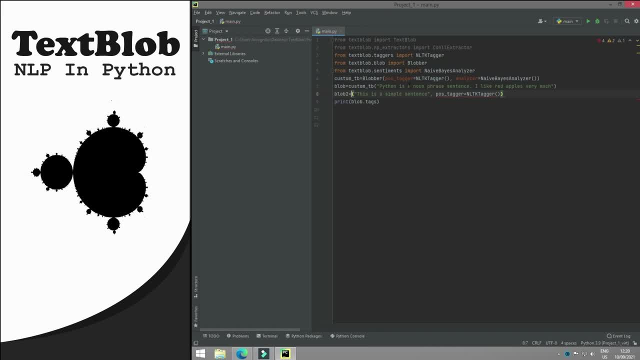 inside this custom text blob. we just need to define our this line, okay, our text, only not the properties. okay, we have. because we have defined all of these properties globally. and now how we can check that whether this blob one or blog two has same post First Tagger? okay, so we need to confirm it. okay, that then. 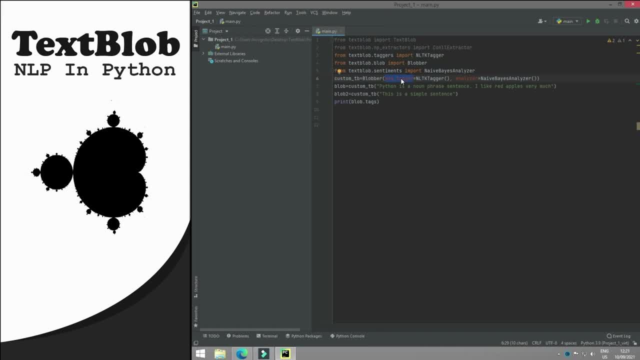 you will believe that I am saying true, or I am true that these blogs have now sent properties. okay. so it's very simple here. I will not print that we bl ob blob dot post tagger is blob two dot post tagger- okay. so if both of these post taggers 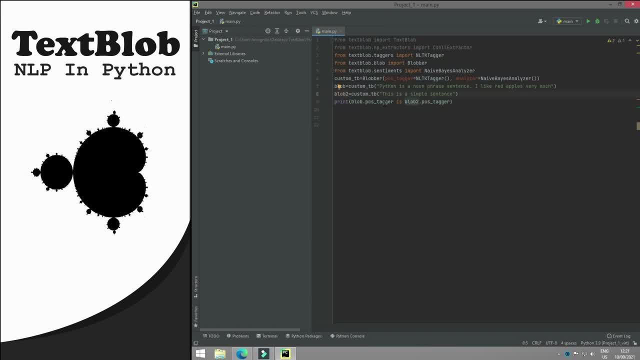 for these blobs are same, then this will print true. otherwise it will print false and it will make my this sentence false, that now these two blobs have same post taggers. so let's try it. okay, so we got true. then this means that this blob one and blob two have same post tagger, okay. 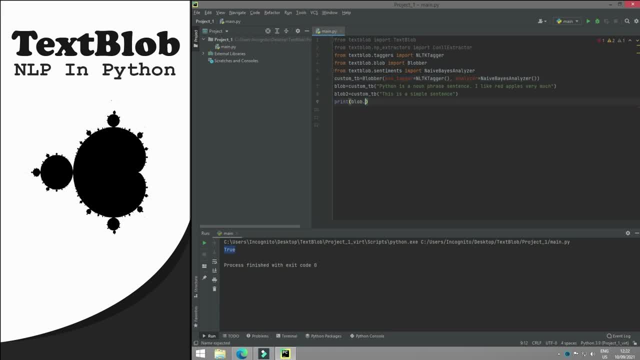 and if i say here, blob one dot tags, okay, blob one dot tags, okay, and it will print the tags of this sentence, okay, with the help of this nltg tagger. okay, and if i say analyzer, so it will override the default analyzer and it will use this nav base analyzer. okay. so just right here, and analyzer and this. 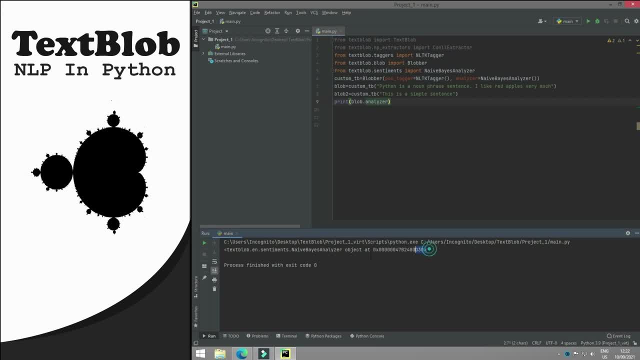 will overwrite the default analyzer. okay, this is my output, and that is: we are currently using nav base analyzer. so this is an other proof. so this is how you can define these properties globally and then you can use them in your whole program. so i hope you have understood the concept. 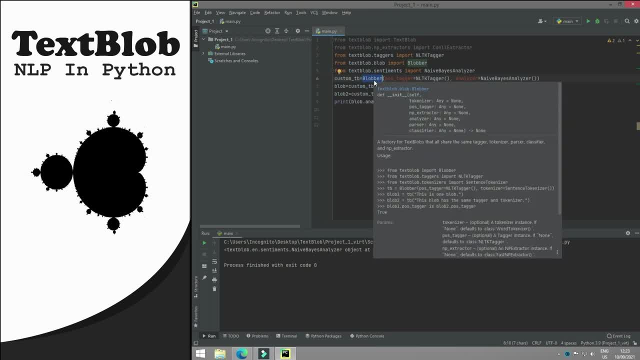 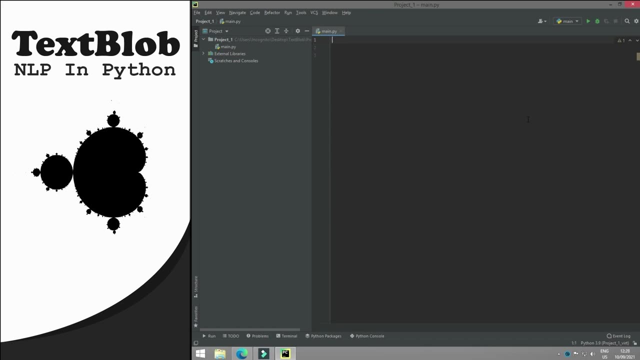 of blobber which really help us in our real world problems. okay, when you are dealing with tons of data, okay, this blobber really help us. so i hope you have enjoyed this tutorial. we will see how we can use text blob for translation and language detection. so let's. 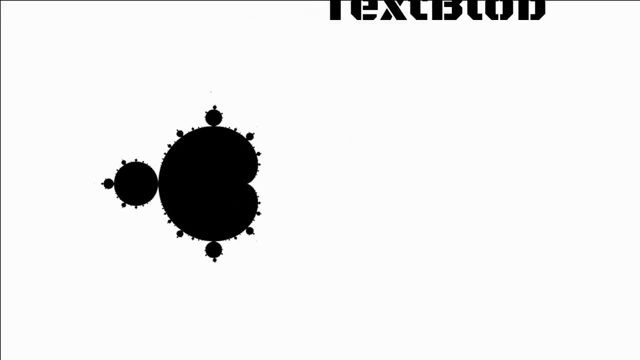 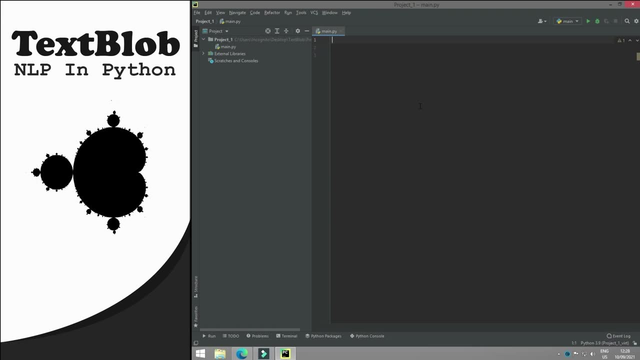 begin the lecture. okay, so first of all, let's create a text blob here of some other language. okay, so from text blob, import text blob. okay, and now create a blob is equals to text blob. okay, and inside this blob i will not write high, okay, everyone, or hello everyone. i will write something other than english, okay, and i will use google. 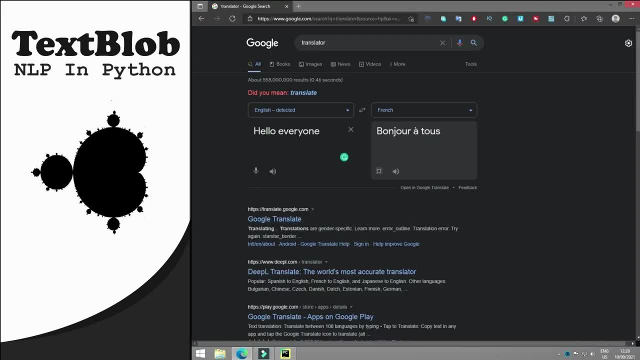 translator because i don't know other languages. so, for example, i have written here this english, okay, and it has converted this english in french, okay, so you can select any language and i will copy this line. okay, just copy it and paste it here and let's see whether our this text blob. 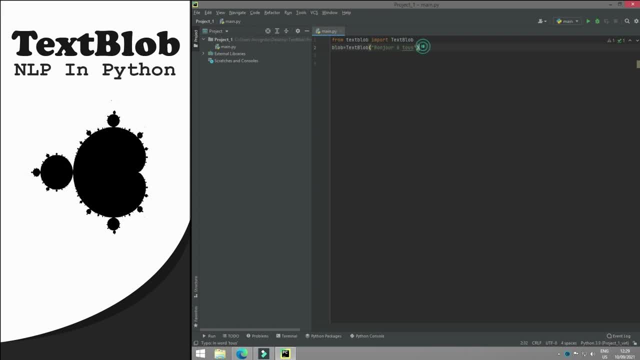 works correctly or not. so, first of all, i want to detect the language, okay, the language of this sentence. so i will write, print, print: blob dot detect language. okay, blob dot detect language, and let's see whether it is correct or not. and yes, fr, this means french, so it is a sentence of french language. okay, and now, uh, let's convert this. 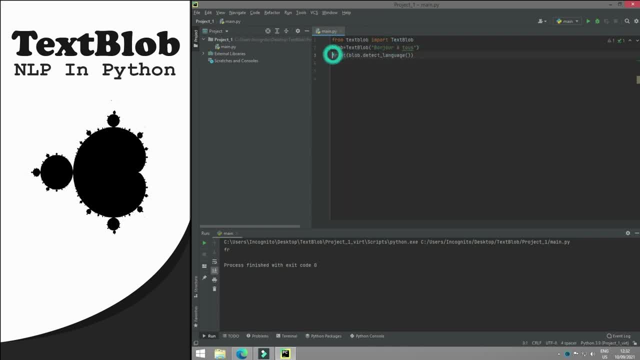 sentence to english, okay, so first of all, let's come into it, okay, and right here print: okay, blog dot translate. okay, blog translate, and i want to trust that. so this from underscore language is, uh, what i say. it's an optional argument, okay, so you, without writing it, it will automatically detect what is the type of language this sentence belongs. 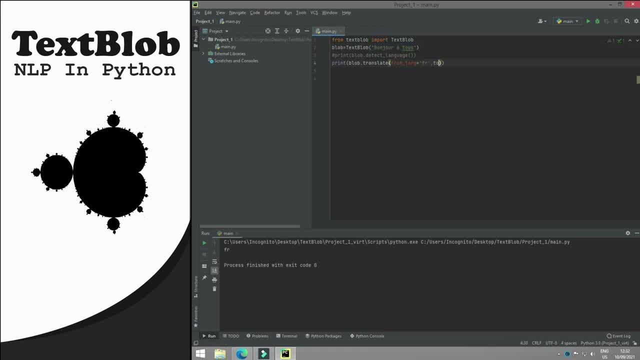 to okay from underscore language is equal to french. i want to convert it to english. okay, two is equals to e and english, and if i run it, you will see that it will print hello everyone. so hello everyone is the english sentence of this line. okay? so i even don't know how to pronounce it. 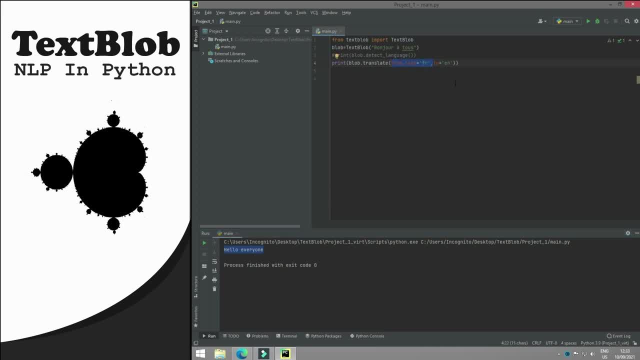 so if i remove this uh statement or this argument here, it will still work. fine, okay, because it will automatically detect it and it will automatically convert it. okay, so it's awesome. hello everyone. so this is how you can use text blob for language detection or language translation. okay, so i hope. 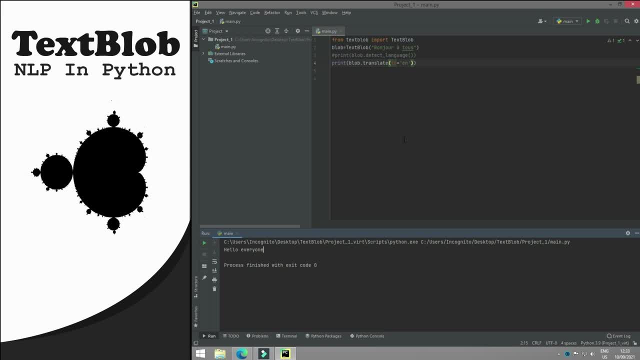 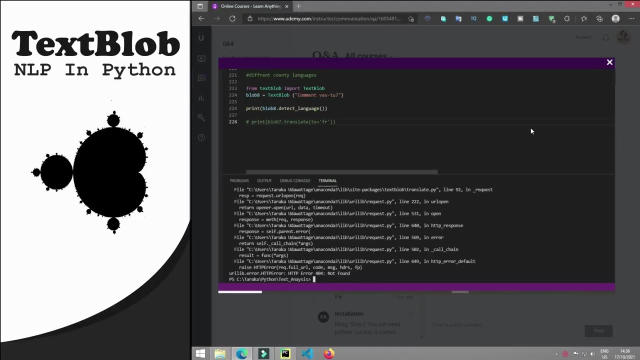 you have enjoyed this course, this whole course, okay, and um, yes, i will see you in the next course, in which i will bring some new things, some easy things, okay, uh, so till that point, bye, bye, hi, everyone. so in this tutorial we will solve this problem. so recently, one of my student just messaged: 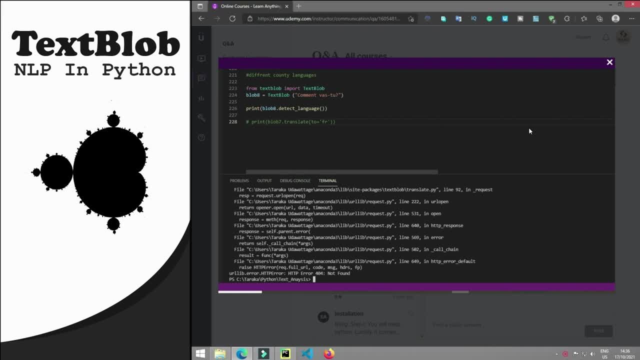 me and he asked for the solution of this problem. and let me explain to you what is he doing. so he is basically, uh, creating a blob, okay, and then he is detecting the language, but he is getting this error, getting the same error. then i think that you should watch this tutorial, because in this tutorial, we 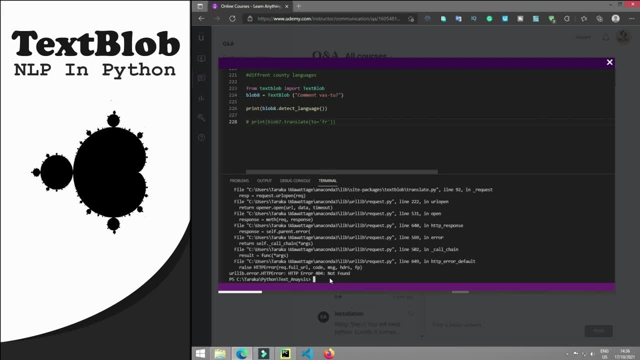 will solve this problem, and it's quite a serious problem. so first of all, to solve this problem, you need to understand how text blob detect languages. so, basically, text blob uses google's api to detect language and you know very well that google has a very, very huge api system and huge 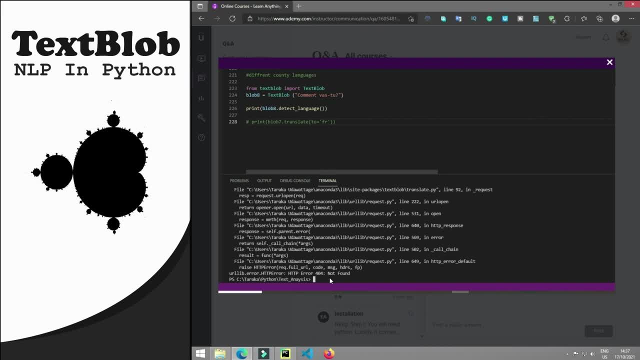 servers and everything okay, and google consistently updates its api system, its servers and everything else. so recently google has updated its api system and that's why you are actually getting this error. so now how we can solve this problem. so the solution of this problem is very simple: you just need to make some changes in text, blob, api or url, which is basically reference to. 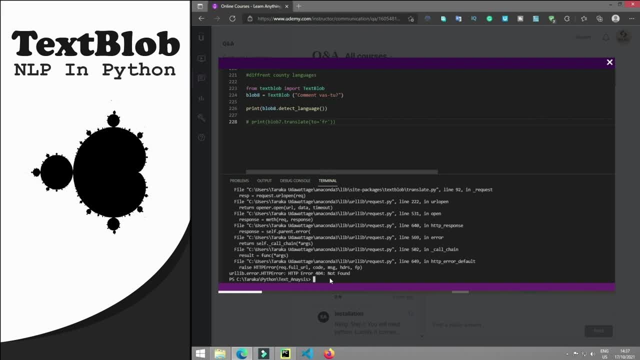 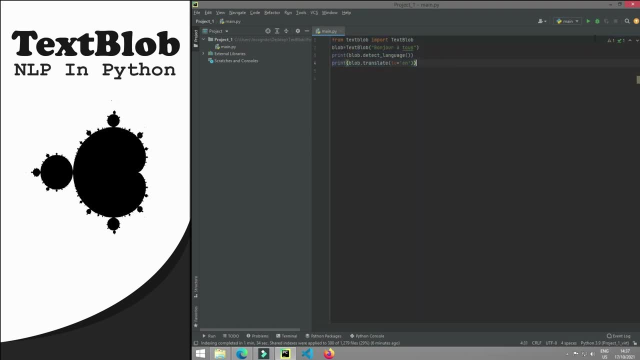 google's api, and then you will get your required results. so, first of all, uh, for example, just open pycharm, okay, and i have this simple program. now let's run it. okay, and this will throw us error. and yeah, here is my error, that is, 404. not found this error, and my this error is same. okay, so now, 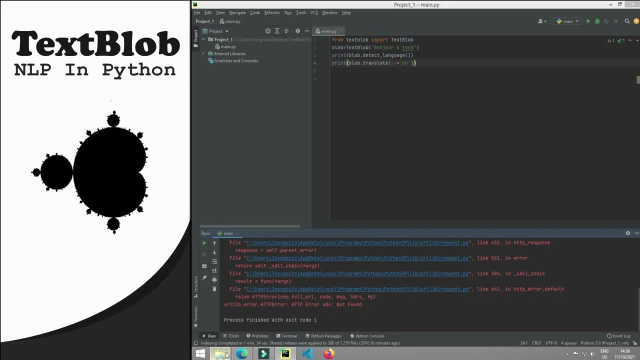 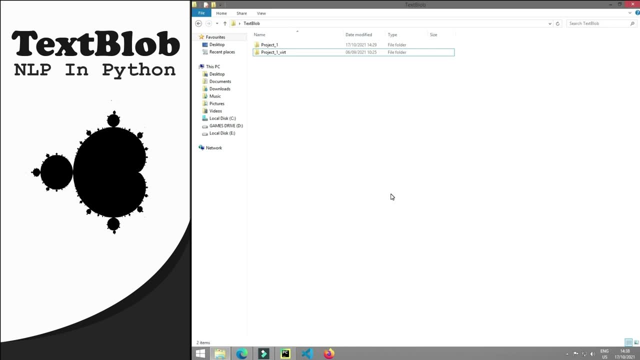 we will solve this problem. so, first of all, you just need to open your directory where you have your project files and then your virtual environment files. okay, so just go to your virtual environment folder and in this case this is a project underscore, one underscore virtual. okay, so double click on it. and then, inside this folder, you just need to go to lib. okay, just double click. 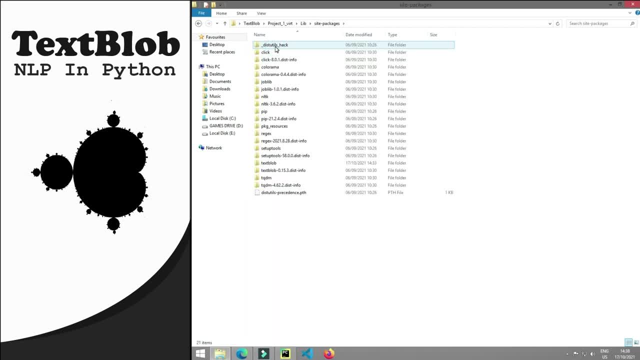 on lib then then click on this site packages, okay, and inside the site packages you will see all of the packages you have installed. okay, so i will go with the. i will go to text blob boxes or just double click on text blob and here you will find all the text. 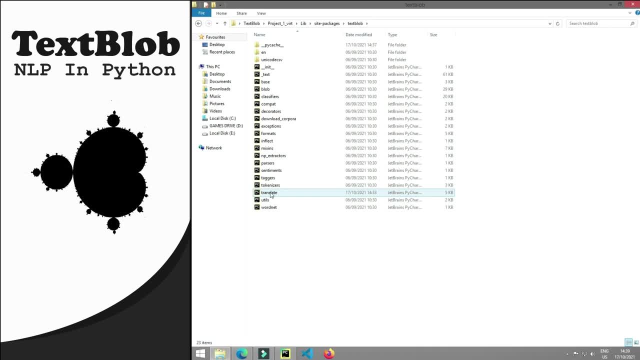 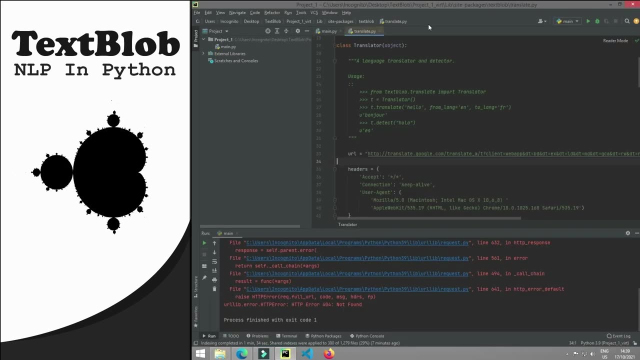 blob file. so, so my issue is with this translate dot py file. ok, so i need to make some minor changes in this translatepy file. okay, so, double click on this translatepy file and it will open the stronsleypy file in your pycharm. okay, so we need to change this url. okay, so this, basically this url. 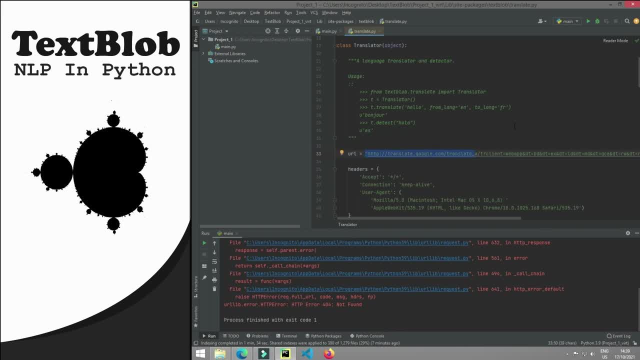 is referring to file management and let's explain the definition of this file. and if we click on text blob, okay, this translatepy file restores the file, depending on the disk itself. so my issues are state to google api, which is actually translating our stuff. okay, so you just need to put here comment. 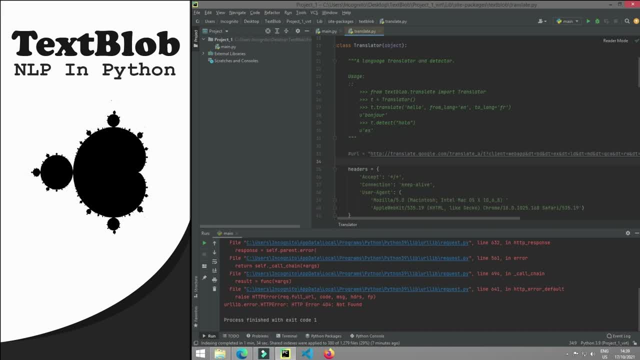 okay, come in. just right. here again url- url is equals to double quotes- and then paste the code which i will give in the description down below. okay, you can copy this code and you just need to paste it here. okay, and now. everything will work. fine. now just come to the program. okay, and now. 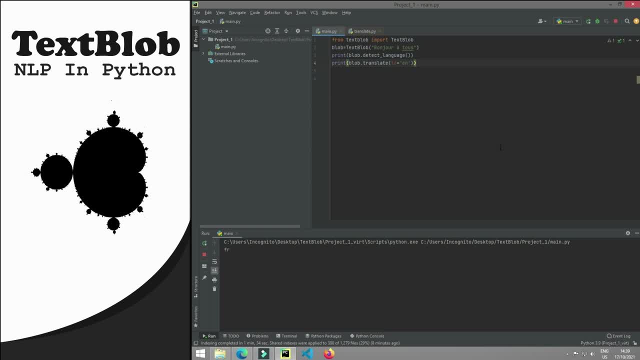 let's run it and, yeah, everything is working fine. it's french hello world, okay, everything is very good. let's run it again and, yeah, everything is working fine. so this is how you can actually solve this issue: just by making some minor changes in this translatepy file. okay, i hope that you. 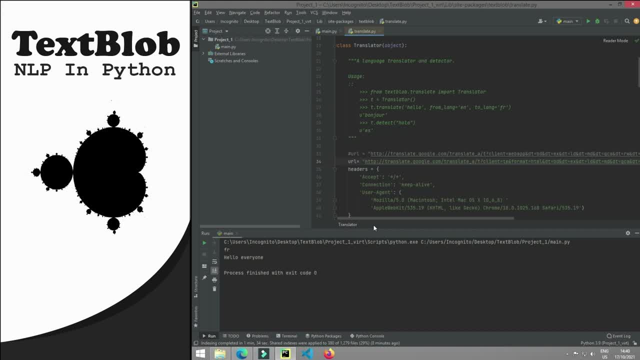 have enjoyed this tutorial and if you have some more issues regarding text blob, then feel free and subscribe to my channel and i will see you in the next video. bye, bye, and ask me and i will definitely answer your questions, okay, so bye, bye.